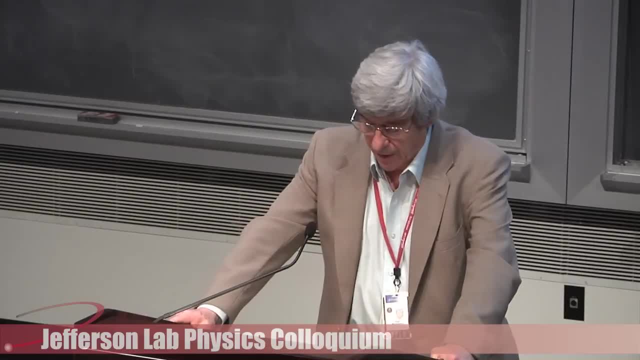 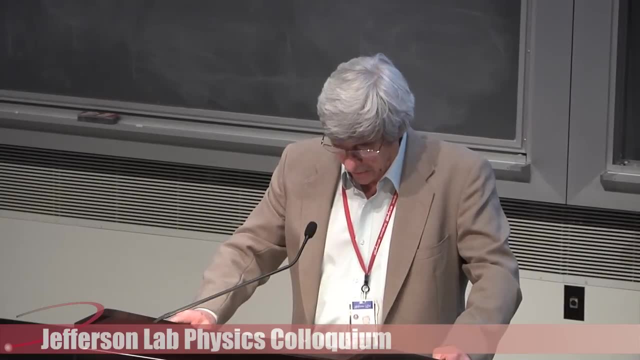 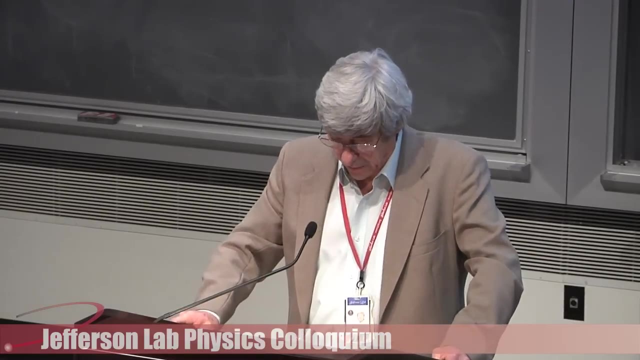 upgrade of D0. That was a device with 800,000 channels and nearly as many problems on the way to completion. But completion was achieved and in fact it ran right through to the end of the collider running at Fermilab. So some rather impressive achievements in his career. 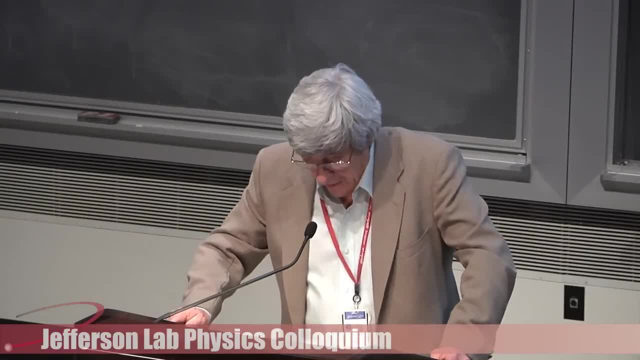 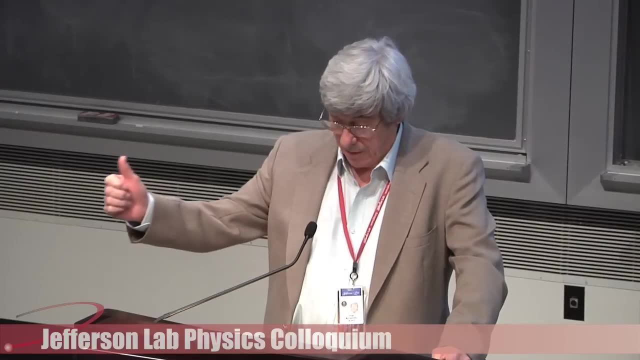 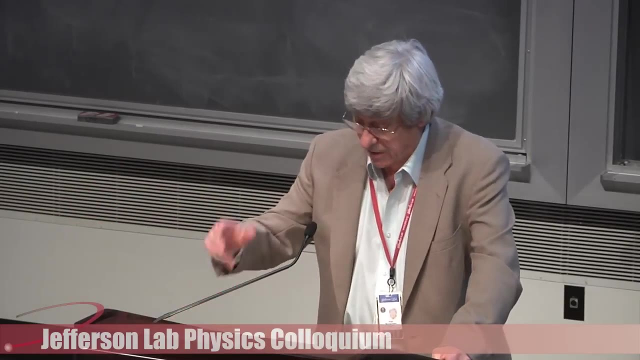 but now he's paying for it. He's a member of the BEL-2 Program Advisory Committee. He's a member of the Large Hadron Collider Committee at CERN. He, for our benefit, is a member of the Electron-Ion Collider Detector Advisory Committee at Brookhaven. And then, to complete, 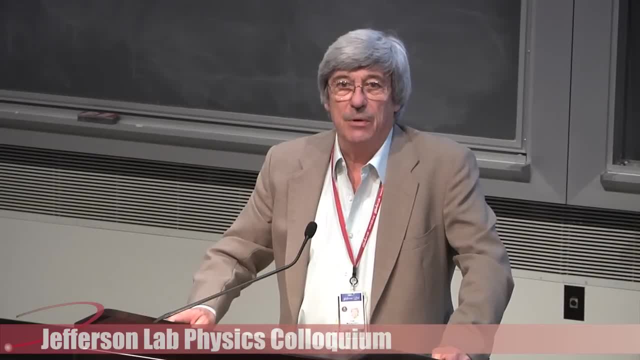 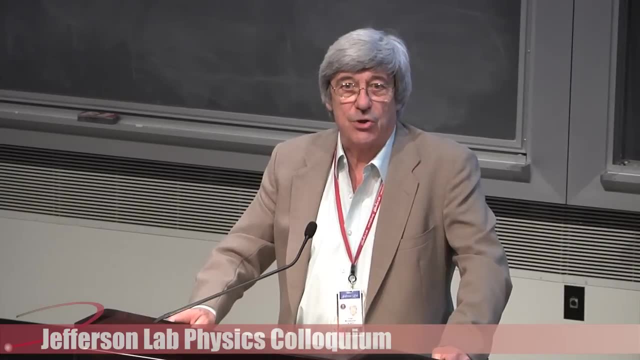 all this, he's got the pleasure of being a member of the Particle Physics Project Prioritization Panel, which he's trying to give us. He's trying to give a shape to particle physics in this country this year. So it's with great 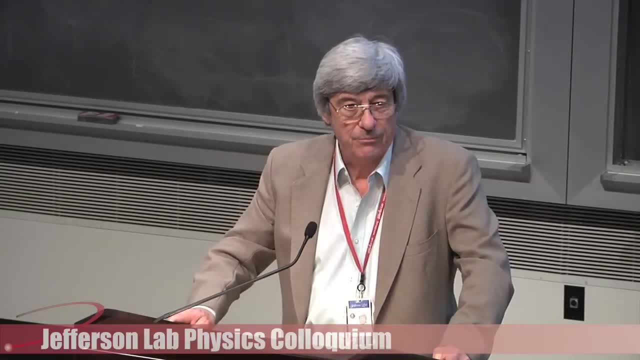 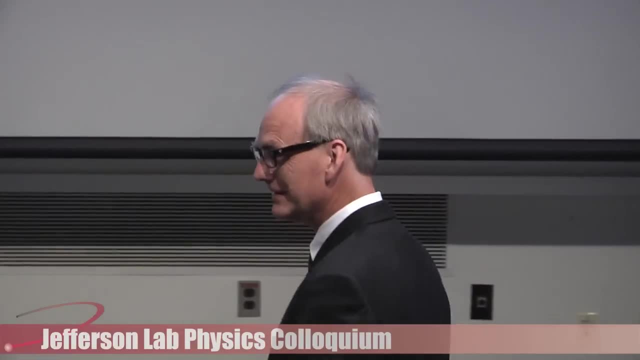 pleasure. Please join me in welcoming Marcel de Mato. Marcel de Mato, Director WMS, University of New York. All right, Well, thank you, Ron, for this nice introduction. You know I don't think that measuring the W mass is still a rite of passage for hadron collider experiments. 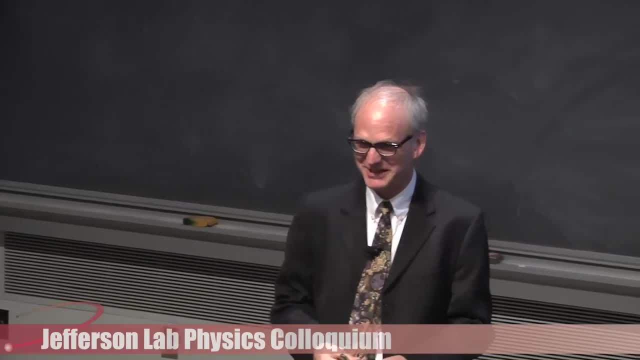 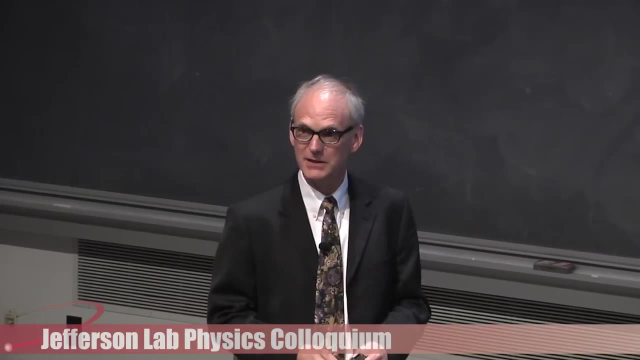 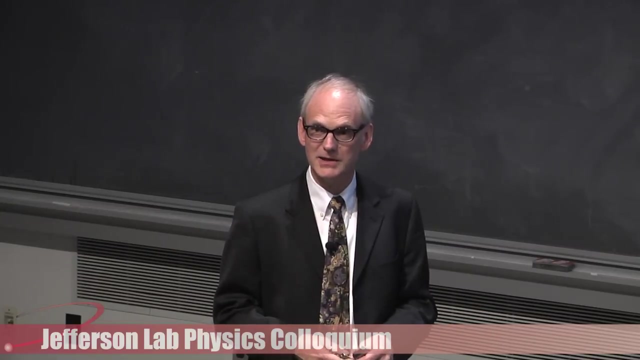 because I don't think, you know, ATLAS and CMS will be able to accomplish that measurement any time soon Anyhow. So again, thank you very much for having me here. It's a great pleasure to be here, And this talk is maybe not going to be as much physics as you may want, but maybe more. 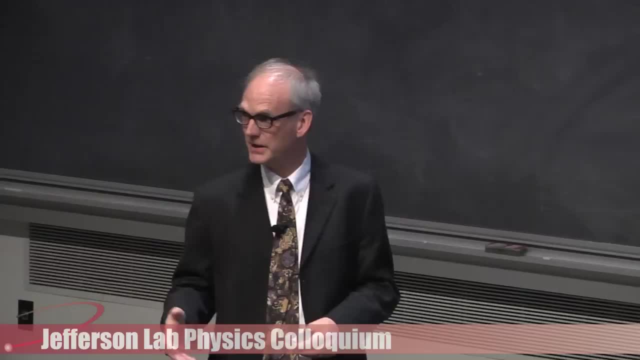 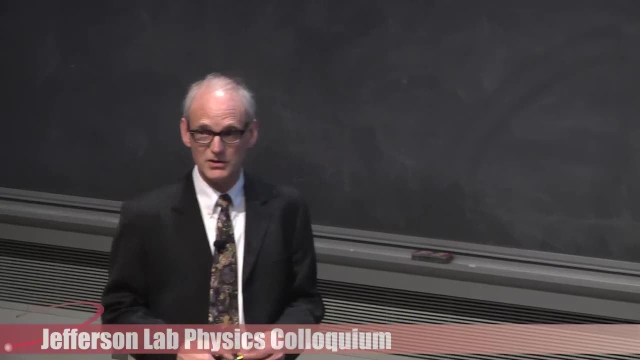 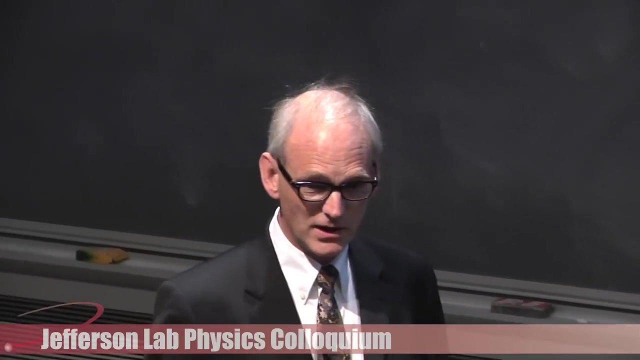 of the direction in which physics is going and, in particular, particle physics. So what I would like to talk about is the tools, the techniques and technologies of high-energy physics and the connections, And, to give you a little bit of the background, this actually came about very tangentially. 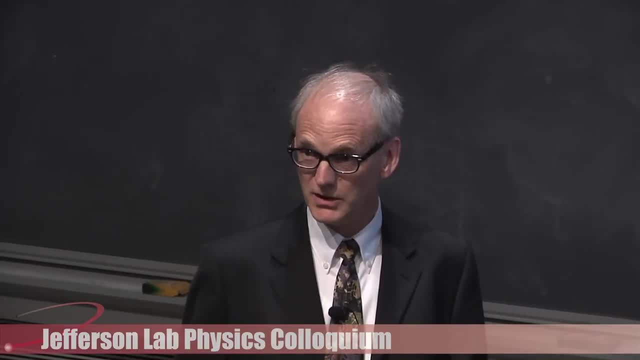 to the process that the particle physics community is going through at the moment, with its prioritization, in the sense that Jim Segrist, who is Director of the Office of High Energy Physics in the Office of Science, would like to understand better. you know what the relation is of. 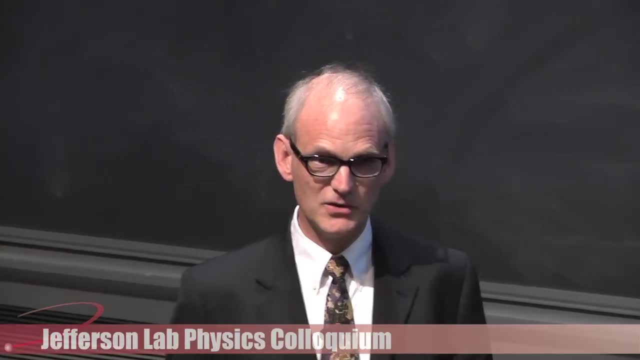 high-energy physics to other science disciplines and society. So I'm going to turn it over to you, Ron. Thank you, I'll go from there, All right. So that's what I would like to bring to this conference. The first step in general is to understand these fields of linkages and relationships. 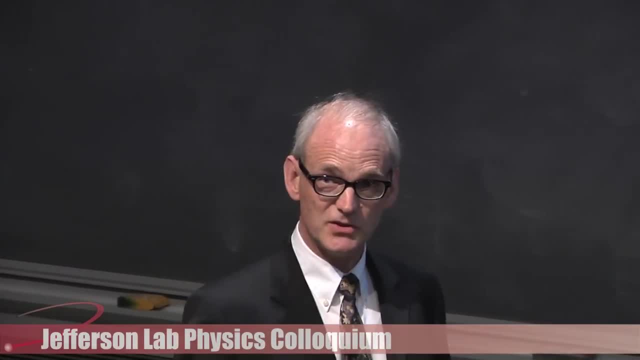 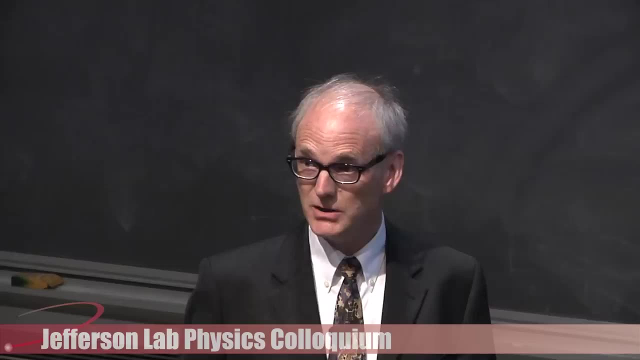 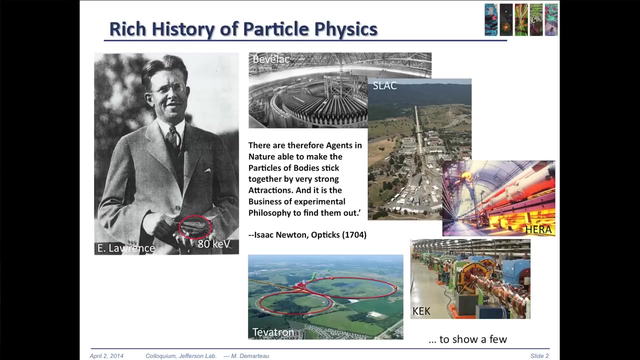 and elements and society in general, and that's how this came about. And again, so this is somewhere, you know, where it is still work in progress to understand these connections and the relationships. So if you have any feedback on that later, that would also be greatly appreciated. 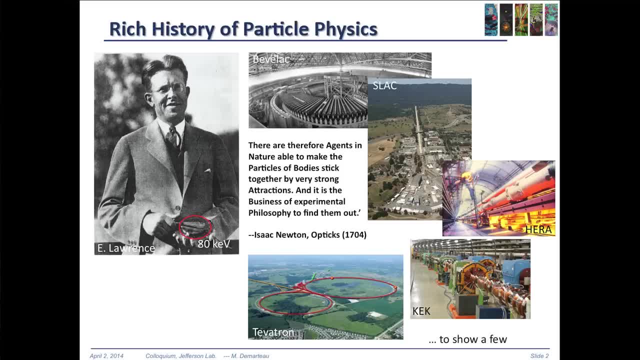 So you all know what particle physics does. You know particle physics has its humble beginnings in, you know, a handheld siendo. you know cyclotron that was developed by Ernest Lawrence and then it developed. you know these, these very massive machines that you know have accomplished. 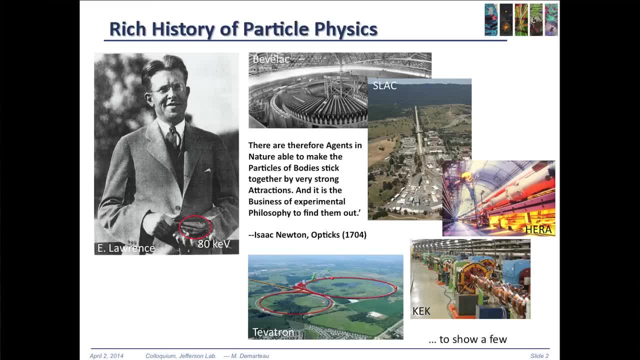 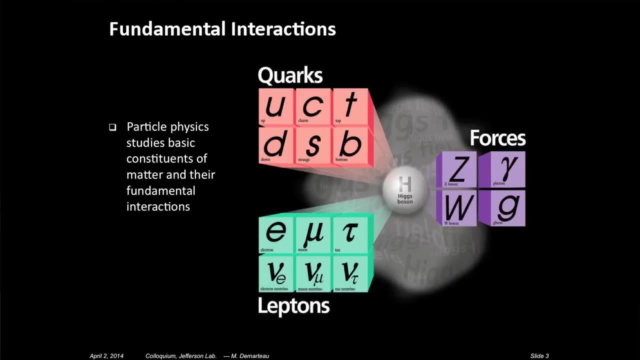 a lot. so the last machine that we had that had the energy frontier was was the Tevatron at Fermilab, which has now been superseded by the LAC at CERN. now what particle physics does, is it just studies the fundamental interactions of nature? 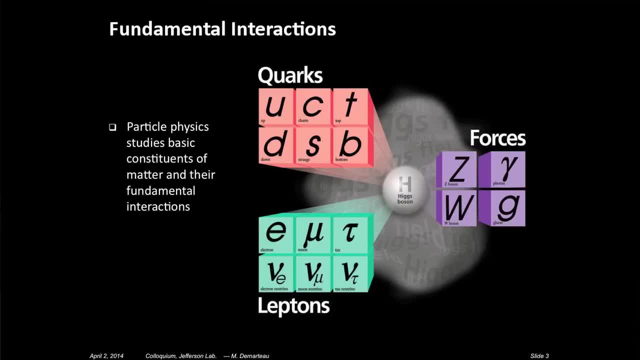 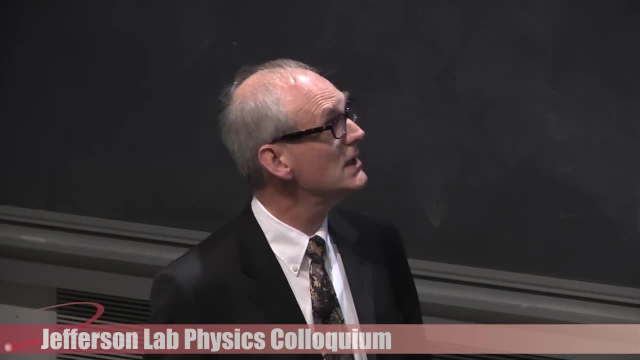 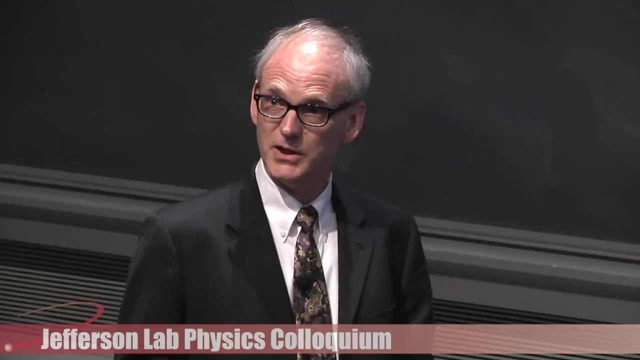 it studies the fundamental constituents of nature and their interactions, which is nicely captured in in this, in this graphic. now, the way particle physics goes at that is by by building detectors, as as anyone does, and the detectors that particle physics has built are really, I think, triumphs in instrumentation. 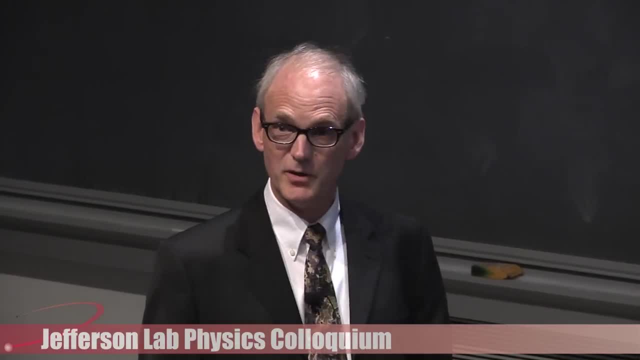 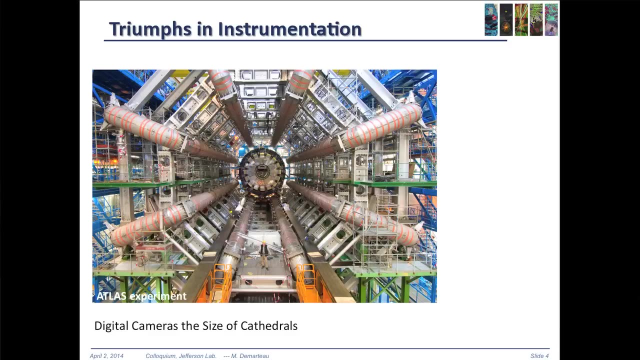 the size of these experiments and the complexity of these experiments are really unique, I think, in the field of science. so here is a picture of the Atlas experiment, just for the scale. this is a person and the other experiment is, you know, the CMS experiment and it really just captures the imagination. it. 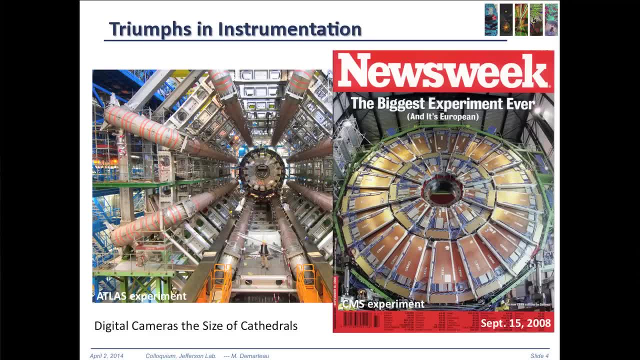 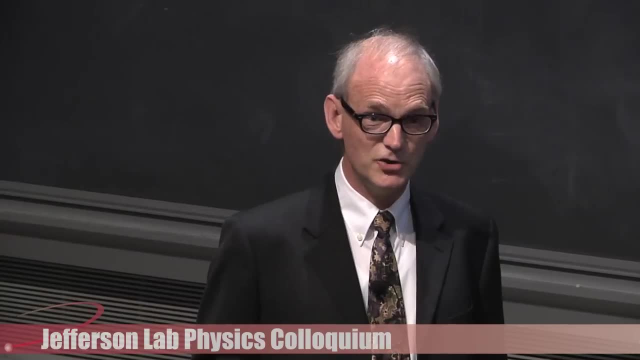 fascinates us. but it also captures the imagination of the public because it actually does make the front cover of the- you know, popular magazines like NewsSuite, You know, even though it does capture the imagination of the public. you also know, and we all know, that journalists often get it wrong. 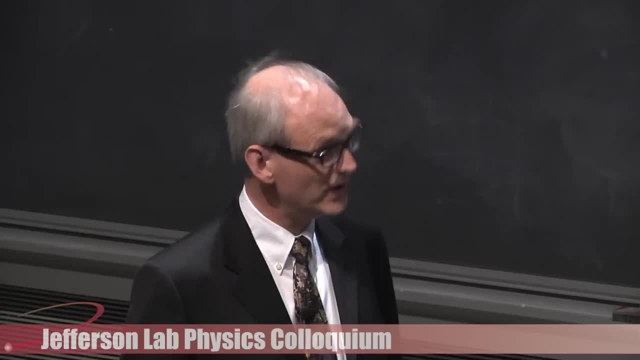 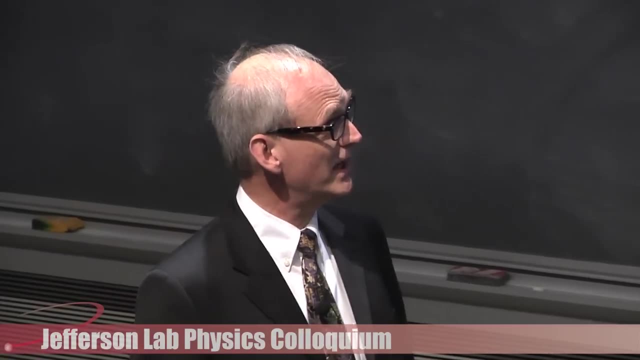 And, just as a side note, even though this is here on the cover of NewsSuite, there are two mistakes on the cover. The first one is this is the picture of CMS and it says that CMS is the biggest experiment. Actually, it's not the biggest. Atlas is the biggest. 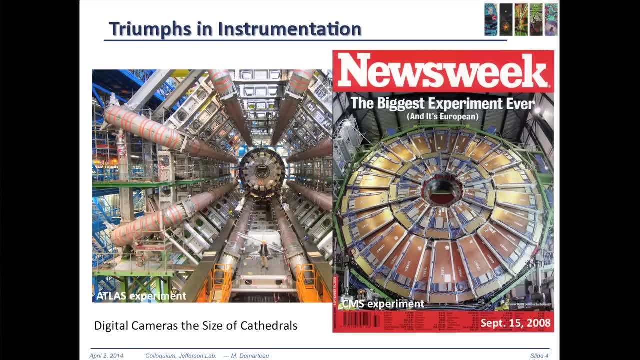 It's the heavier one of the two, but Atlas is the bigger one And the other one, which is, I think, a big mistake. it says it's European and it's not European, because the US has contributed more than 30% to both of these experiments. 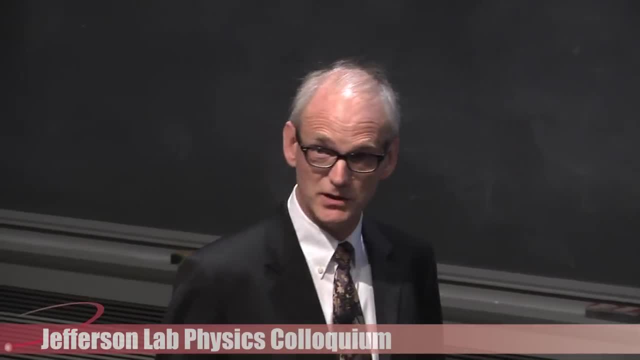 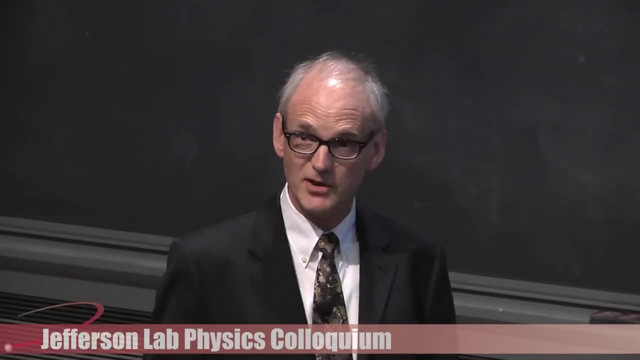 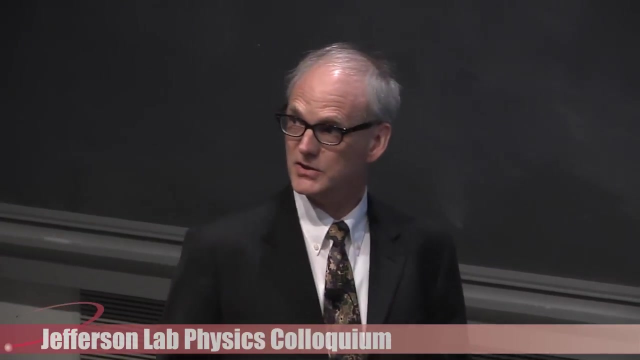 and has contributed significantly in actually the machine. But with these experiments, you know, we tried to get at the science and for the last couple of years the field has also made, I think, enormous strides in getting at the science. I mean two years ago both the ATLAS and CEGNAS experiments. 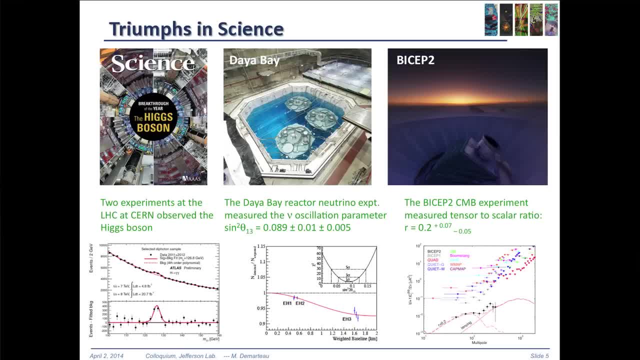 discovered the Higgs boson and this is a picture of the Higgs decaying into two gammas. Then you know, the experiment at Dia Bay in China has a reactor. neutrino experiment has measured one of the last remaining parameters in the PM&S matrix for the neutrino oscillations. 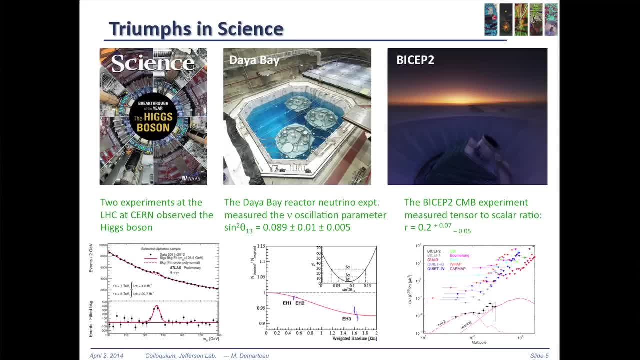 and measured the angle sine, squared theta one three and measured it to be rather small. And then, as you all read, I'm sure, is that two weeks ago the BICEP collaboration had the first evidence of actually inflation and gravitational waves. 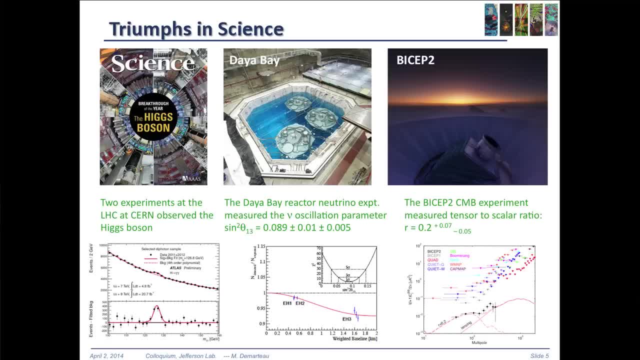 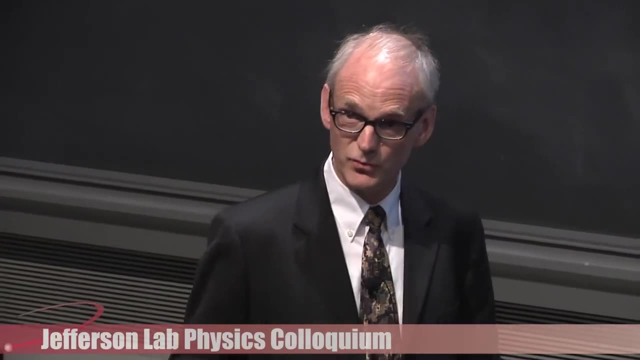 by looking at the cosmic microwave background radiation and they measured this parameter, R. So here is the power spectrum as function of angular momentum and this blip here is the indication that R, which is the ratio of the tensor to scalar ratio. so really you know the effect of gravitational waves. 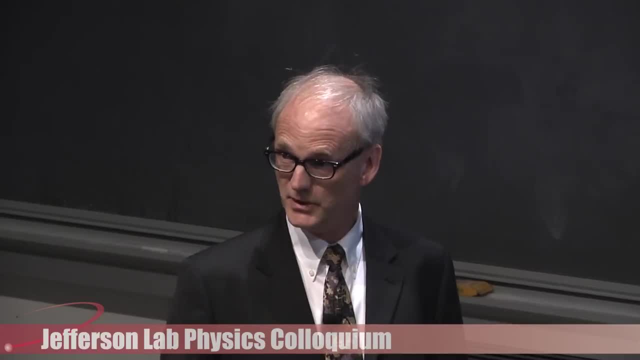 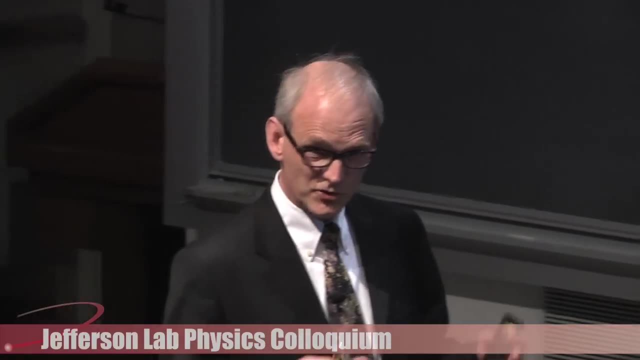 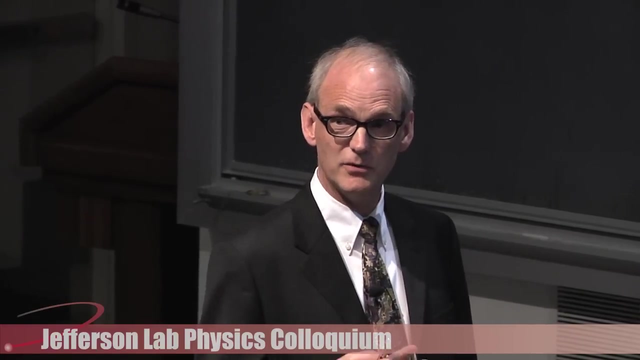 is actually much larger than people had expected. So the question then is- or you know, to just put this in perspective- particle physics, of course, has not done this alone. It has relied tremendously on other science disciplines. but at the same time, 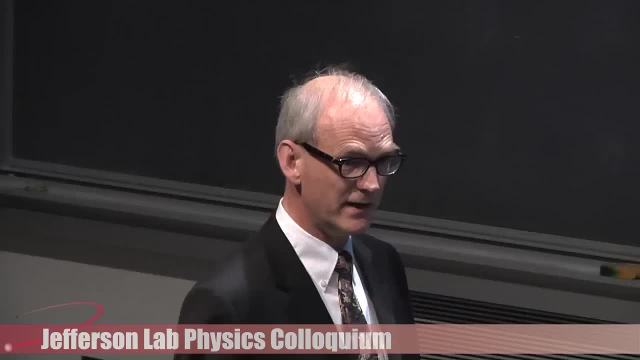 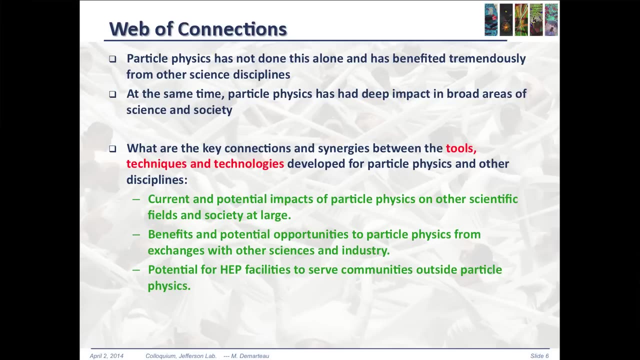 particle physics has had a broad impact for other sciences and for society as a whole. So the question is: you know, what are the key connections and the synergies between these tools, techniques and technologies developed for particle physics and other disciplines? So what I would like to do is to look at these impacts. 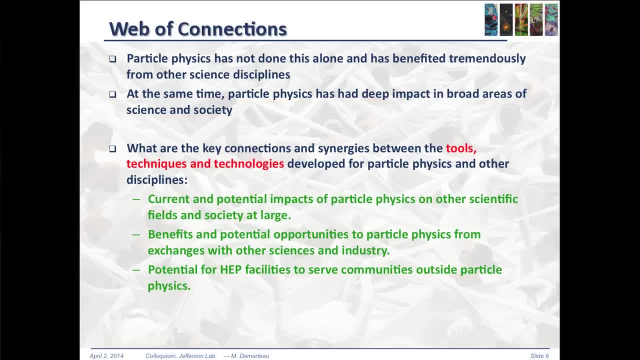 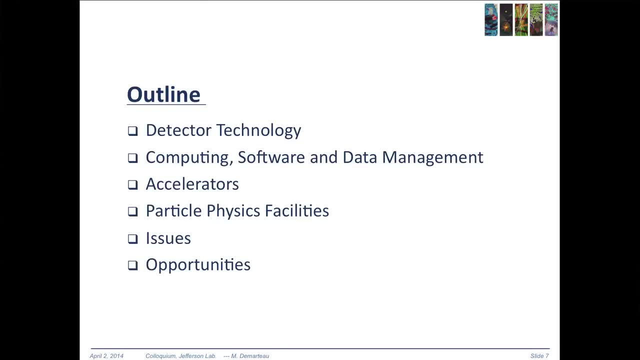 you know, and go over them one by one. So what I would like to do is first look at the detector technology, then go into computing accelerators and then facilities, and then I will conclude with what I view as some outstanding issues. 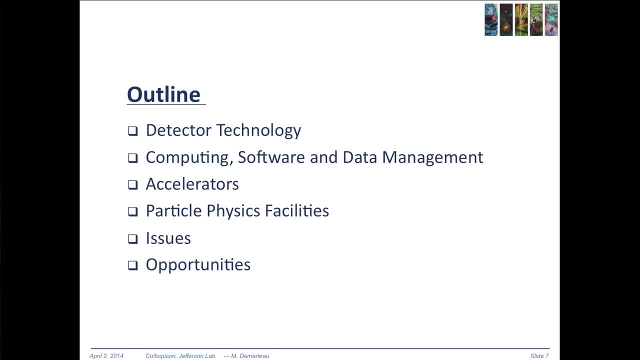 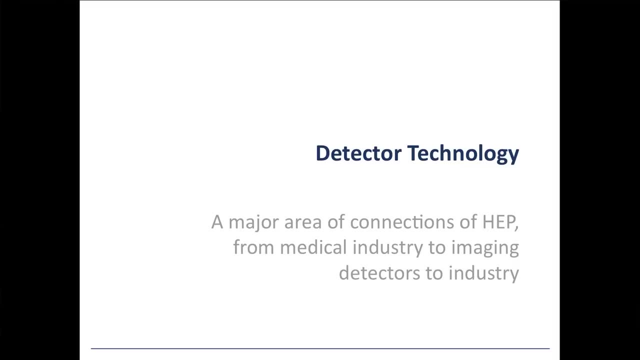 and then, especially, what the opportunities are for all of us. So first, you know detector technologies, So this is a major area of connection, of particle physics that has reached, you know, I think, all the way from medical industry to actually imaging detectors. 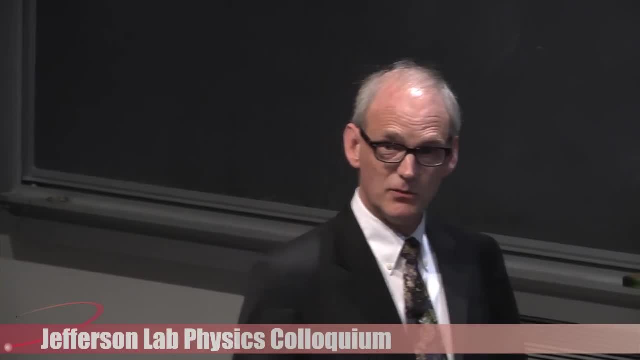 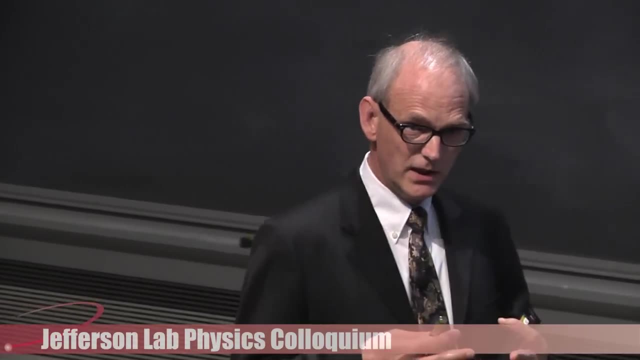 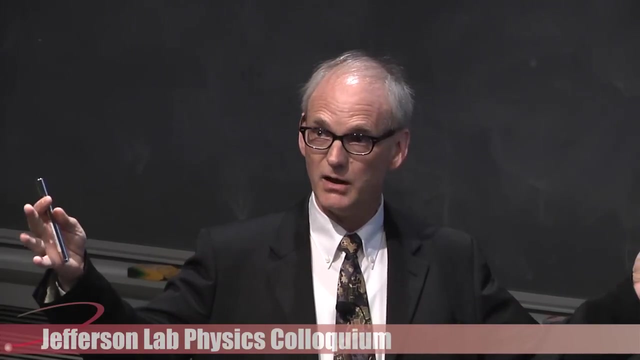 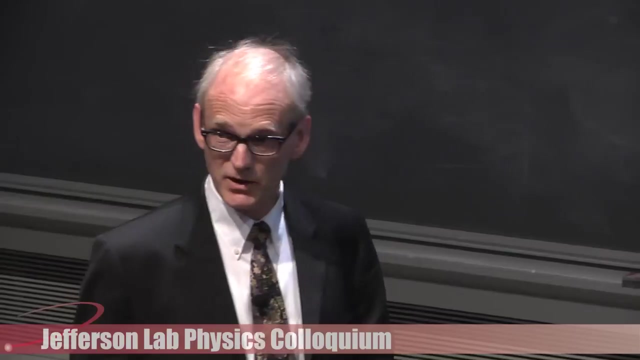 So one technology that I would like to highlight is the silicon technology. The silicon technology that high-energy physics started and brought it to such an unprecedented scale that we see now realized in these LHC experiments, actually had its beginnings in industry. It is because industry developed, you know. 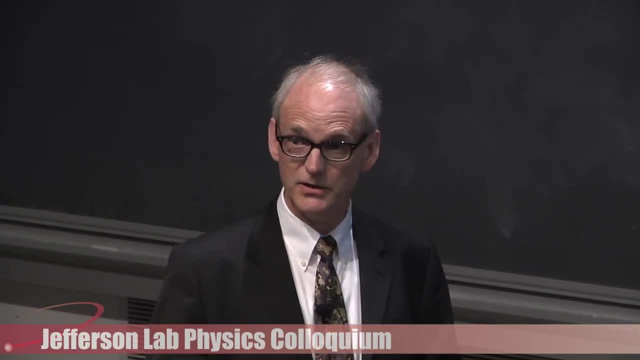 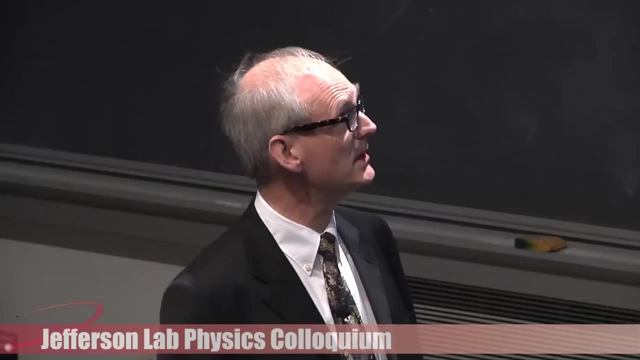 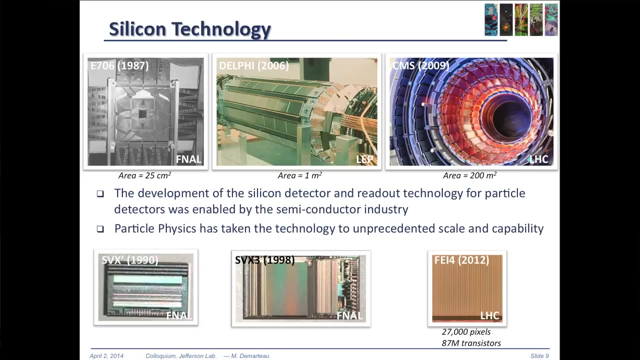 the lithography and the integrated system. The lithography and the integrated circuits. is that what you know? particle physics capitalized on and started to make these silicon detectors. So, again, it had very humble beginnings. Here's a picture of 1987 of an experiment at Fermilab. 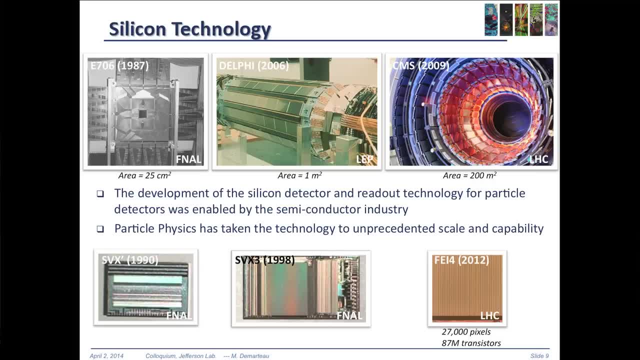 where the area of silicon here is about 25 square centimeters. That developed all the way to you know current experiments where the area of silicon is more than 200 square meters. In parallel with that, what was developed is application-specific integrated circuits. 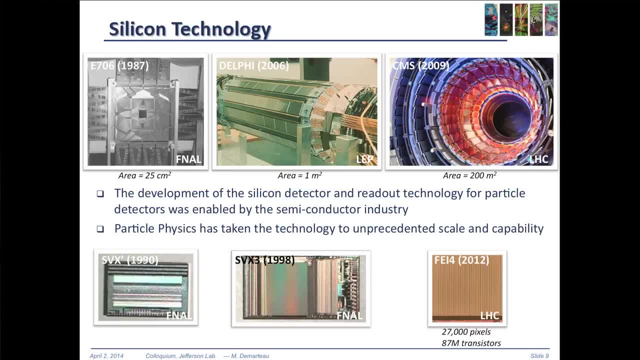 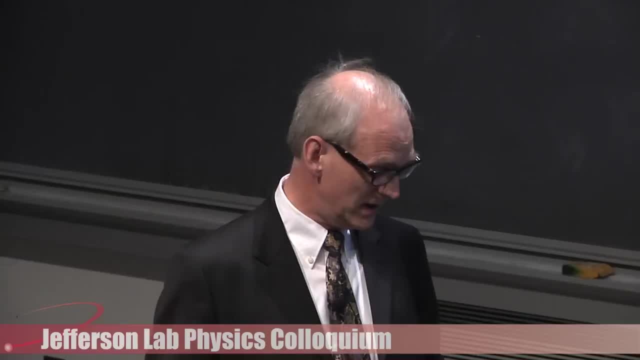 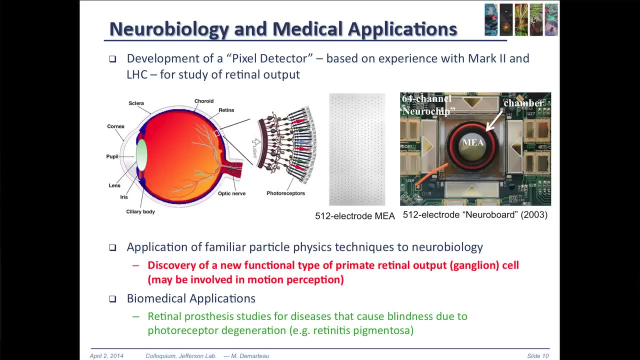 So these are integrated circuits that read out these devices. Now, believe it or not, but this technology that lies at the basis of this has been applied in neurobiology, because so it was in some sense, you know, the crossing of the path. 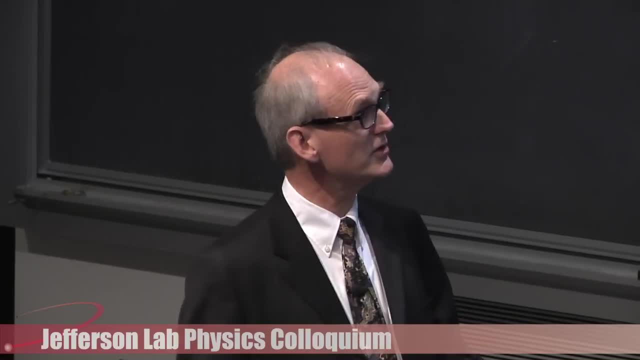 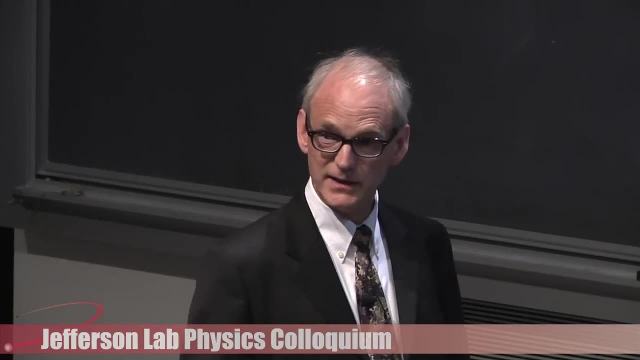 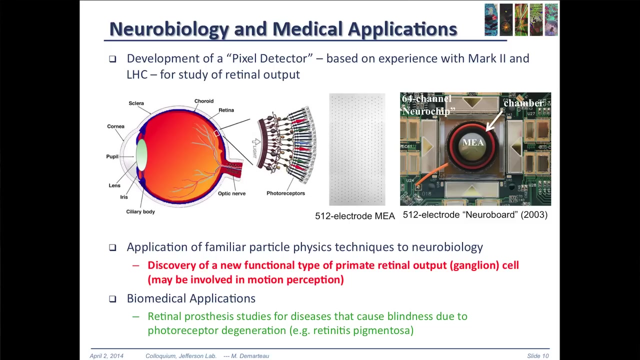 of a particle physicist and a biologist to try to understand. the problem that the biologist faced is. he said, you know, he wanted to measure the nerve pulses at the end of a retina And what they developed is exactly the same methodology that we use in silicon detectors. 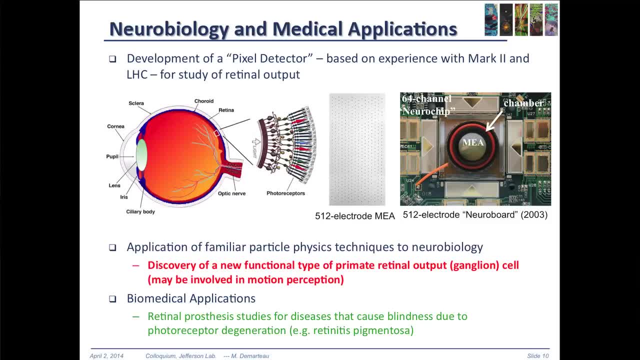 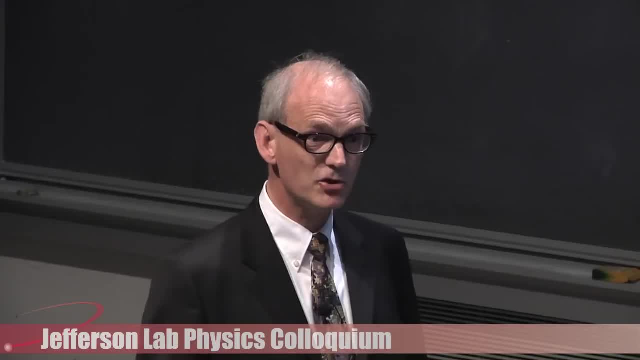 because you have, you know, a pad array of electrodes. you wire, bond it and you read it out with an application-specific integrated circuit. So you use exactly the same methodologies and the same techniques and the same readout circuitry that was developed for particle physics. 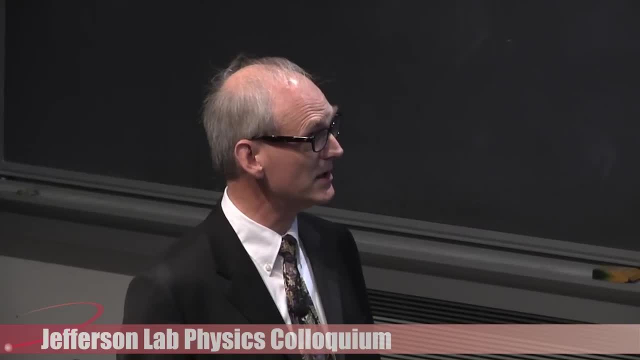 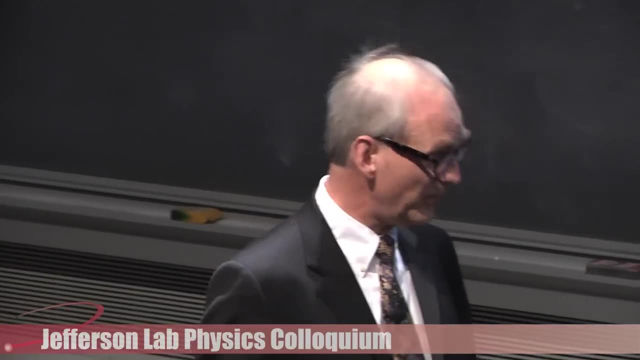 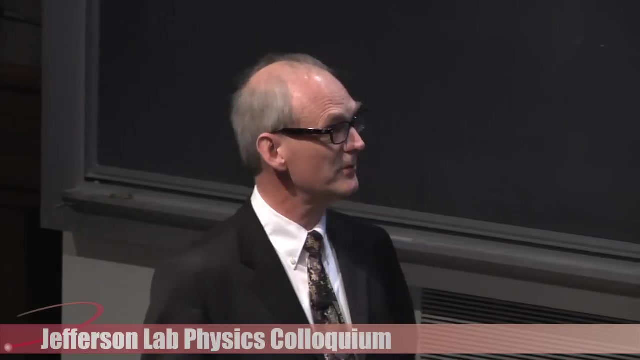 to study the eye And what they discovered? actually that there's a new functional time of the retinal output that was not known before before they did this. The other area where particle physics has had a tremendous input and still has a tremendous impact. 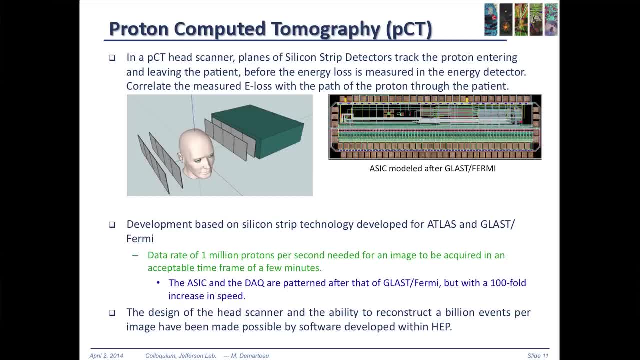 is, you know, medical imaging. So here in proton-computed tomography, what you do is- it's much better than you know tomography with gamma scattering. It's where you use protons, So you measure the direction of protons. 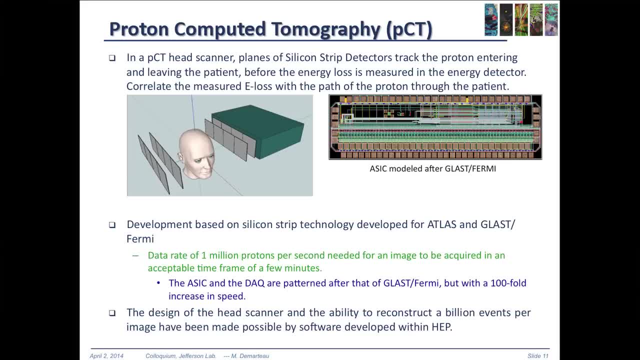 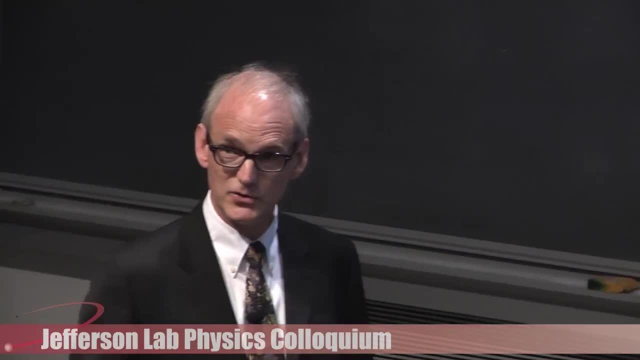 very precisely before the object, very precisely after the object. so you measure the scattering and you measure the energy laws of the proton in a calorimeter behind it. So this proton-computed tomography is being developed at the University of Santa Cruz. 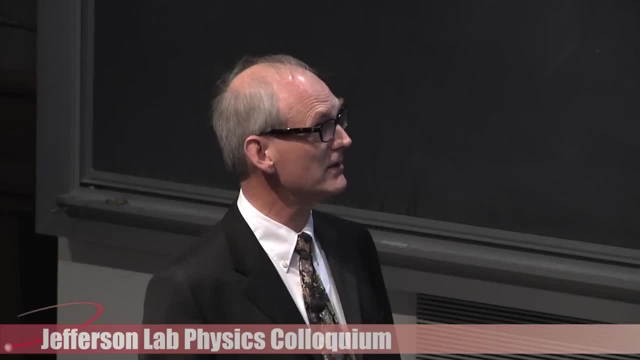 and what they use is, again, silicon detectors: silicon strip detectors to measure the projectivity of particles, and then a calorimeter to measure the energy laws, And the readout of this is exactly the same readout that was used for the GLAST-FERMI telescope. 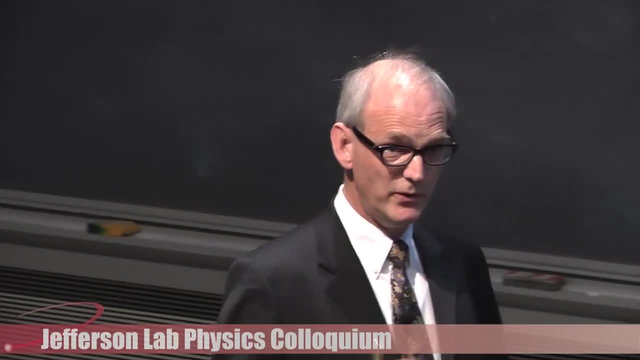 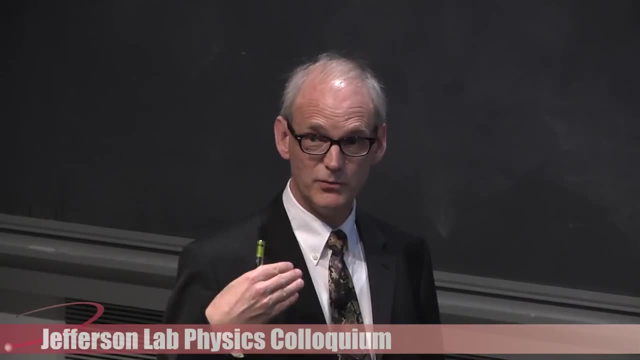 that is up in space. The main difference between this application and the application in space is that if you want to do proton-computed tomography, you have to read these out. You want to measure, you know a million protons per second. 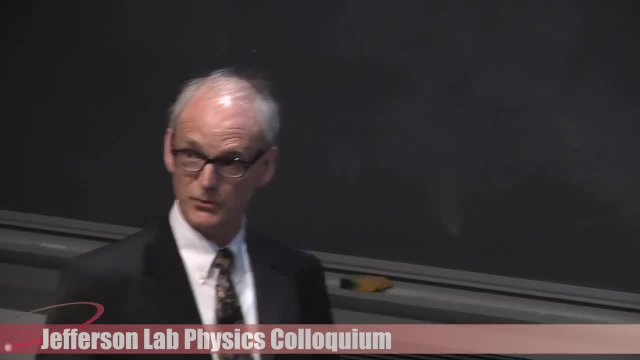 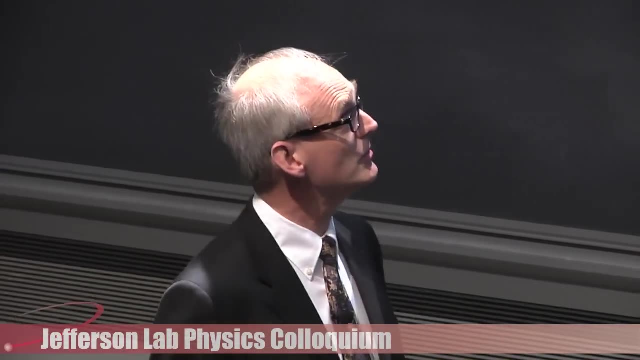 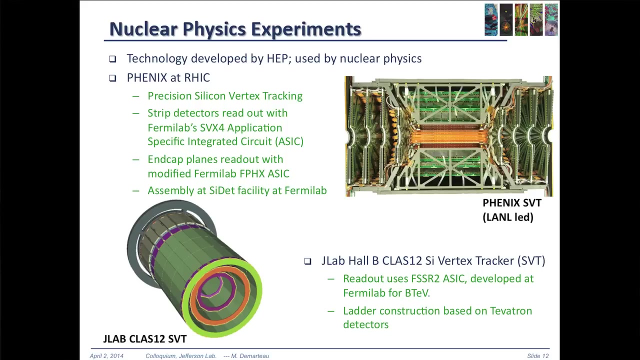 to actually be able to image, you know, a person very rapidly. Now this technology, you know, has migrated to nuclear physics, Even here at J-Lab. I mean there is the J-Lab class 12 experiment where part of the ASICs that were developed 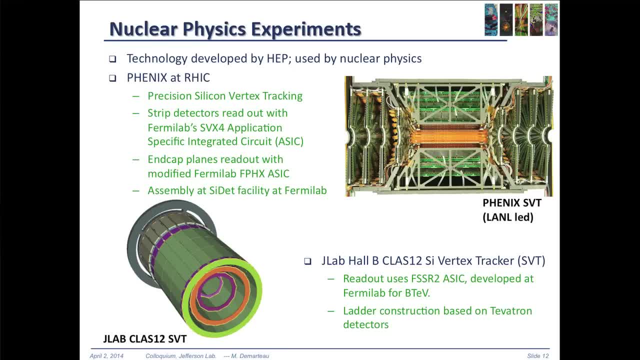 that are being used to read this out were developed at Fermilab and also at Phoenix. The SVT at Phoenix uses the readout that was developed at Fermilab for, you know, RUN-II And some of the assemblies actually occurred also at Fermilab. 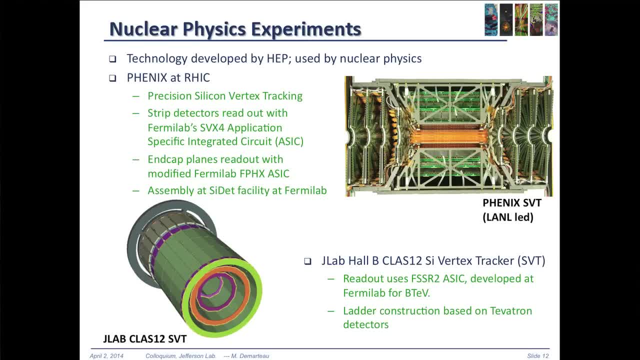 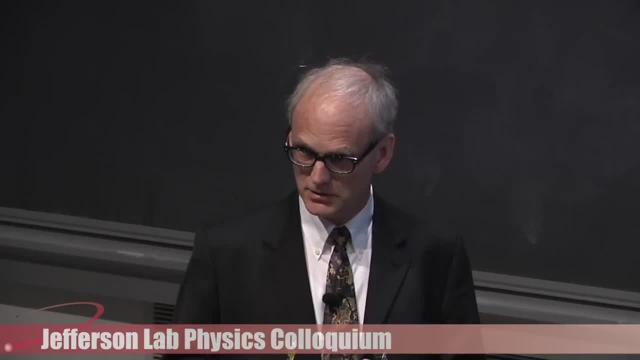 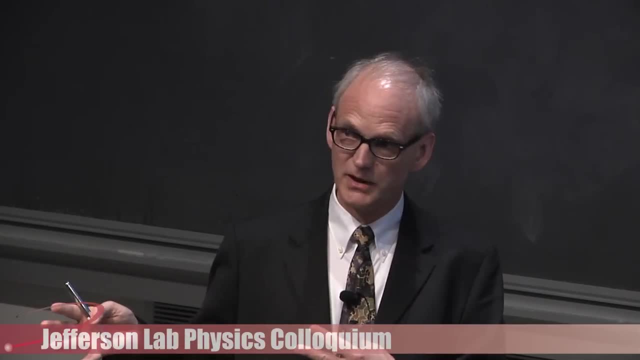 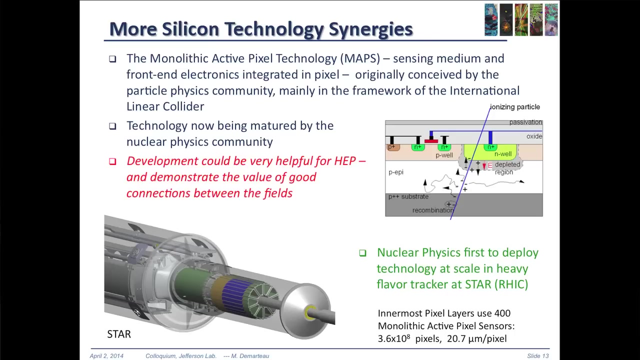 Now, one way to go beyond where we currently are, to increase the power of where we currently are, is to go in a different direction with silicon technology, and that is using what they call monolithic active pixel sensors. So in a monolithic active pixel sensor, 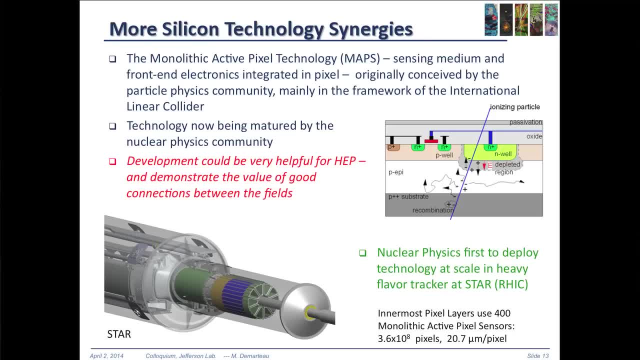 what you do is you have a sensing medium which is still silicon, but in the sensing medium right on top you also have the first stage of your front-end electronics. So you can do the process and you can put the logic and the intelligence right there. 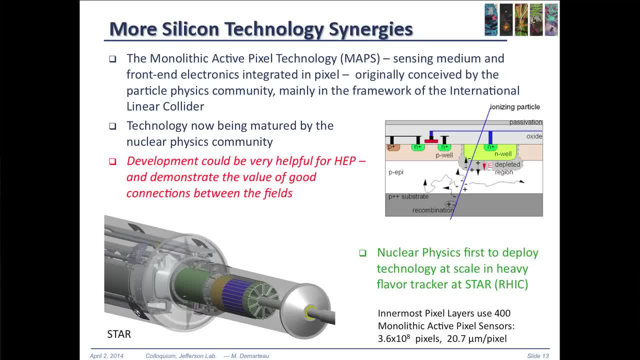 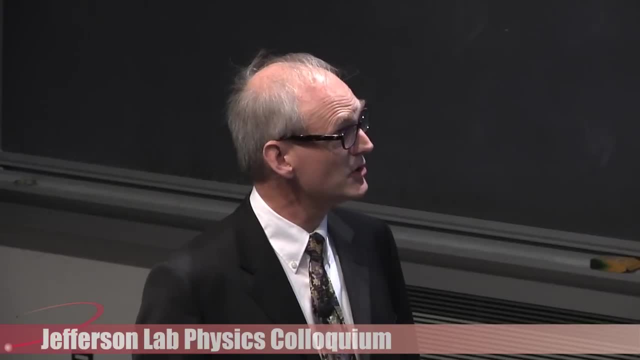 where you do the measurement. Now, this technology was conceived by the particle physics community, but at the moment it's the nuclear physics community- it's you guys- who are really running with it. So the first application of this technology is in the Star Heavy Flavor Tracker. 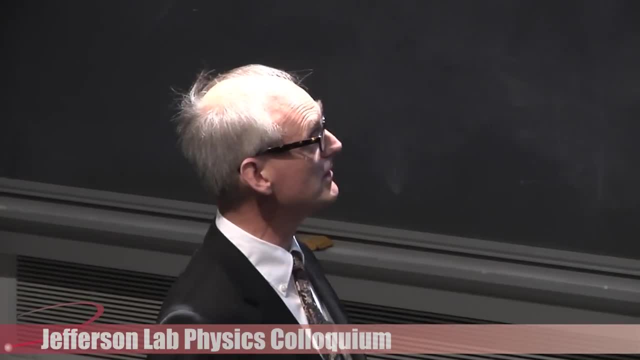 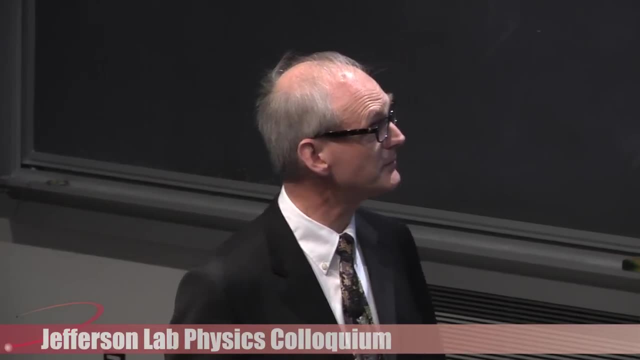 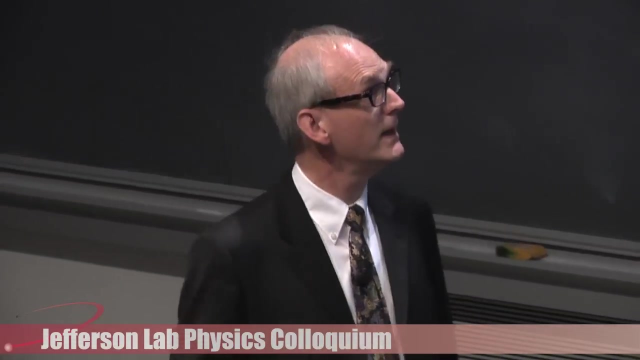 where they have a couple of layers of silicon detectors, and the further development of this technology could again really be very beneficial to particle physics. Again, to indicate you that the nuclear physics community is really pushing this technology very, very hard is here is a picture. 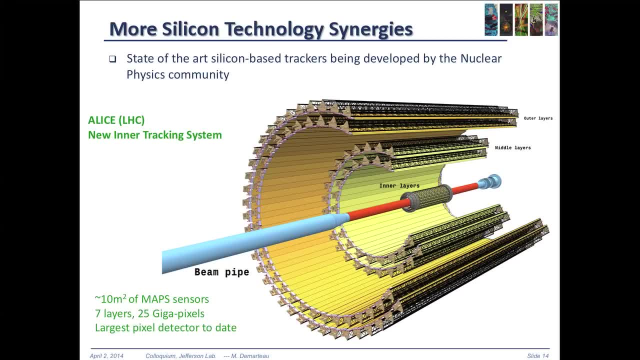 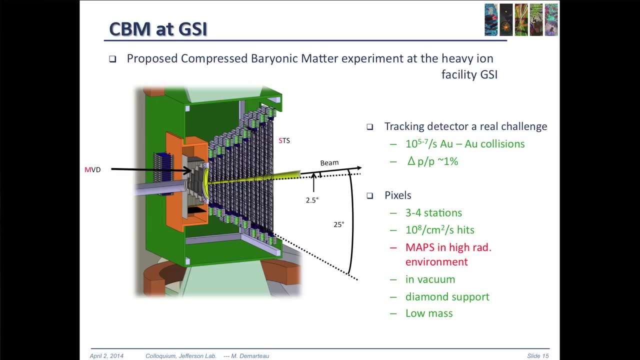 of the ALICE inner tracker system. We're just looking at the construction of a seven-layer tracker that will use 25 gigapixels. It's the largest pixel detector that has ever been built. Similarly for the experiment at GSI, where again, the first four layers- 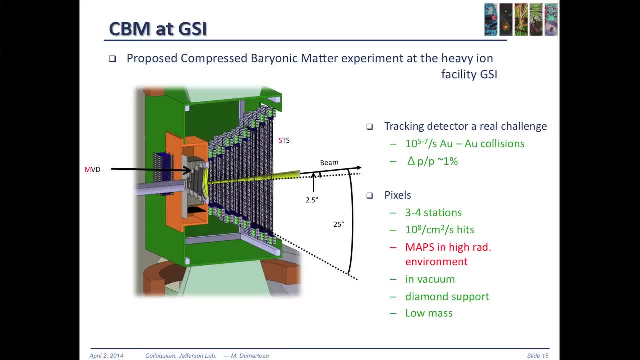 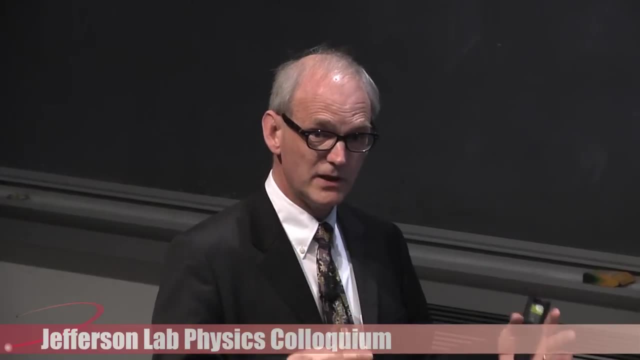 are going to be built with this technology, with the added requirement that it also has to be radiation hard, which is really something that the particle physics community will be very interested in. Now the pixel technology, the silicon pixel technology, has also spun off. 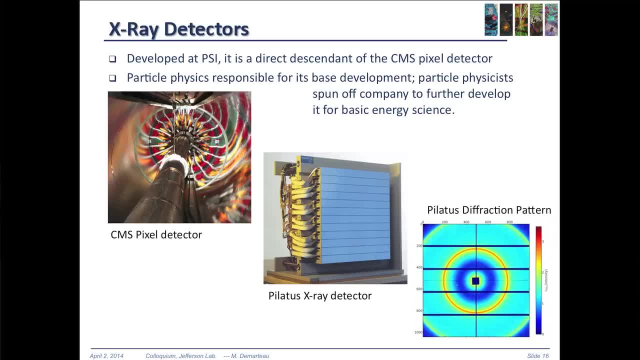 into the X-ray community. So while the CMS pixel detector was being developed- and here's a picture of the CMS pixel detector- they realized actually that you could use the same technology to also measure X-rays, And the company was spun off. 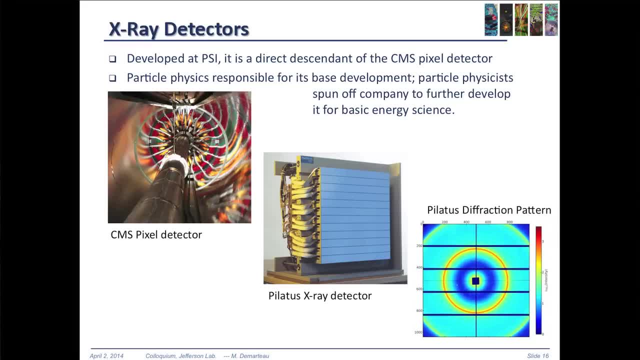 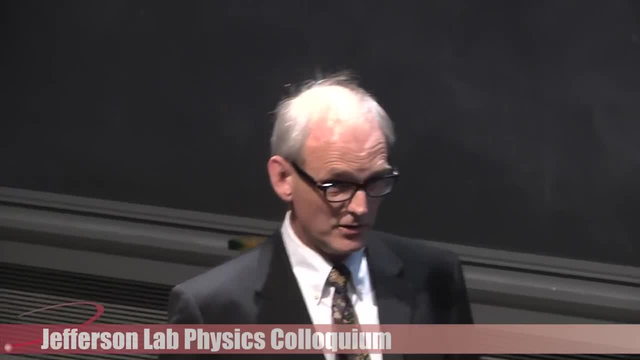 called Dectris, that has developed, you know, these X-ray detectors which are now the workhorses at almost any light source. Now, taking a look just even one step further in Europe, at the XFEL, there are a couple. 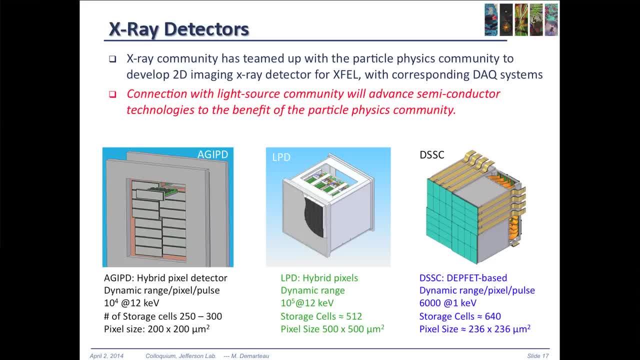 of X-ray detector projects that are being developed. The three are shown here. One is a hybrid pixel detector, The other one is a large pixel array and the other one uses another technology- DEPFA- that came out of the particle physics community. 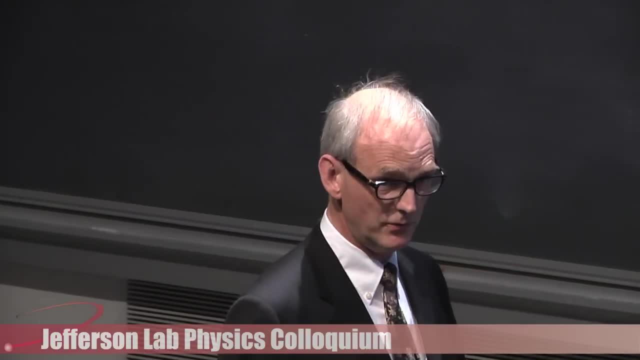 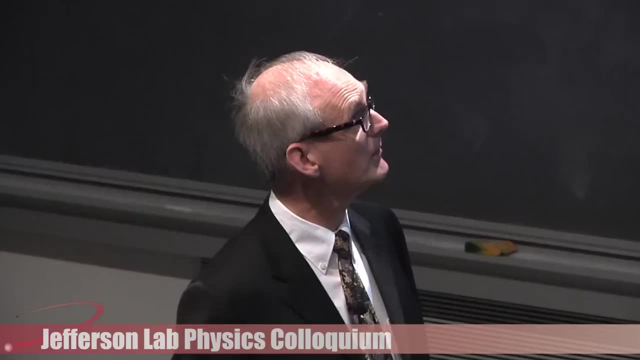 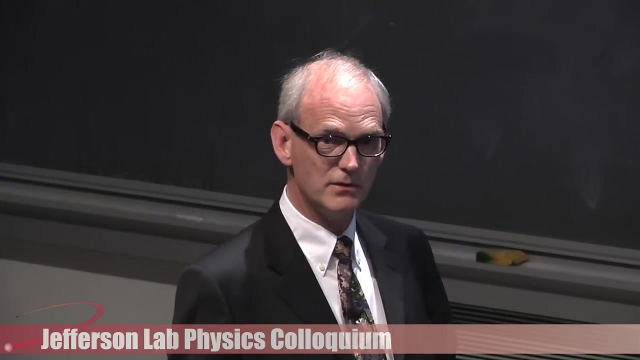 But again, these are all built as a collaboration between the particle physics community and the high-energy physics community To enable their science. Now, integral to all of this technology is the readout. So, as I mentioned already, you know application-specific. 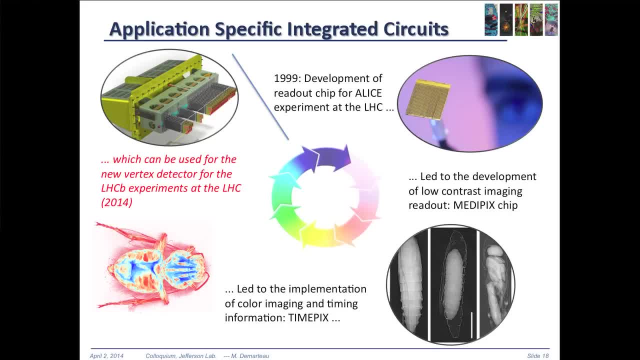 integrated circuits were fully pushed by the particle physics community And this is, I think, a rather interesting example of you know the path that these technologies have followed. So in around 1999, the particle physics or the nuclear physics community, 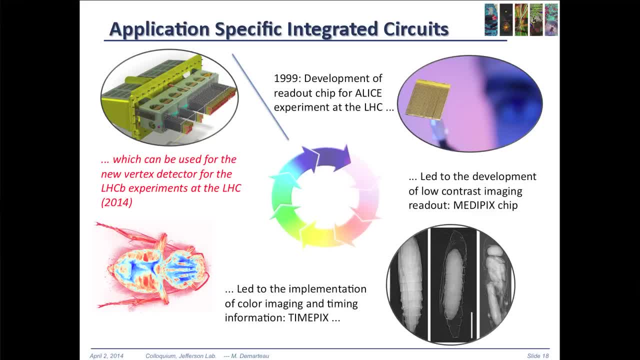 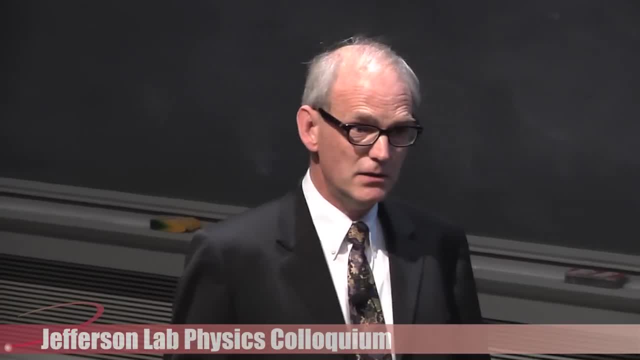 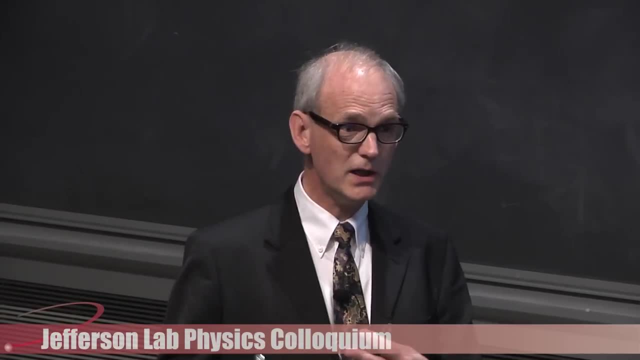 actually needed a readout for the ELISE experiment at the LHC And they developed a chip that was used for the pixel detector at ELISE. Then the project essentially stopped because there were no follow-on projects. But while working on, 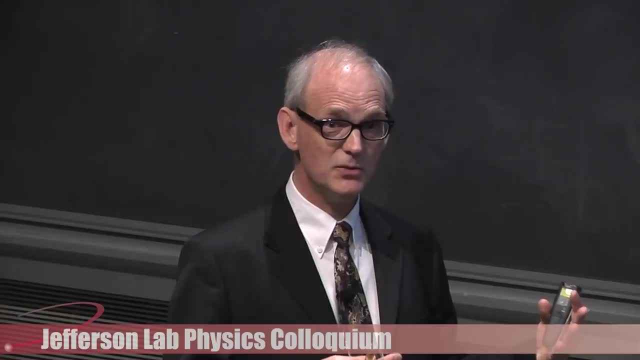 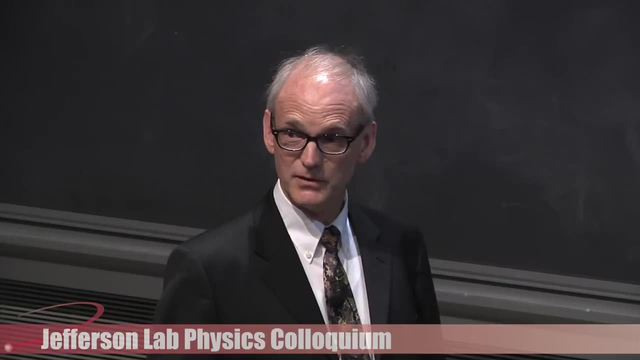 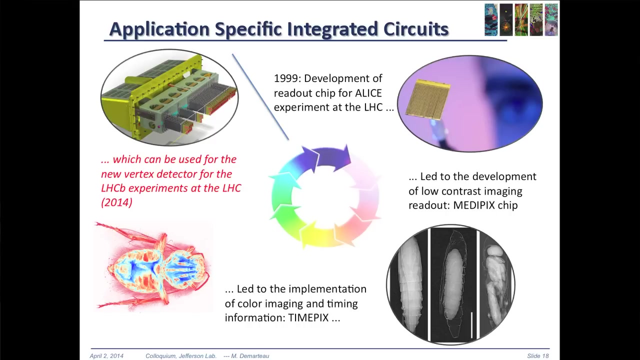 the project for ELISE, they realized that this was a damn good chip to also use for X-rays. So out of this came the development of the MediPix and the TimePix development that is now being used to make you know these X-ray images. 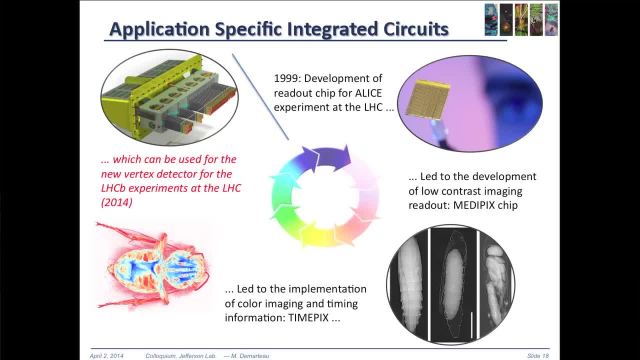 Now it turns out that in these 10 years of development- and they really have pushed this development- now they have a chip- the TimePix 3, that is used for the LHC, which almost meets all specifications for the upgrade of the LHCb detector. 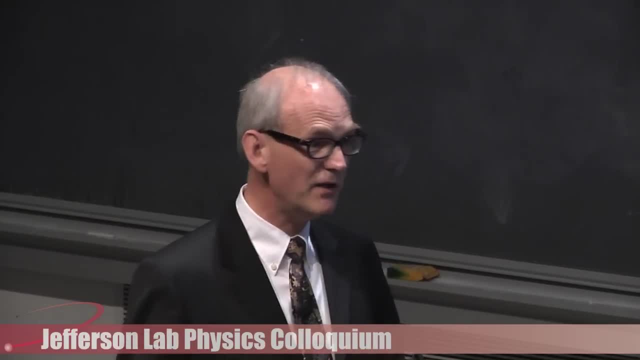 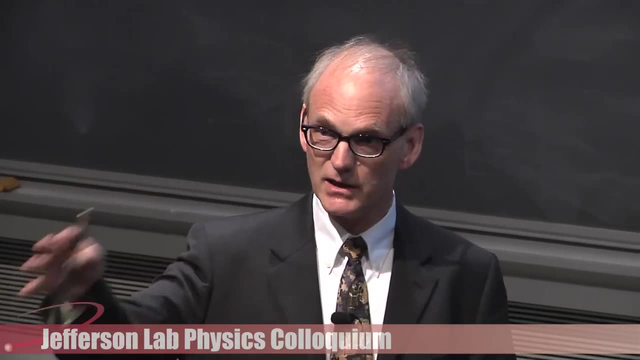 So it is not. it was the way I view this is, you know, enlightened management that let this project go on and maybe have a little detour from its path has fully paid back. you know the investment that was made. 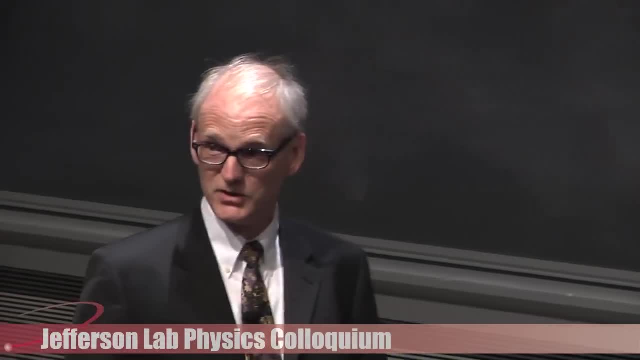 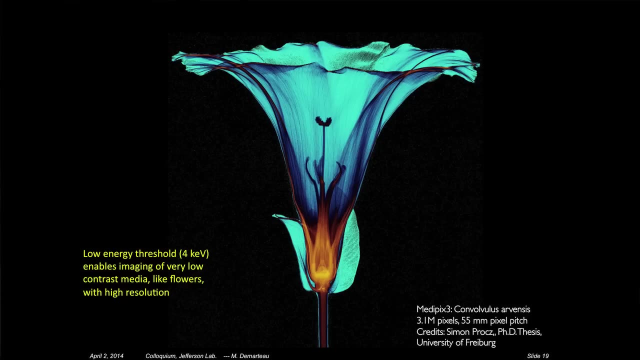 And to show you here a picture. this is a picture that was taken by the TimePix, the MediPix 3 chip, you know, which shows the contrast that you achieve with this device And this. these are 4 KEV. 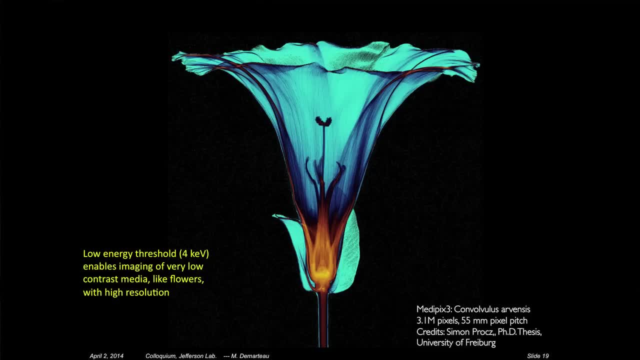 you know gammas and the only way you can get this if you really have single photon efficiency and very, very low noise readout. If you compare this to the X-ray you get from your dentist, you know the difference is striking. 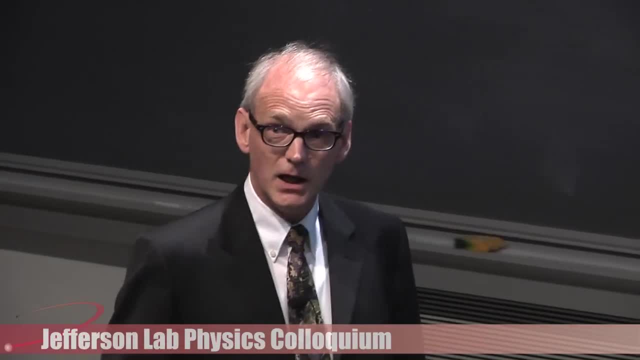 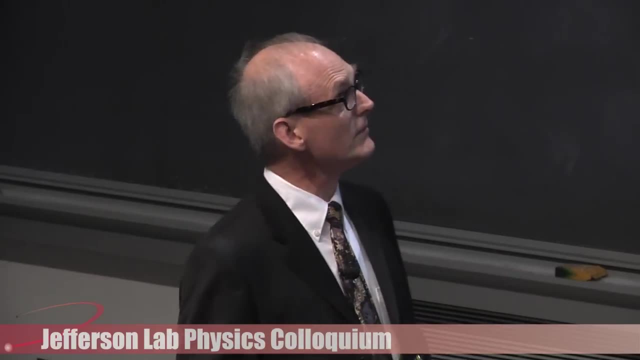 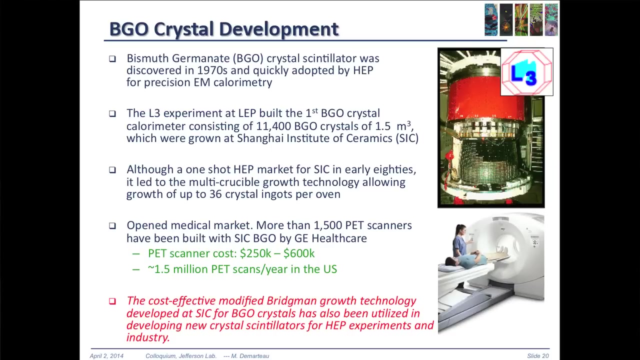 I find It's striking. Let me just change track here a little bit. And that is crystal development. So you know, we knew that BGO, which is this crystal bismuth germanium oxide, existed in the 70s. 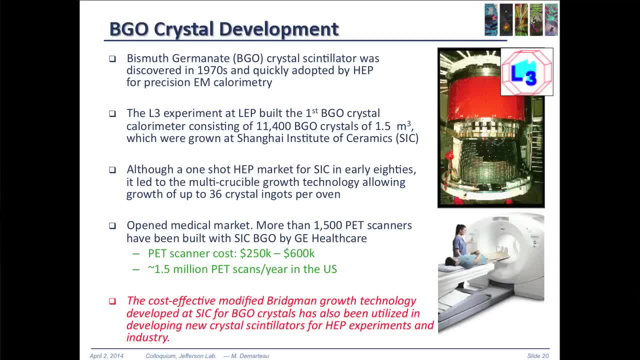 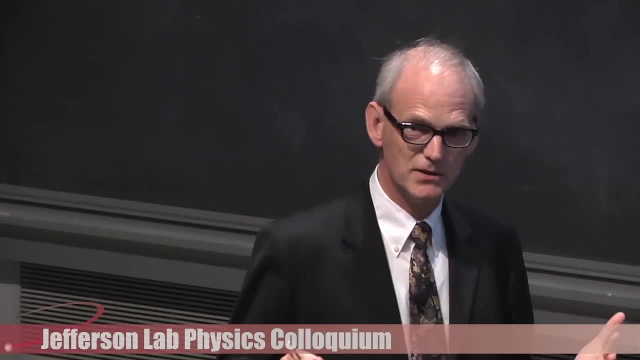 But the L3 experiment at LEP, at CERN, decided to actually at one point build an electromagnetic calorimeter using these crystals because it had the best energy resolution, And this is again something that is unique to particle physics, and that is the scale. 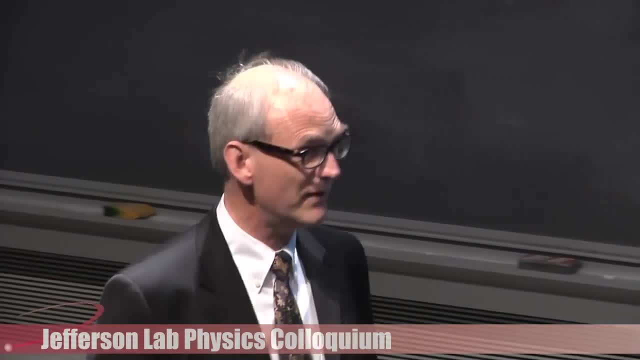 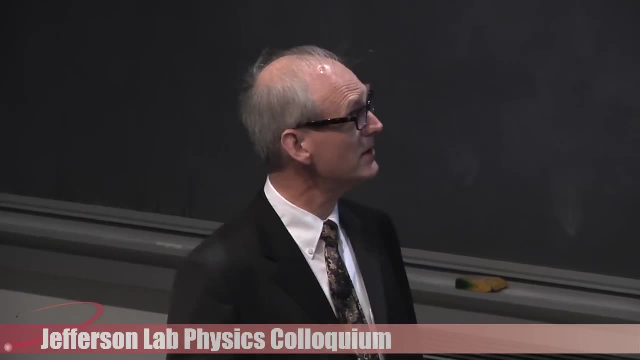 of these, of these devices. So L3 needed about 11,000 of these crystals and at the time that they wanted it, they could only grow a crystal one at a time, But they contacted, you know this- Shanghai Institute of Ceramics. 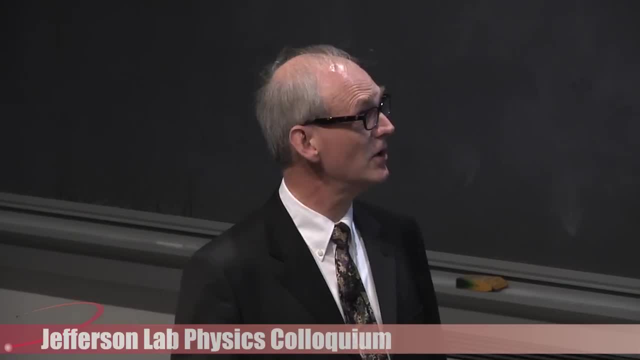 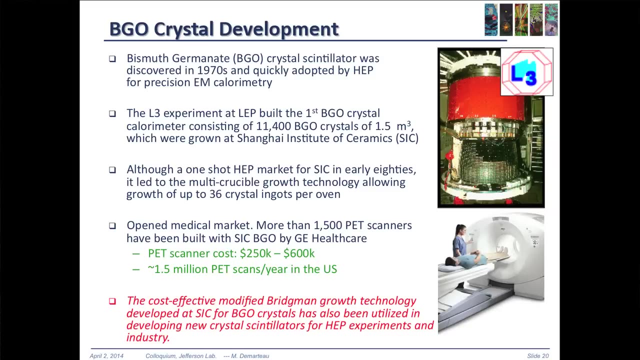 and they developed, in conjunction with this company, a method where they could build 36 crystals in one shot, And that simply was the breakthrough: to make this technology available to the medical imaging industry, because then it suddenly became cost effective, So this opened the medical market. 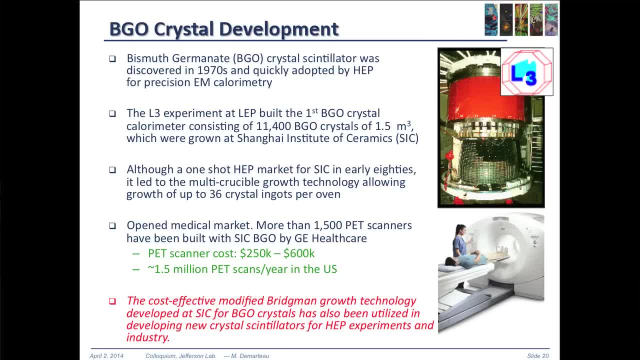 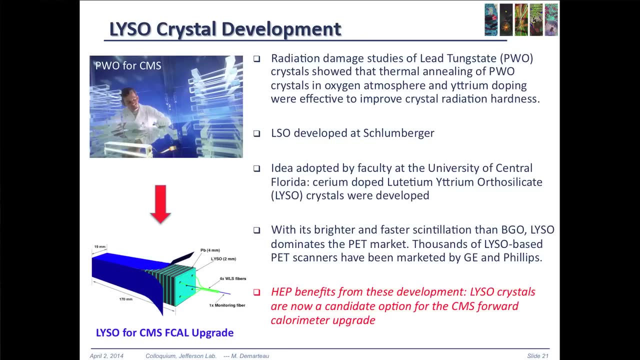 and 1,500 PET scanners have been built by GE Healthcare, you know, using crystals used built by this, this method, by the Shanghai Institute of Technology. Now, another example is the development of, of lysocrystals. So, during the 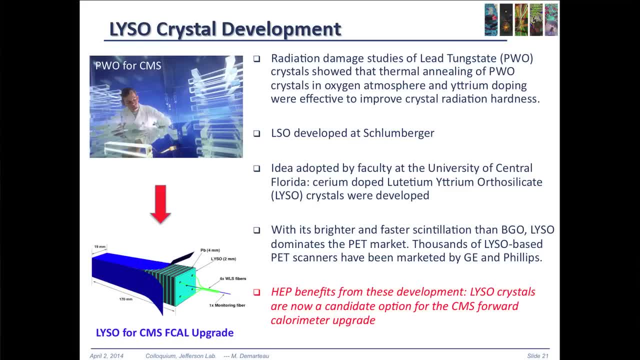 the last phase of of the LHC, when CMS was building its electromagnetic calorimeter, they decided to use lead tungstate. One requirement for the LHC experiments is always that everything has to be radiation hard. So when they were looking at the radiation hardness, 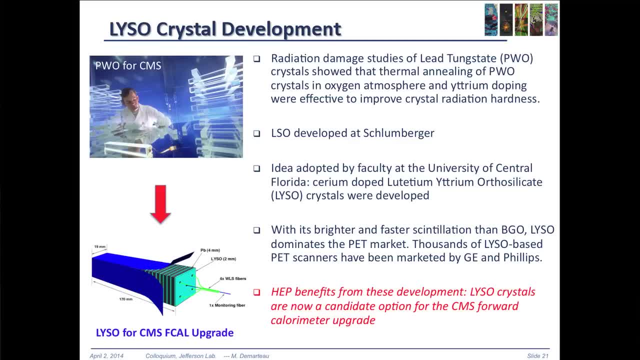 of lead tungstate. what they discovered was that the LHC is a way to make lead tungstate radiation hard, That is, through special annealing and yttrium doping. Now, at that time, LSO was already discovered by H Schlumberger, but somebody 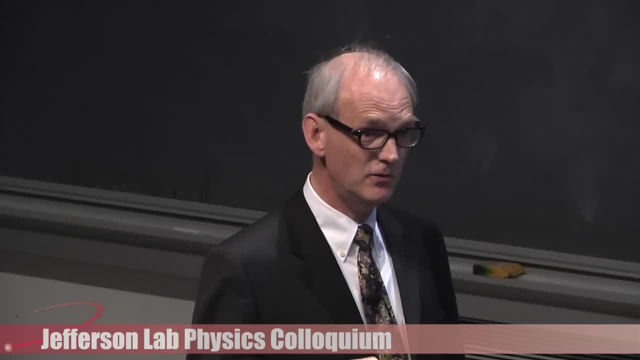 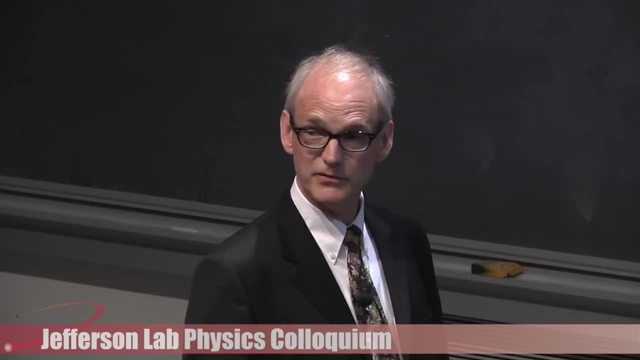 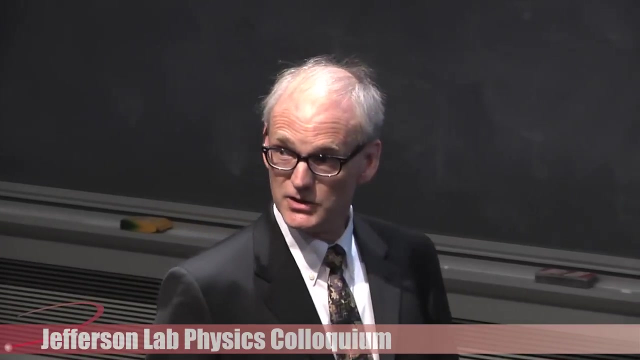 put these two together. So somebody- and he gives the particle physics community full credit for that- He says: you know that because of the yttrium doping he, you know, invented LISO. So that is the crystal that is now being used. 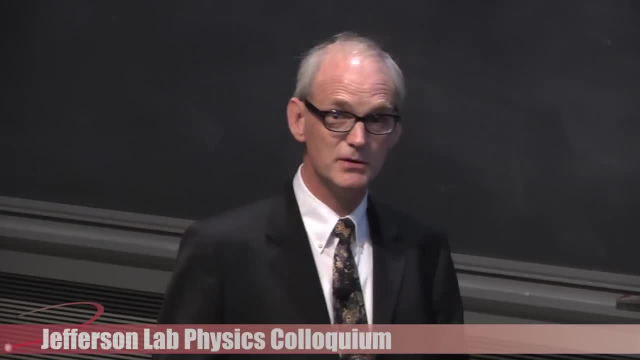 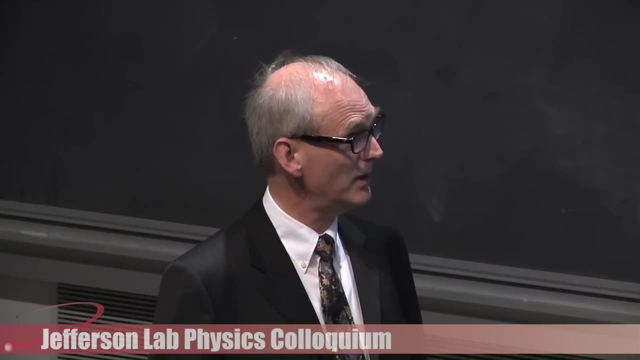 most within PET scanners in the medical industry. So here again, and now you know. in turn, the particle physics community can use these crystals for their next generation of experiments, because the MUTV experiment at Fermilab would like to use LISO crystals for their calorimeter. 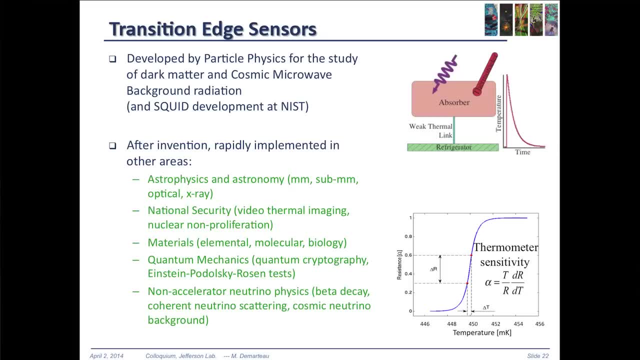 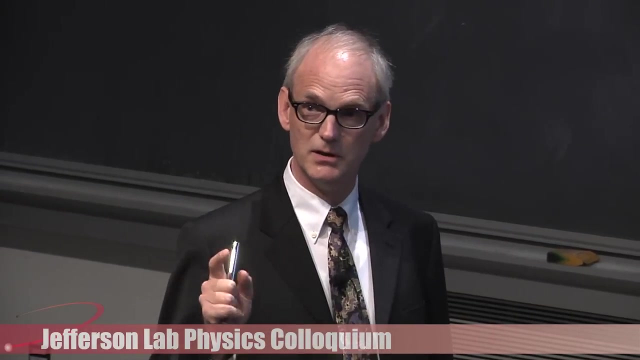 Now this one I put in because it is the basis of the result from two weeks to look at gravitational waves, because these gravitational waves have been detected with transition edge sensors. Transition edge sensors have been fully developed by the particle physics community. There's just no doubt. 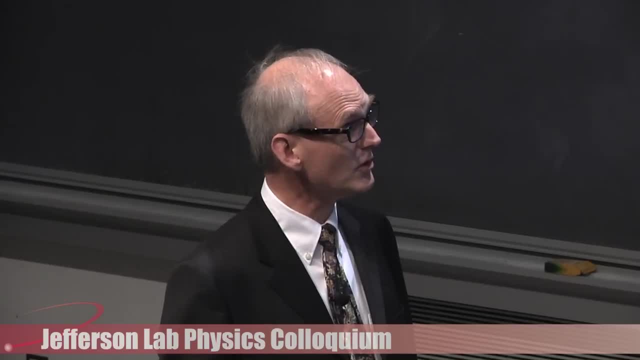 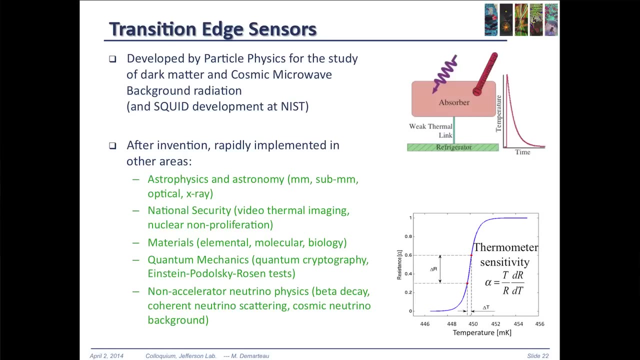 about it, And what is really interesting about this experiment is that there are two types of materials that are used to measure the temperature of this absorber. So what you do is you engineer this superconducting material to be right at the center of the 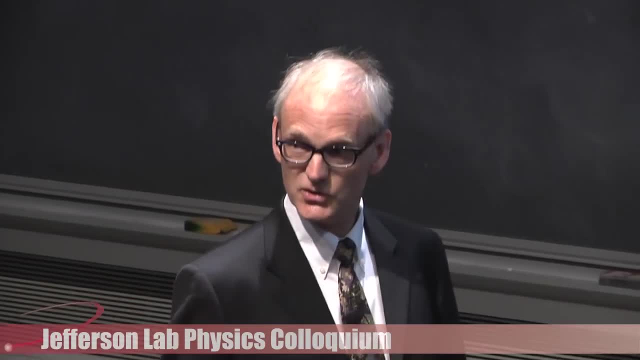 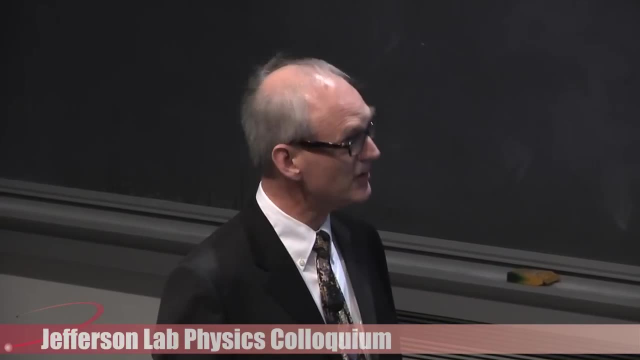 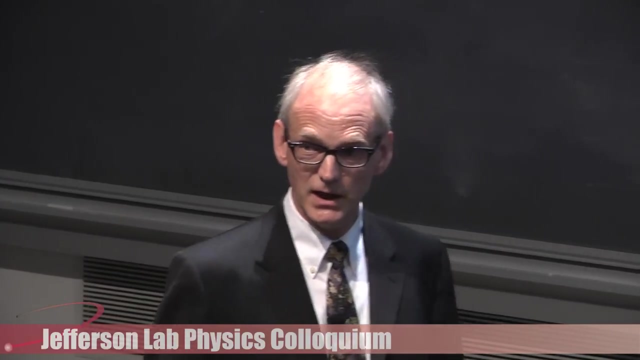 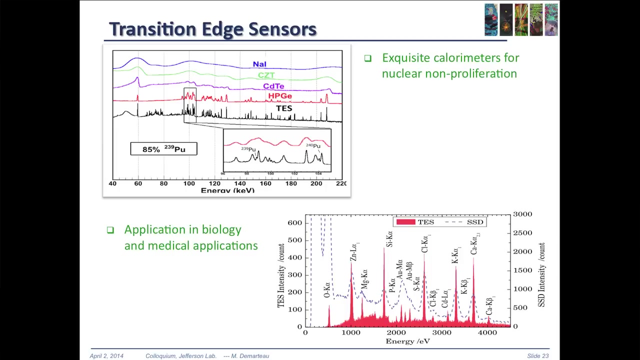 absorber. So what you do is you measure the temperature of this absorber, And what you do is you measure the temperature of this absorber, And what you do is you measure with sodium iodide all the way up to a transition head sensor. 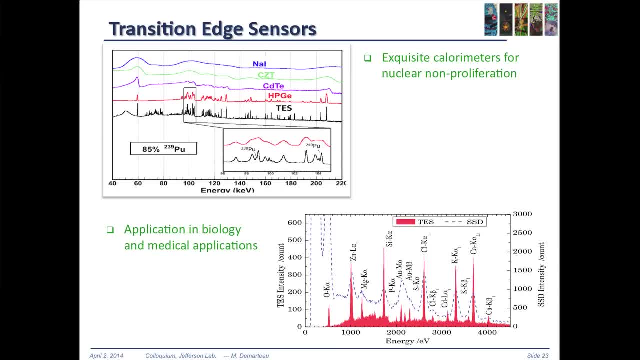 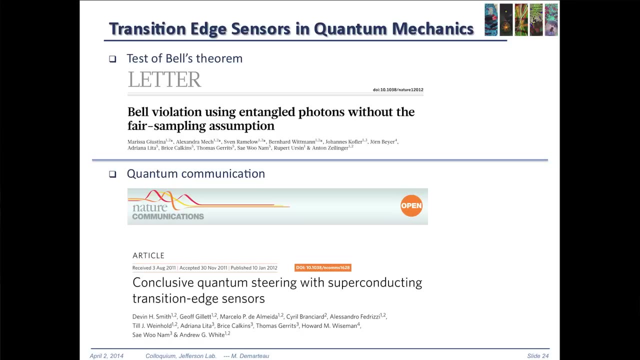 and you can see that with a transition head sensor you can distinguish all these individual peaks. Similarly for a biological application, because of their sensitivity And they're also being used to really look at fundamental measurements. Now, some detectors that we use are, you know, large. 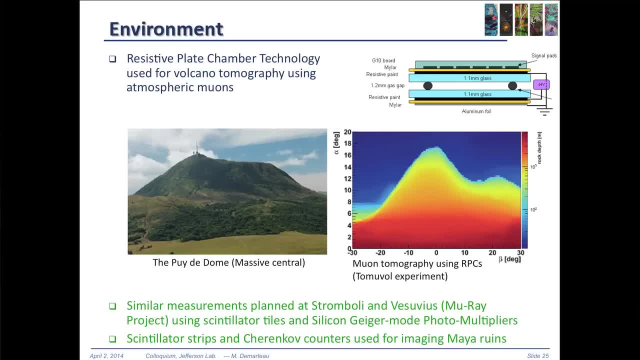 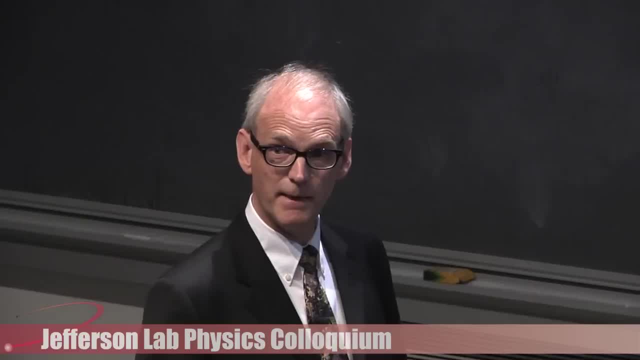 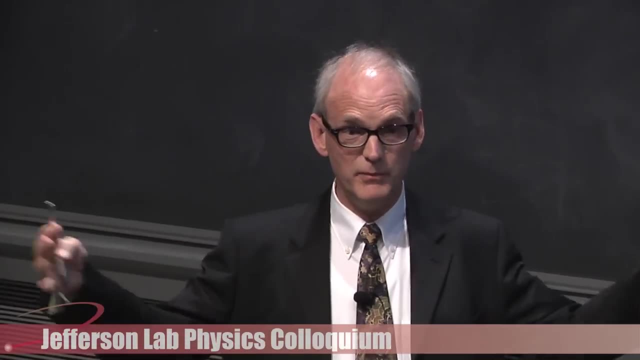 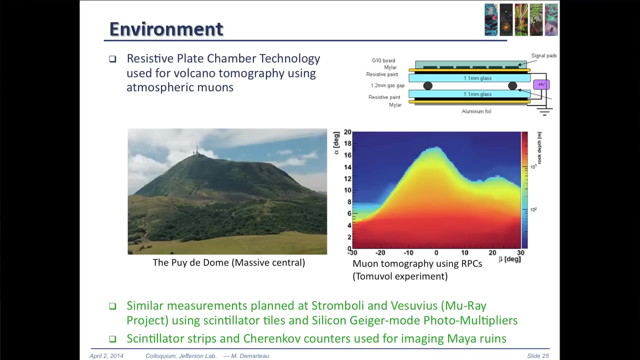 area and relatively cheap, like these resistive plate chambers. So in resistive plate chambers you have two plates filled with a gas system. Well, you know, the environmentalists have tried to use these to actually look at imaging, for example, an imaging of a dormant volcano. 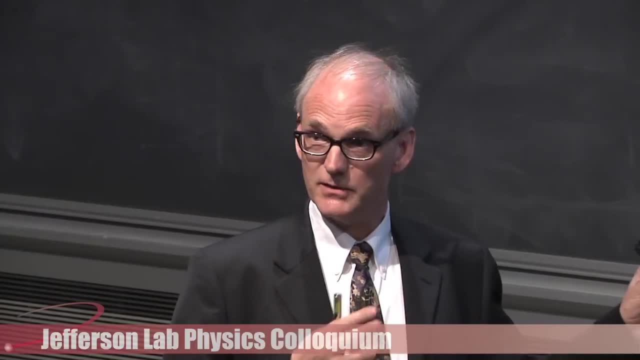 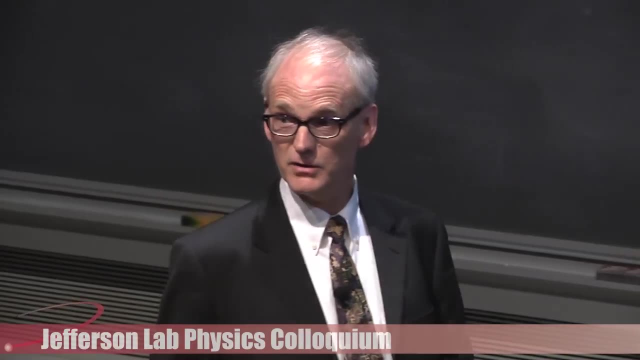 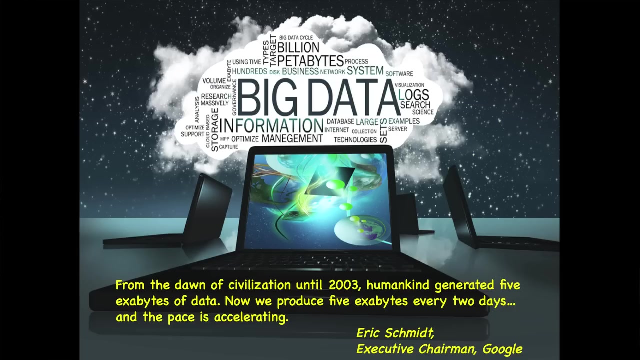 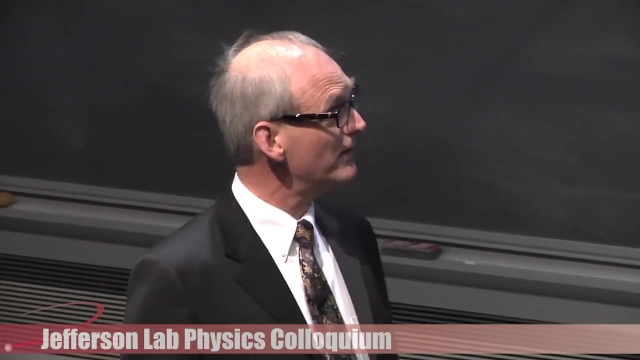 in France where they study, you know, the interior of the volcano. So that was all I wanted to say about particle physics. You know, particle physics is known for big data, But big data means something different these days than it did 10 years ago. 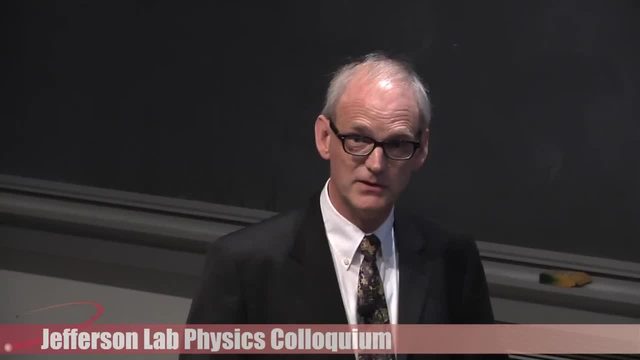 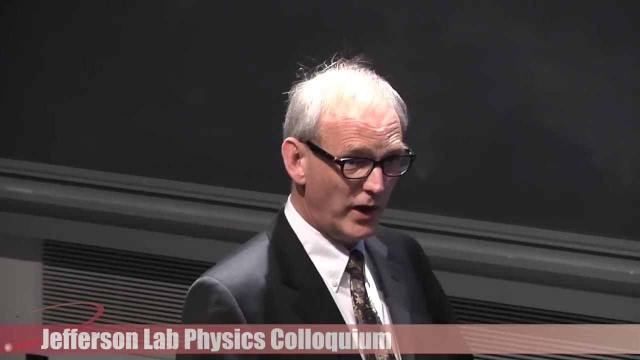 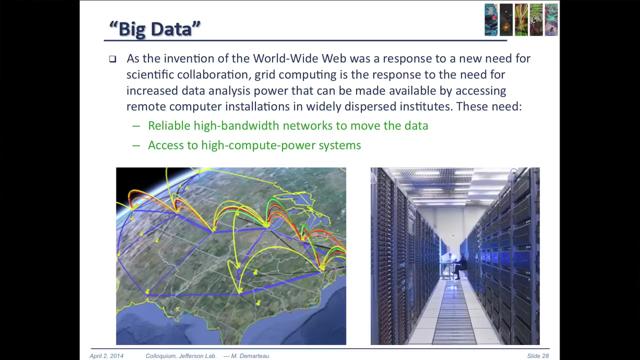 So, you know, Eric has the field that really pushes big data. So, as you all know, the world wide web was invented at CERN and that was a response to the need, you know, to the need for scientific collaboration. The grid is a response to the 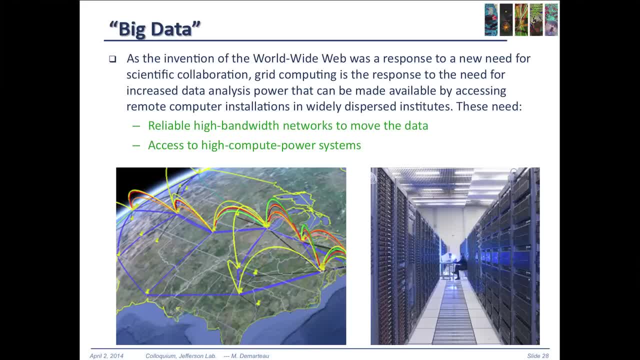 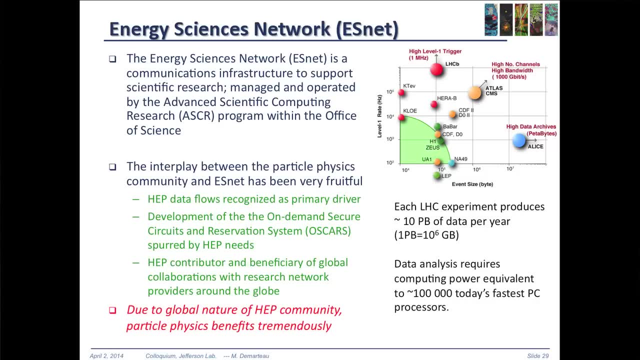 need to have high bandwidth networks and then access to these high compute power systems. So again, this shows you the problem that the LHC faced here is the event size in bytes versus the rate of these events, And this is what the particle physics community did as 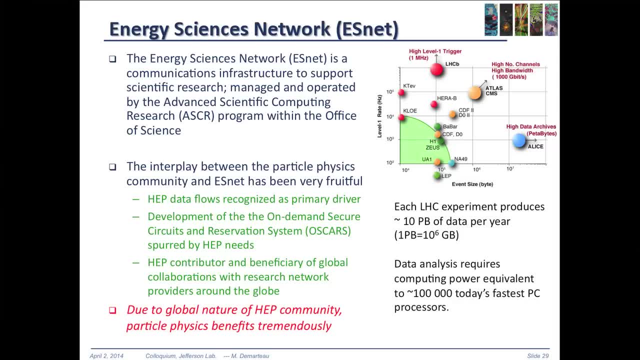 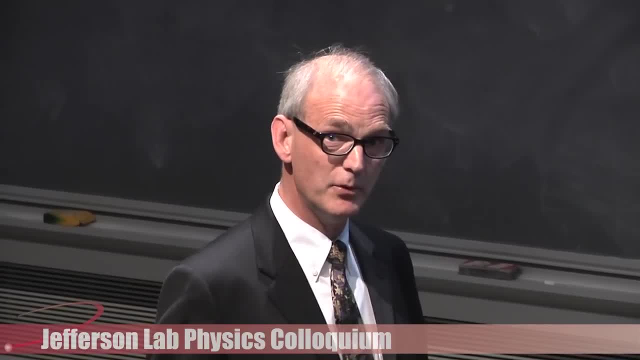 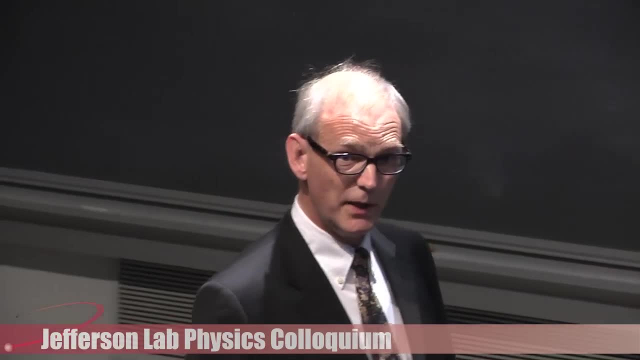 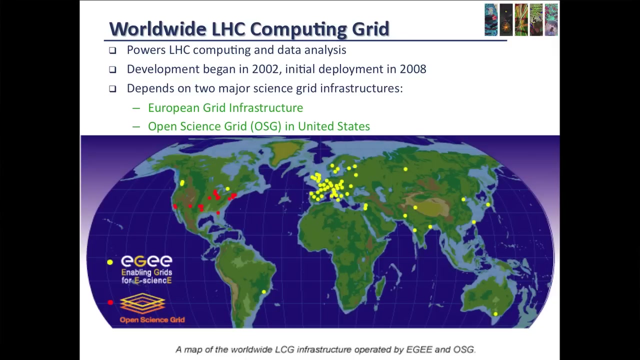 they worked with energy science network, ESNet, to really develop a system that met the needs of particle physics. So this was really an interaction, a collaboration between the two, between the computing science group and those built on two backbones: the European science grid infrastructure and the 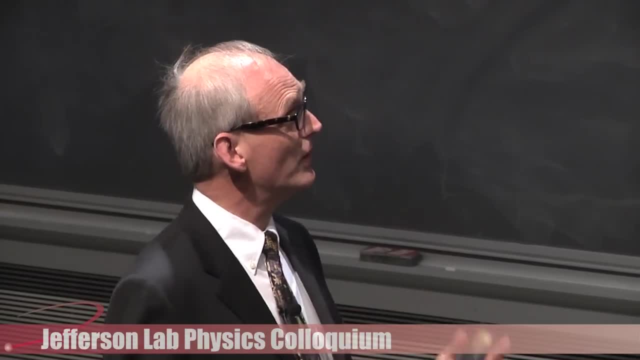 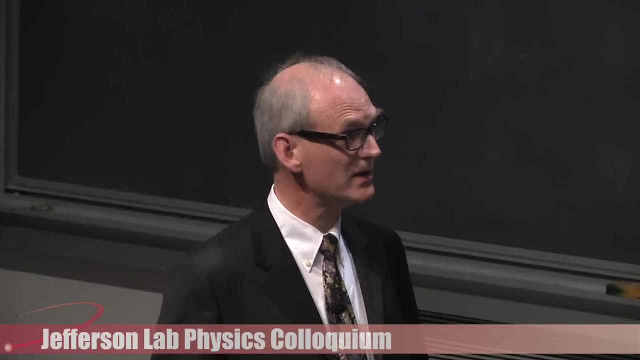 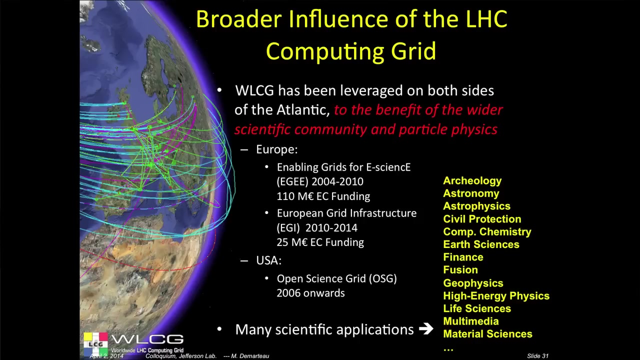 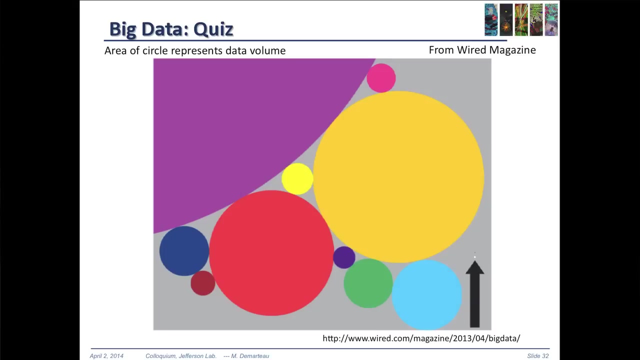 open science grid in the United States. And again, the tools were all developed and for grid computing, and now grid computing is not limited anymore to particle physics analysis. Now I would like to give you a quiz, and the reason why I give a quiz is I'll 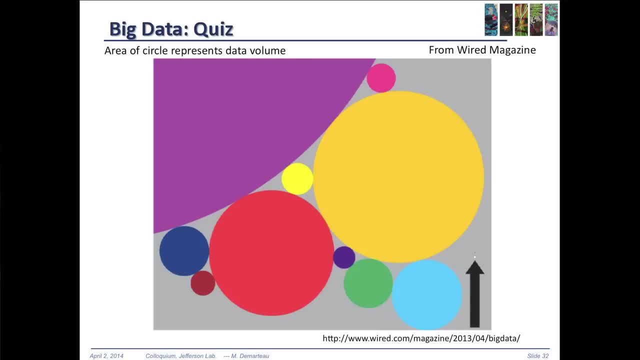 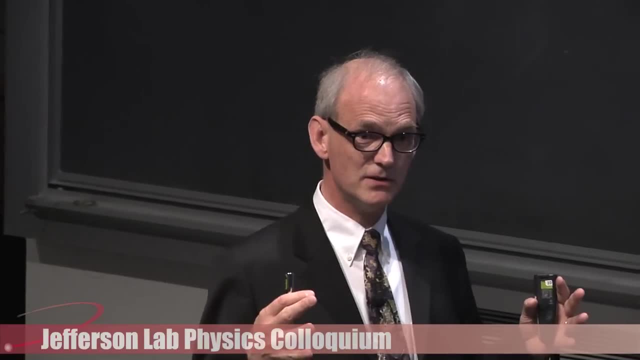 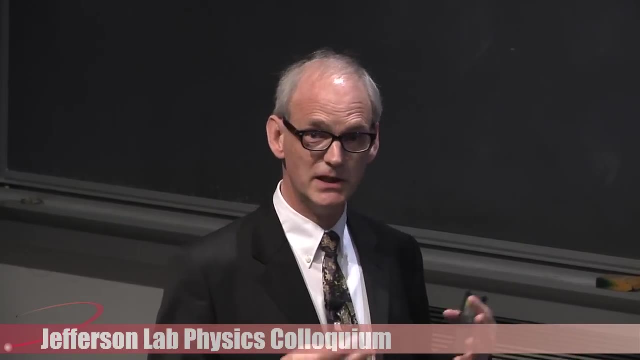 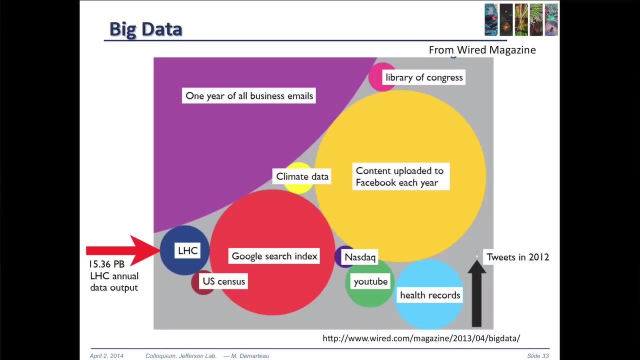 come back to that later. This is a quiz on big data and this is from Wired Magazine from last year. The size of the circle represents the size of the LHC data. I'll give you the answer. This is the LHC data. 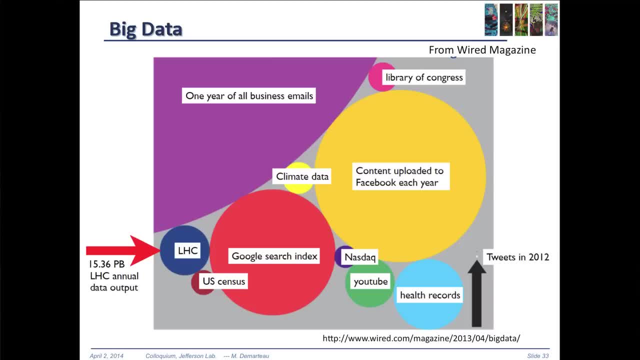 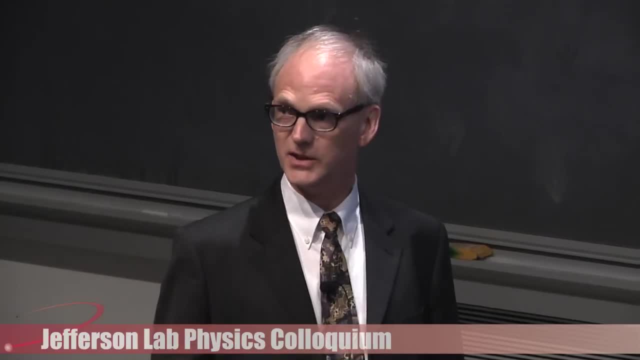 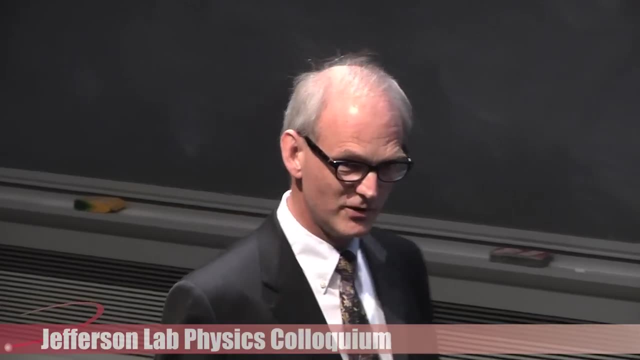 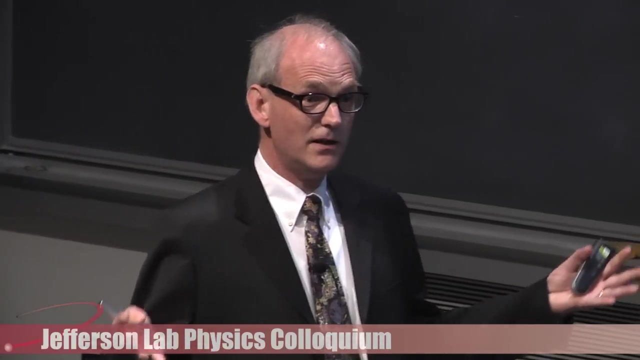 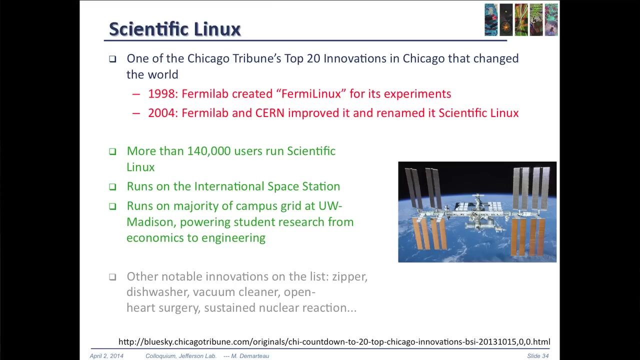 You can see that Facebook, which didn't exist- and this is important- Facebook, which didn't exist when the data was released. This is a picture of the docs that get uploaded every day on Facebook, Another thing that I think our energy physics can take credit for. 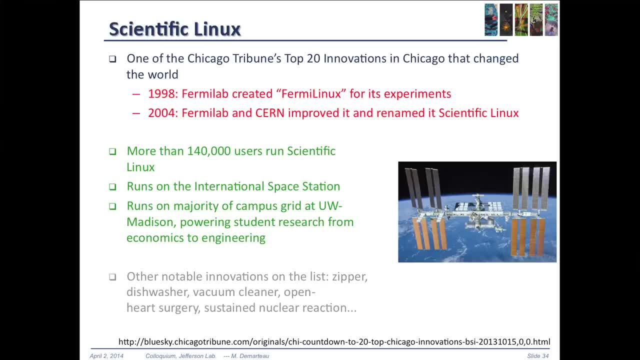 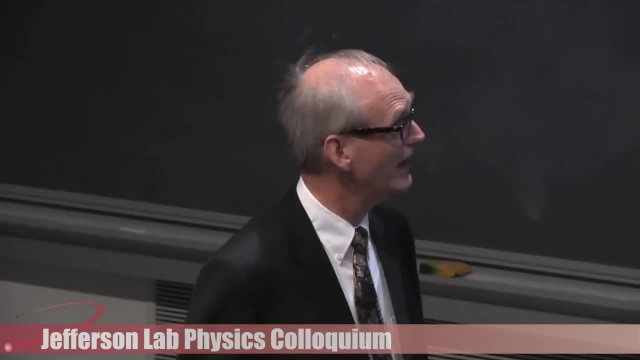 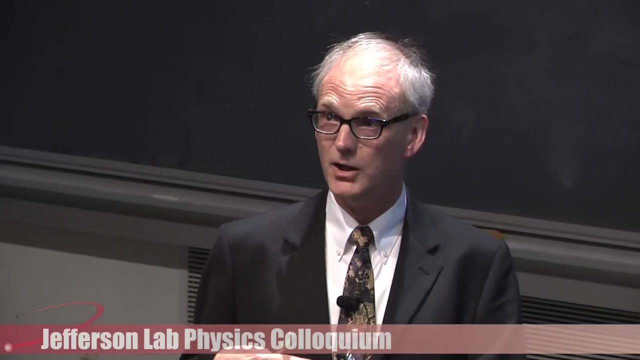 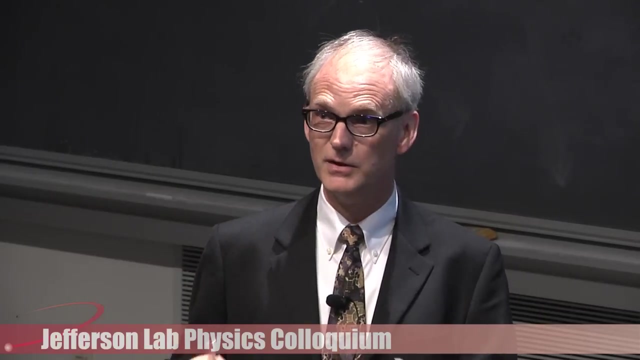 is the development in the Chicago area that happened. By the way, some of the other inventions in Chicago are listed here. It's interesting to see that it competes with the invention of the vacuum cleaner. Then another thing: This is where nuclear physics 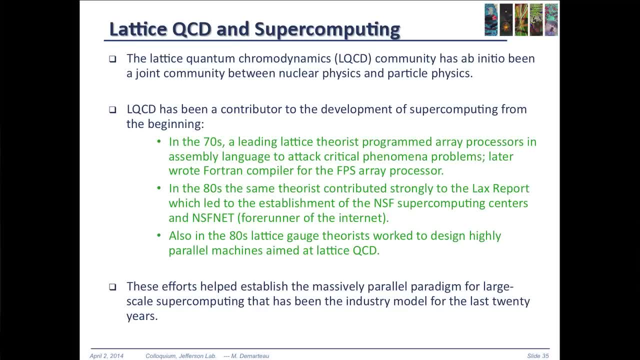 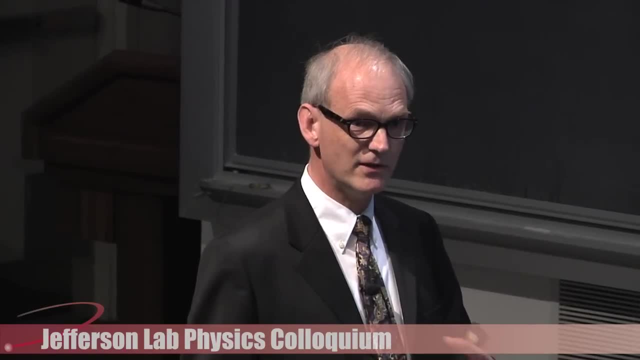 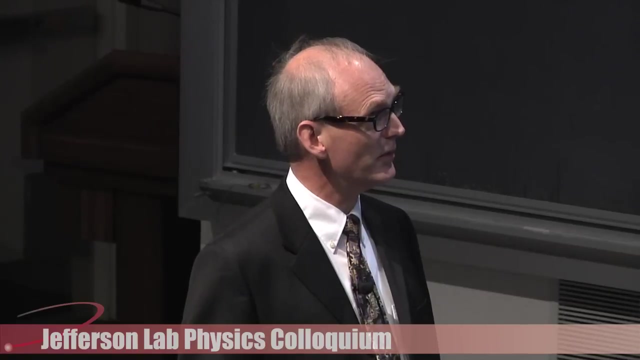 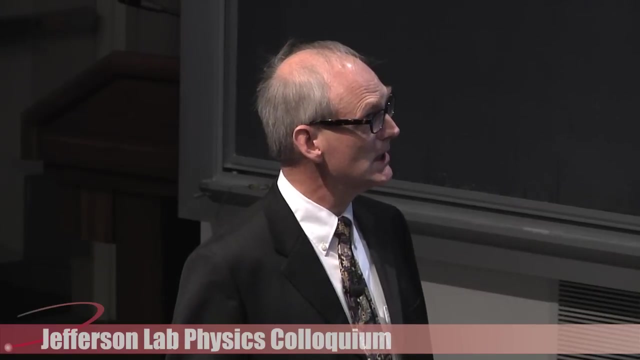 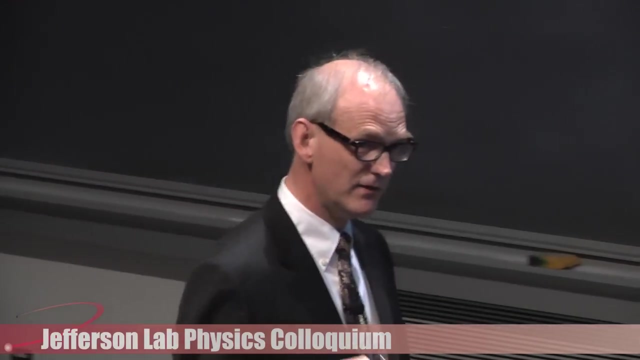 and quantum physics have a significant impact. That is, the development of supercomputing through lattice QCD. At one point, the theorist needed a way to tackle lattice QCD. In the beginning, the scientists started developing machines that were really aimed at. 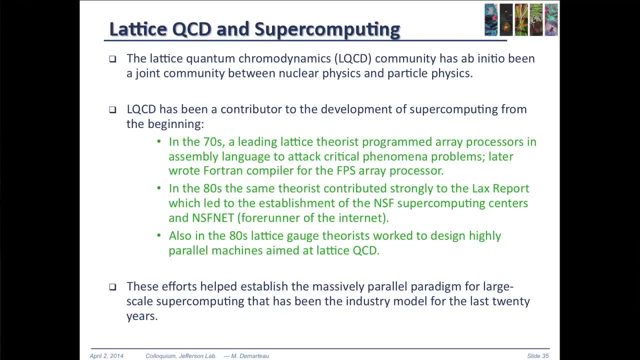 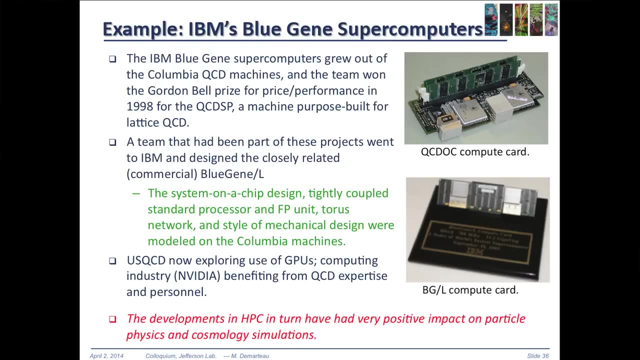 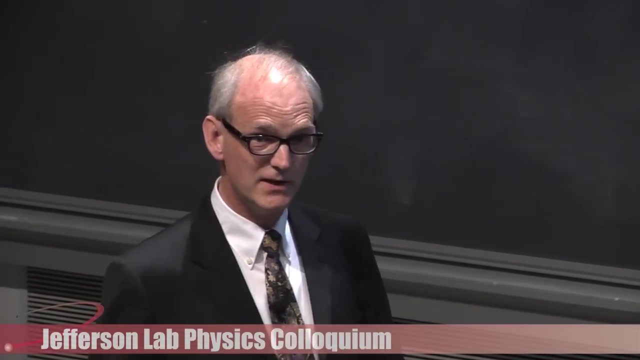 the performance of lattice QCD calculations. The initial effort there was an effort between the nuclear physics community and the blue gene supercomputers developed by IBM. A few of the key people who were involved in this project from the start actually moved to IBM to develop. 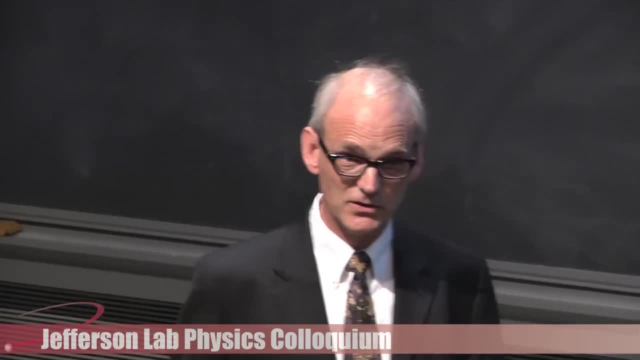 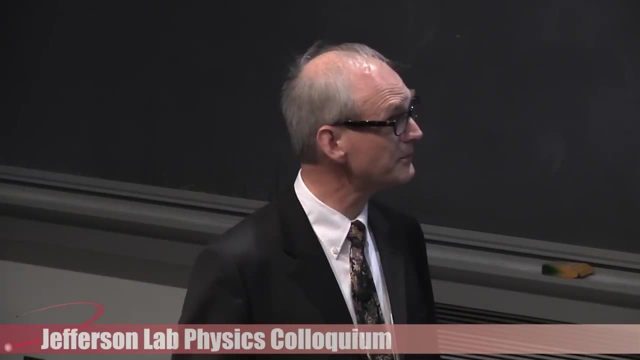 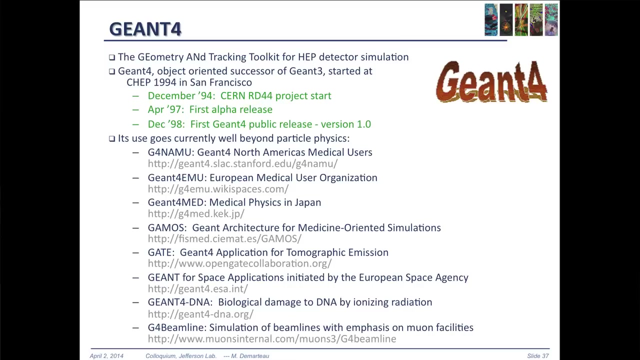 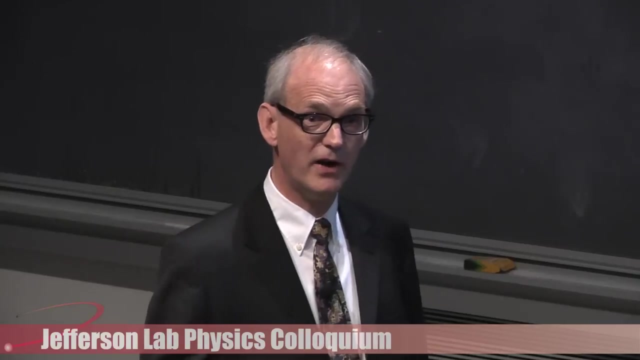 supercomputing And then again high-performance computing. these days is being used in the nuclear physics community. Another thing that many people may not be aware of is GEON4.. I don't know how well it is used within the nuclear physics. 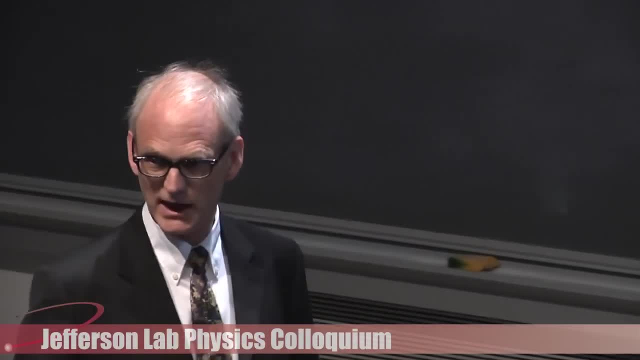 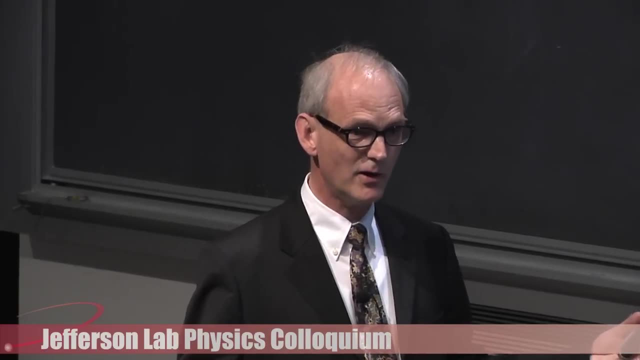 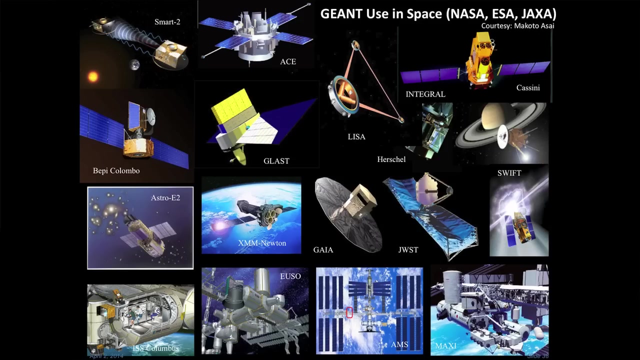 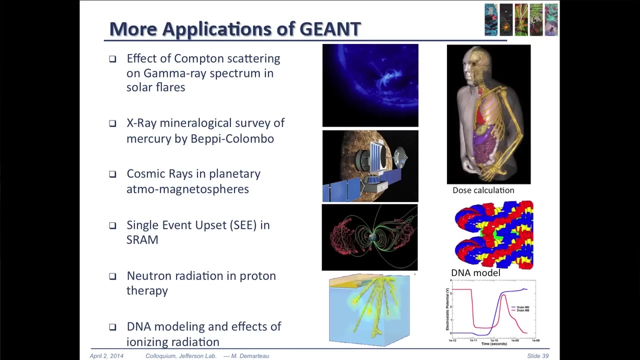 community, but it has been used in the nuclear physics community for many years. It has been used in the nuclear physics community for a number of years. You know, planetary missions are even being used now to study for DNA models. They look again. 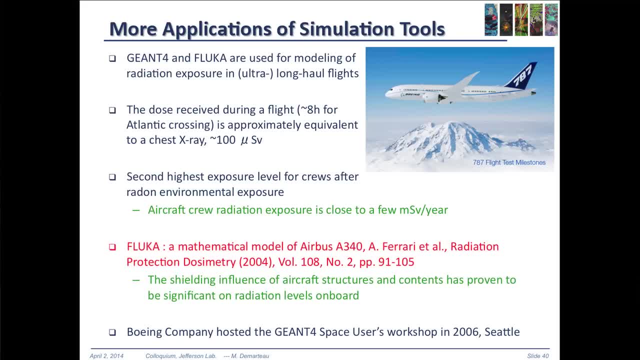 for medical imaging, and even single event upsets are being studied with GEON, And another thing that's really interesting is that there's a paper on it, and even before I started this study myself, I was not aware of this paper where it 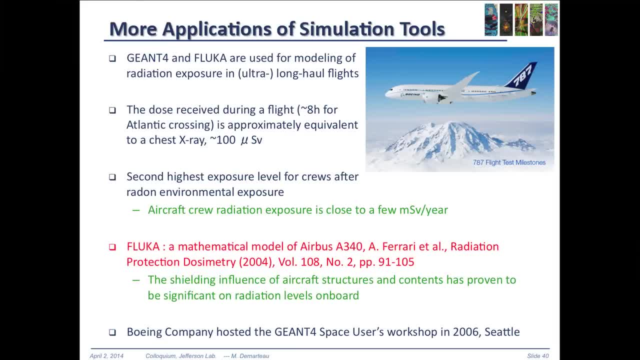 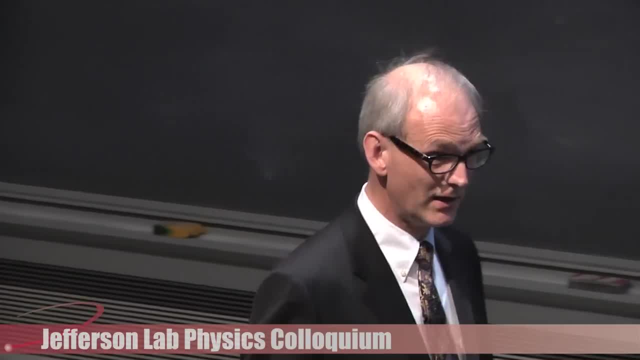 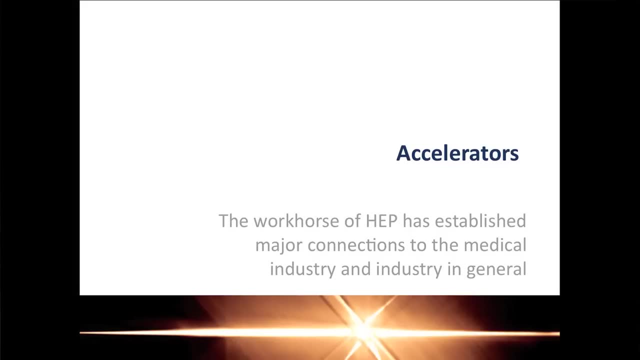 is interesting to see that particle physics is actually trying to design an air bus and look at what it's doing. OK, then we come to accelerators. So accelerators, as you all know, is the workhorse for particle physics. So 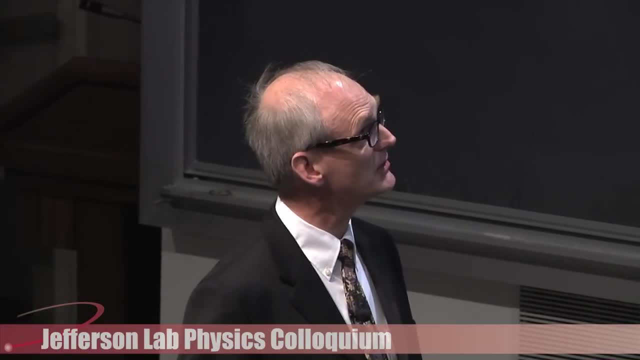 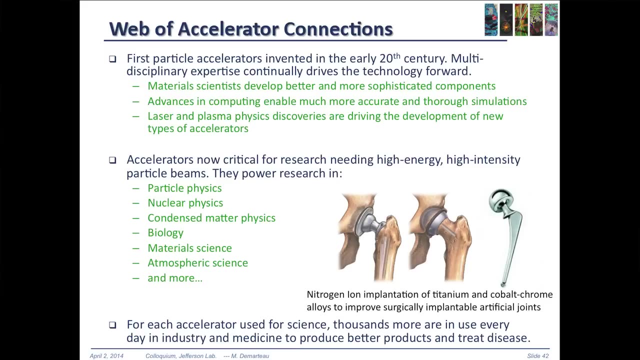 at the moment. they are being used in a broad range of applications, So they're used for being driven by particle accelerators, And here again is a list of topics where accelerators are being used. So anyone, for example, 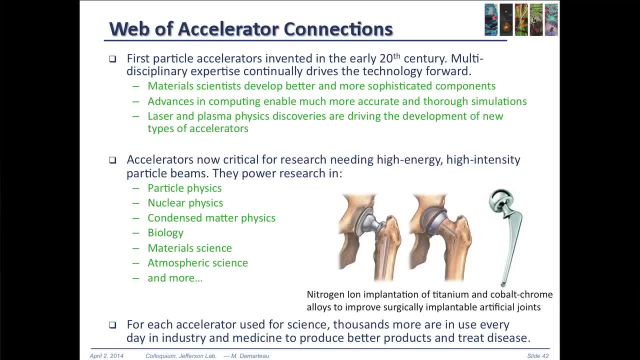 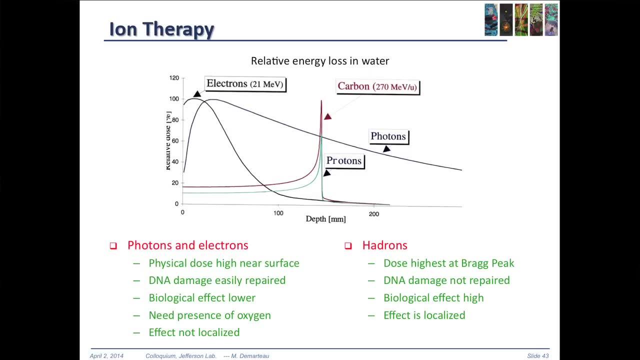 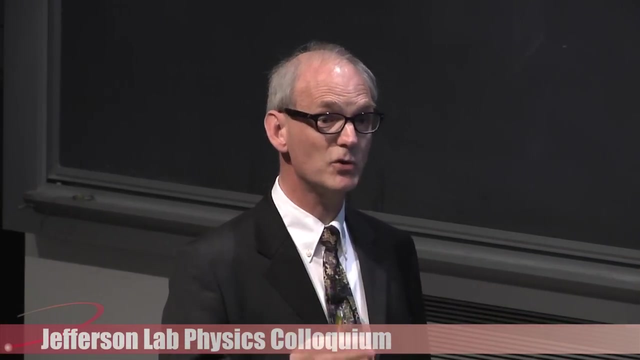 who has an artificial hip or something. your hip has to be driven by a particle that is moving in the same direction as the particle is moving in the same direction as the particle is moving in the same direction. so for specific tumors, you know, ion therapy. 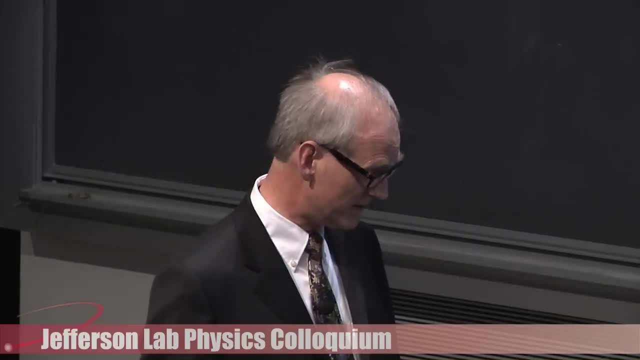 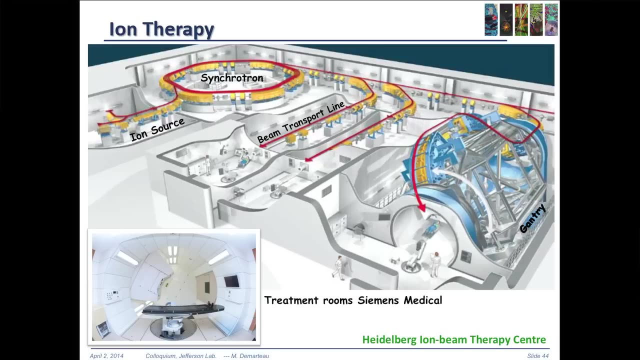 is really the most ideal therapy to treat certain forms of cancer. So this is a picture of the Heidelberg Ion Therapy Center in Heidelberg And, as you can see, it is very similar to, you know, the other scientific laboratory that we. 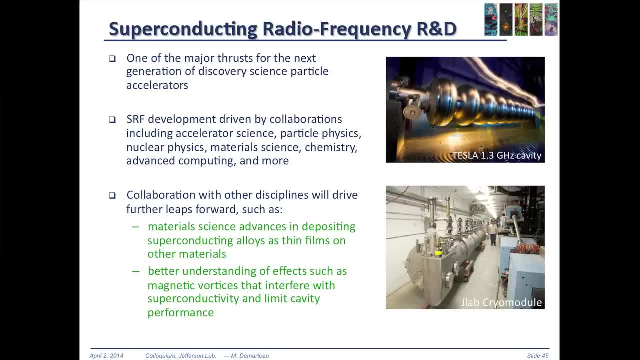 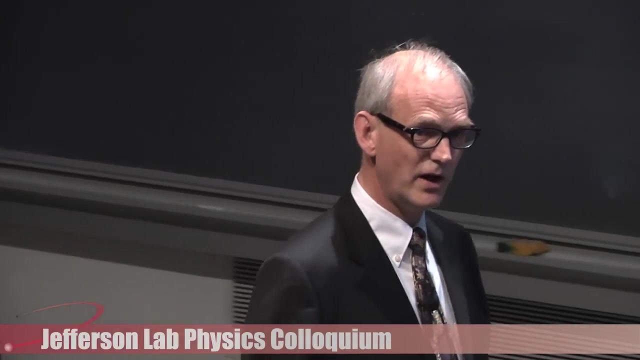 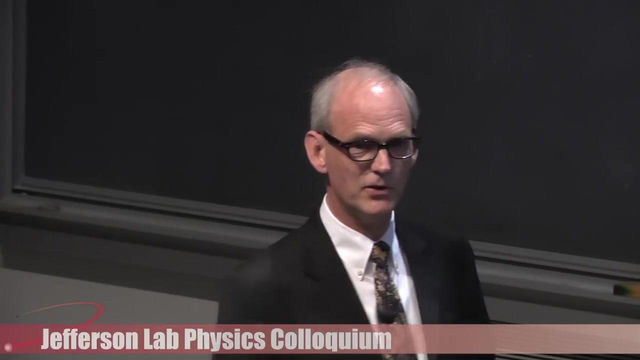 have here to treat patients. Then we have superconducting RF, where actually nuclear physics is a major leader in that. So it's a disciplines that really will drive this technology and this further, because we need the interaction with the material scientists to understand you know where. 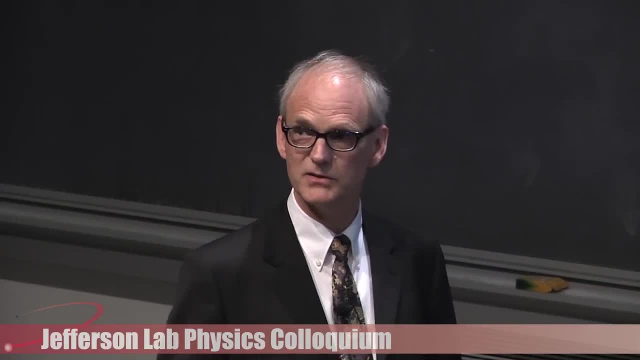 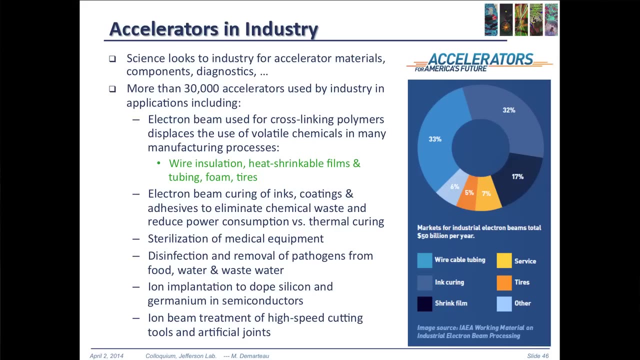 a cavity, for example, breaks down or why you cannot reach the gradients that you actually want to want to achieve. now. accelerators are used in industry almost everywhere you know, from from disinfection of water to ion implantation for silicon devices to to, you know, each ring films. now you all. 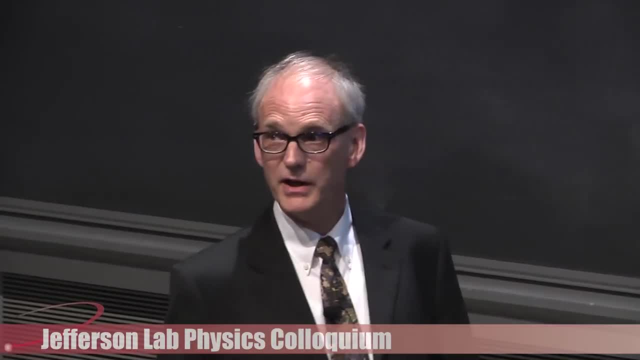 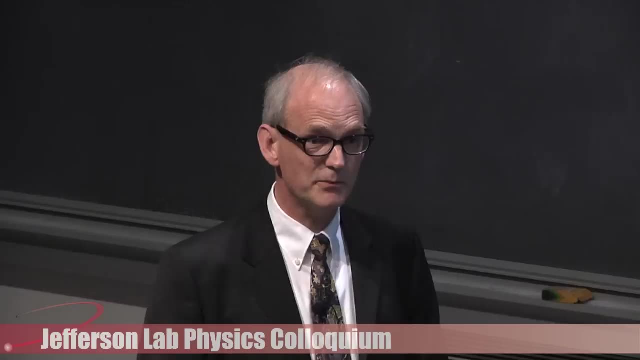 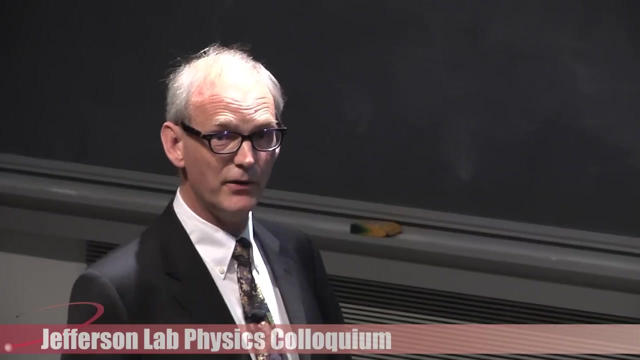 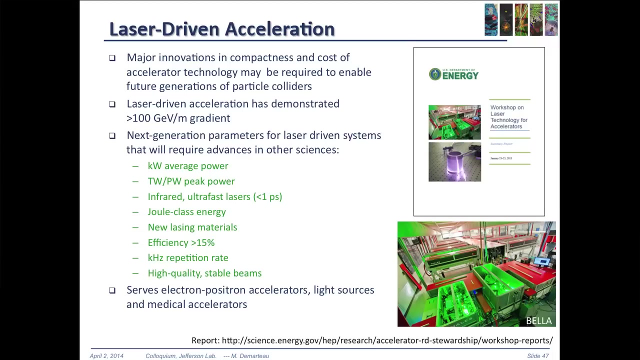 know also that we are starting to reach a limit with the scalability of of accelerators. they're just becoming quite unaffordable. you so one way to break that barrier is maybe through laser driven acceleration. but- and this may really be required to enable us to make our next generation of. 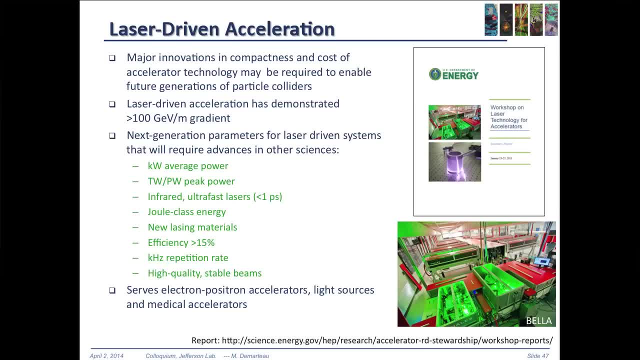 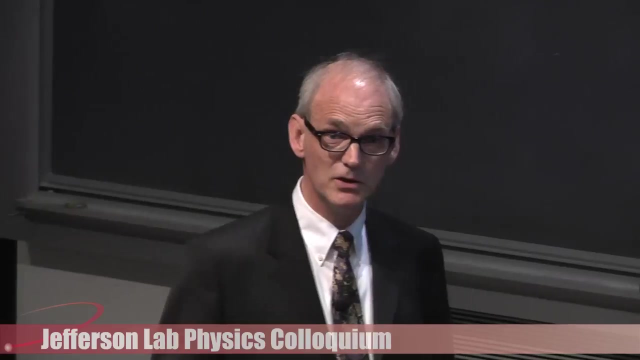 particle colliders. but what this relies on is really advances in in areas of science that are beyond particle physics, because here you really need lasers, for example, that have kilowatt average power, with terawatt or petawatt peak powers, you know, with a large efficiency and with a high rep rate. so particle 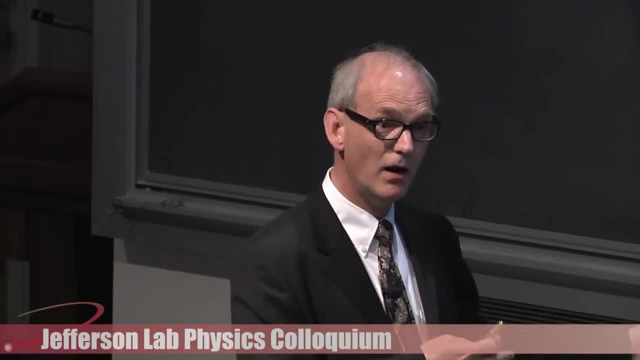 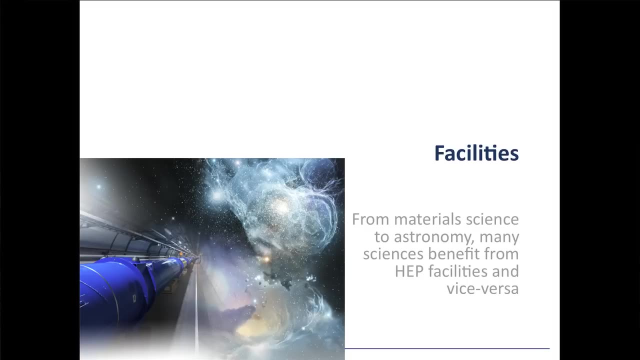 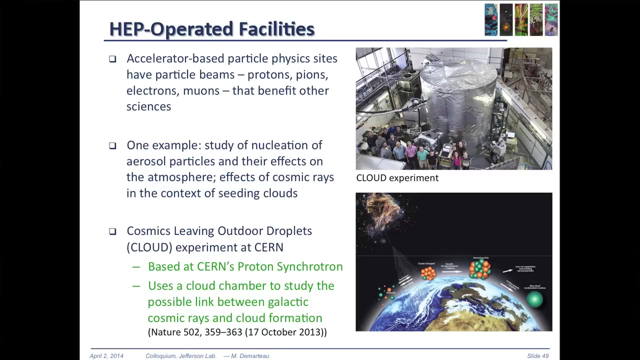 physics will become more and more dependent on these other technologies. the last topic is a few words about facilities. so we have HEP operated facilities, so particle accelerator based particle facilities. but one very nice example, for example, is the. the test beam at CERN was used for a cloud experiment and the cloud. 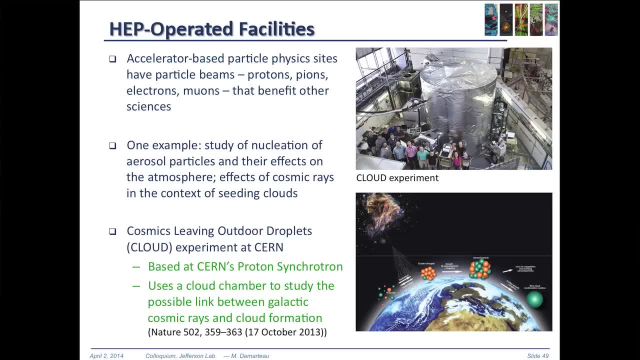 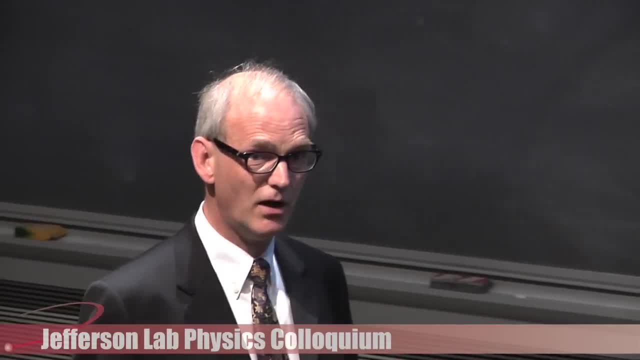 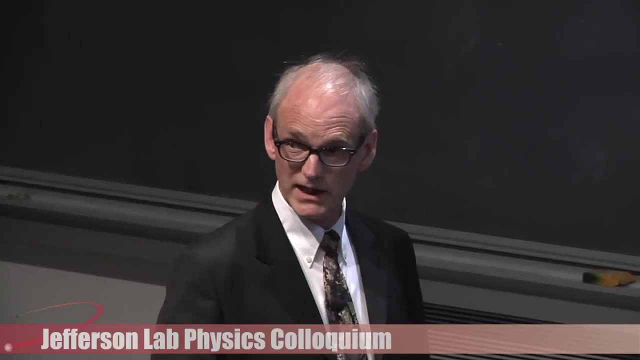 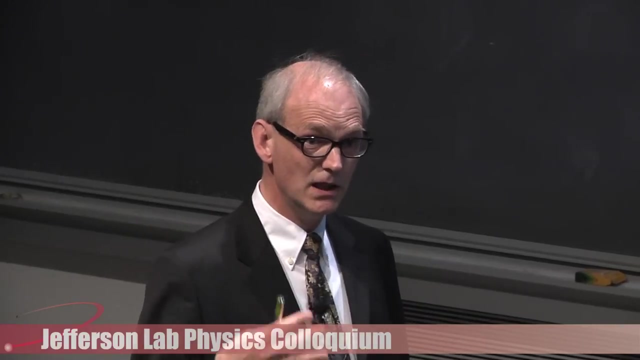 experiment stands for cosmics leaving outdoor droplets. that is an experiment that is looking at the formation of aerosols and the formation of clouds using aerosol particles in the sky. So it's really an atmospheric study where they use particle physics facilities to actually get at that science. 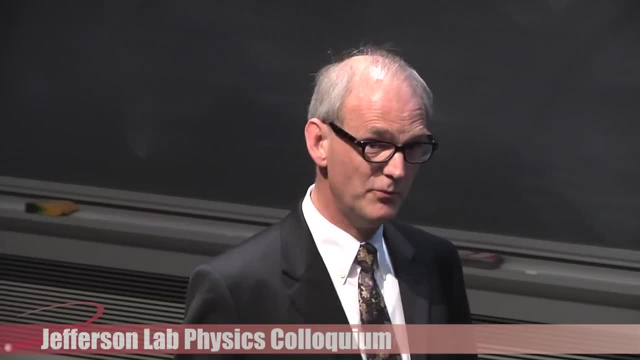 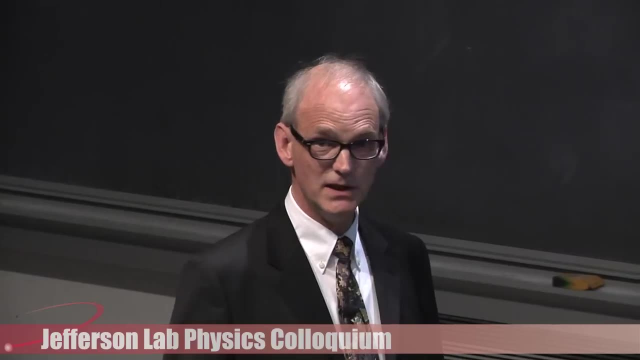 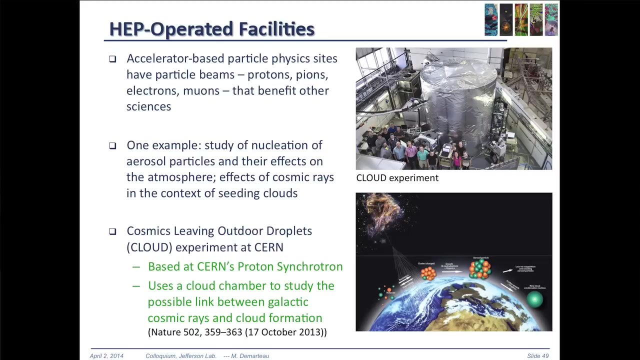 And the reason why particle physicists can do that is they can provide them with particular beams that simulate cosmics and they can provide the environments that they need, For example, the very ultra-high vacuum environments that we have for the beams, and in this particular, 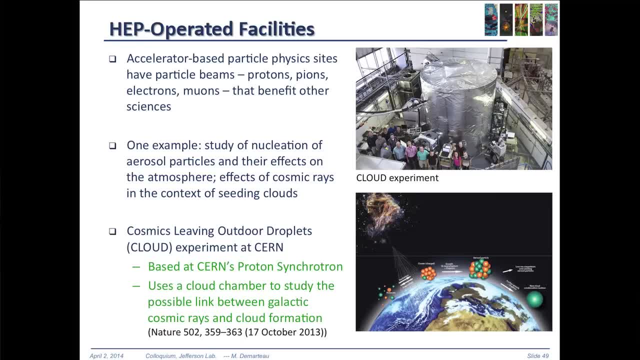 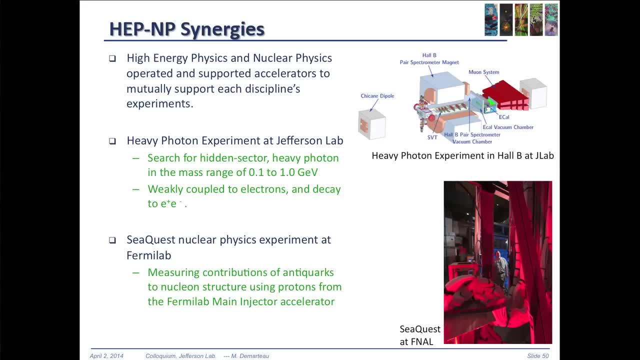 case in this huge vessel. One thing that is very appealing to me is the sharing of facilities already between the different disciplines. So here we have a particle physics experiment. you know, the heavy photon experiment that is, I think, a particle physics experiment, but it's taking place here in Hobie. 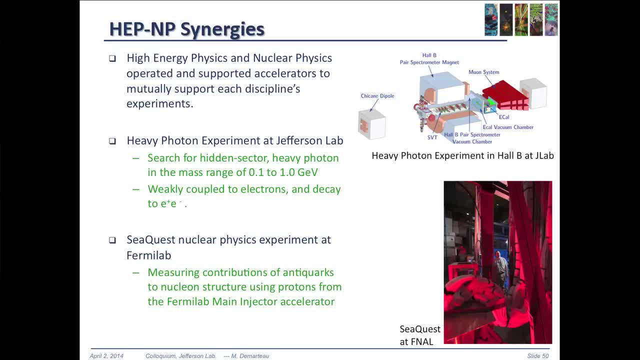 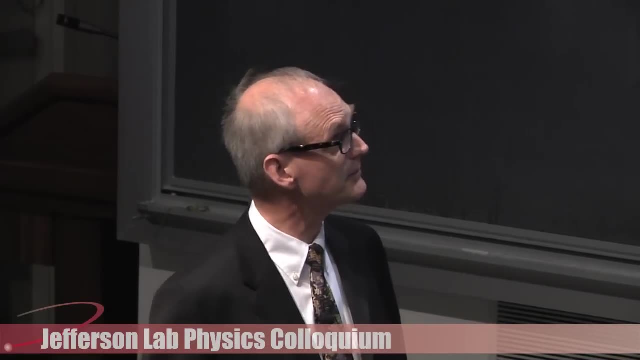 At the same time, there is the experiment sequence. It really looks at the composition of the sea inside a proton which is, you know, falls under nuclear physics, which is actually taking place at Fermilab, And I really believe that we should have much more of that. 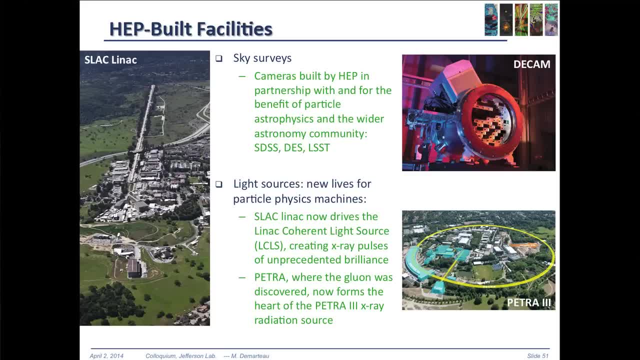 And we also have built facilities, facilities that are really built by particle physics. So we built, for example, the sky surveys Fermilab, built the dark energy camera, which is just an array of of about 60 or so CCDs to carry out these sky surveys, to look at dark energies. 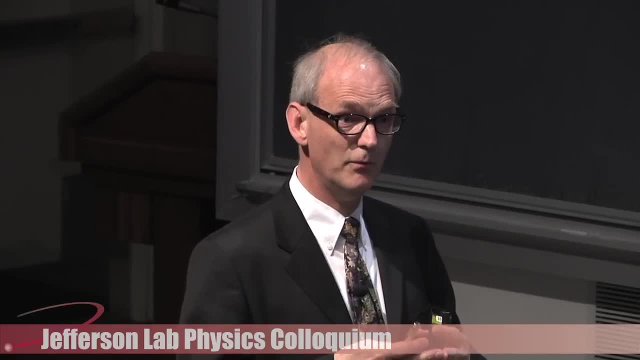 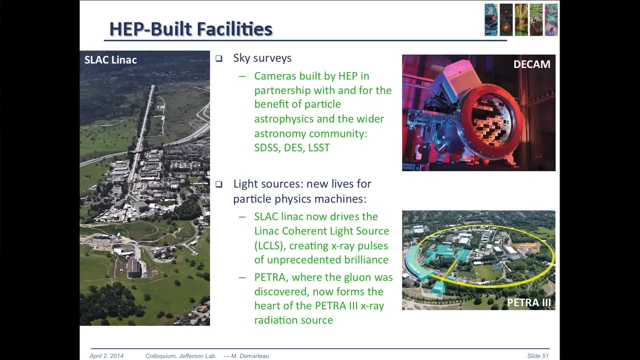 It's built by high energy physics but it really benefits a much broader community. And then you know we have these huge infrastructures like SLAC and, you know, PETRA at DAISY that are now being used as light sources. where you know, basic energy sciences can just come. 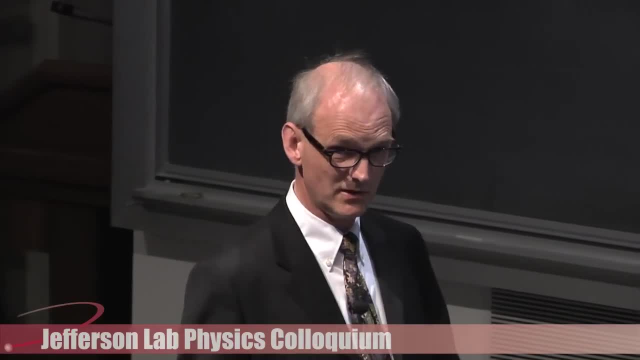 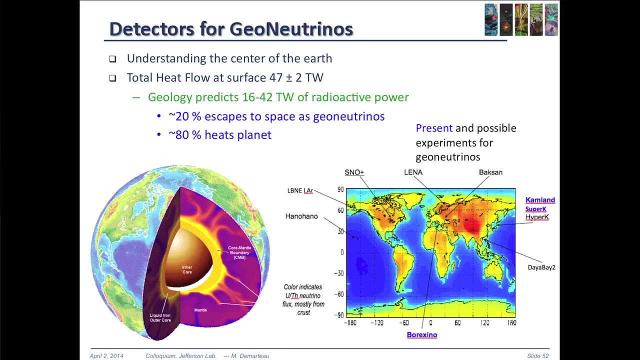 in and use their facilities, These large facilities, these large investments in infrastructure for their physics. Then we have detectors that can be used for, really for geophysics. I mean, some people say that we understand the inner core of the sun better than we understand. 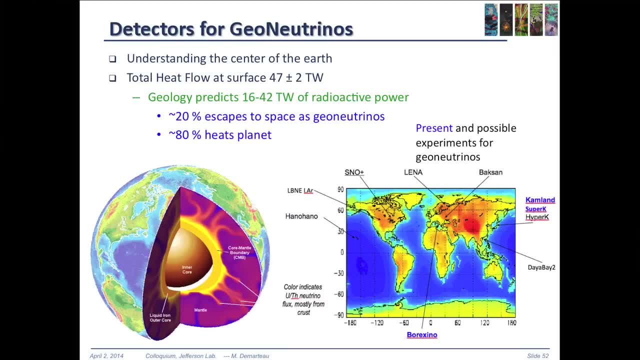 the inner core of the planet that we live on. But one way to study actually the inner core of the Earth is to look at geonatrinos. So you know the neutrino's coming off of the interactions in the Earth and the experiments. 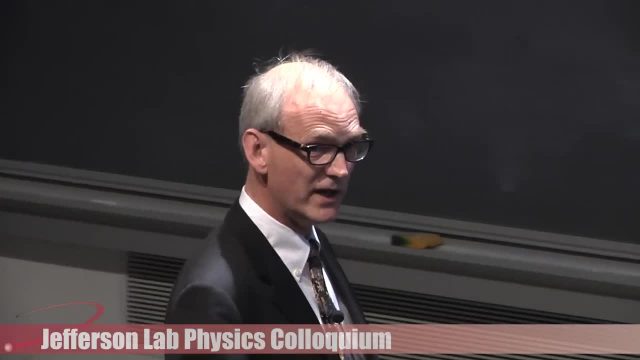 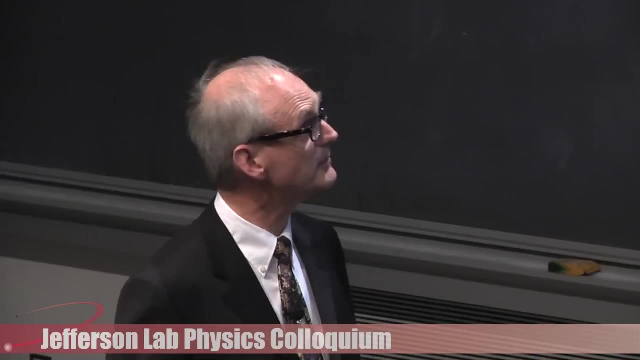 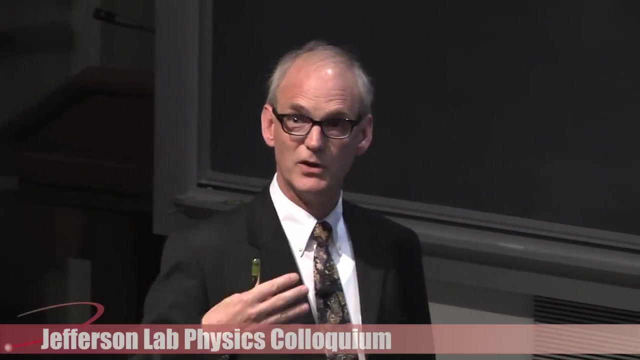 that we have the large neutrino experiments that we can have could actually be very beneficial. It could serve, you know, the geophysical community rather than just our own community, And then we could go a step forward. I mean, if we are going into the direction of muons, for example at Fermilab, you know, 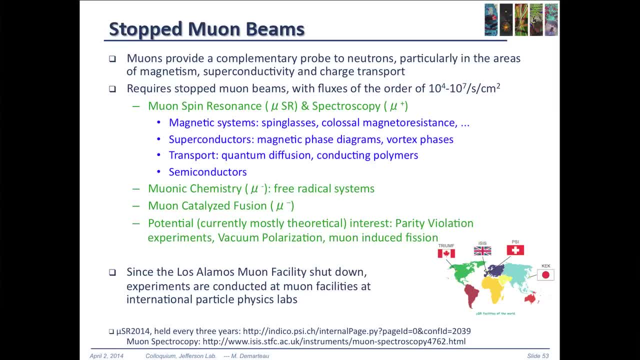 they're trying to create muon beams. maybe one could think of creating a facility for stopped muon beams. At the moment, the US does not have a stopped muon beam. US does not have a stopped muon beam facility anymore. 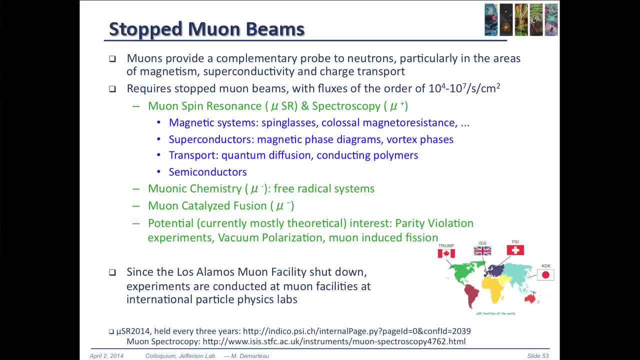 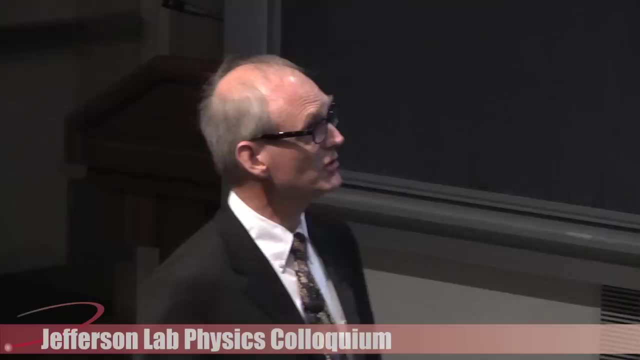 We had one at Los Alamos. it was shut down And now to do any one of those studies, you know people have to go overseas And muon spin resonance is a very sensitive probe, especially for material science. So this is being used to look especially at superconductors, at magnetic phase diagrams. 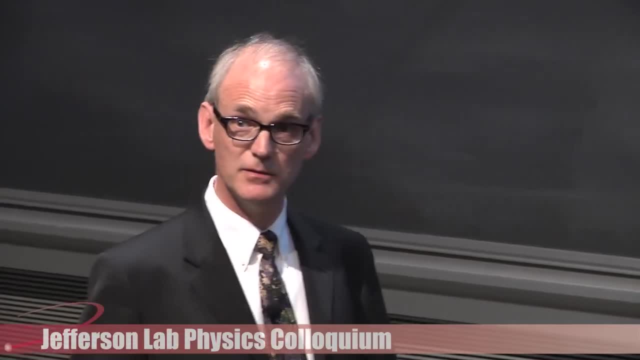 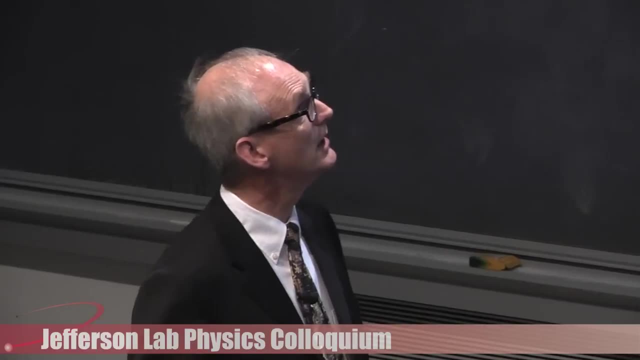 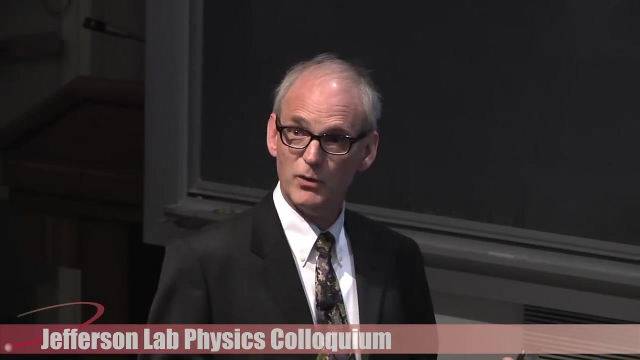 and that facility could be provided by, for example, a nuclear reactor, For example particle physics, for, you know, the benefit of a broader society. So I would like to conclude then here. So I think what I tried to do is to show that there is a web of connections of particle. 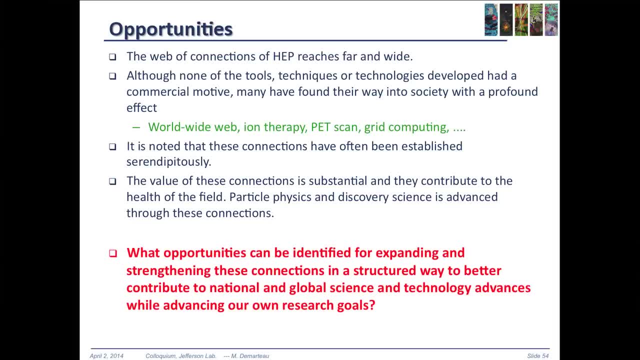 physics to other science disciplines in the society, and that web is rather broad And none of the two tools that were developed at particle physics had any of those applications in mind. It was just purely curiosity-driven basic science, But it found its way into broader society. 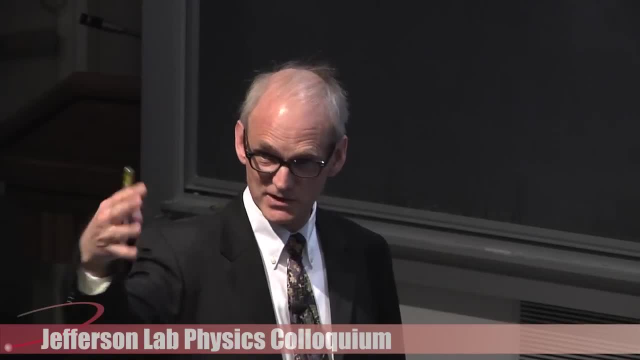 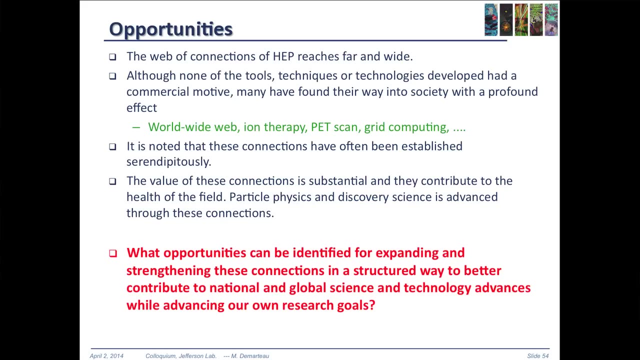 And often the path these inventions and these developments have followed was rather serendipitous, just by chance. But the value of these connections, I believe, is rather substantial. But the question is what opportunities can be identified. What opportunities can be identified? 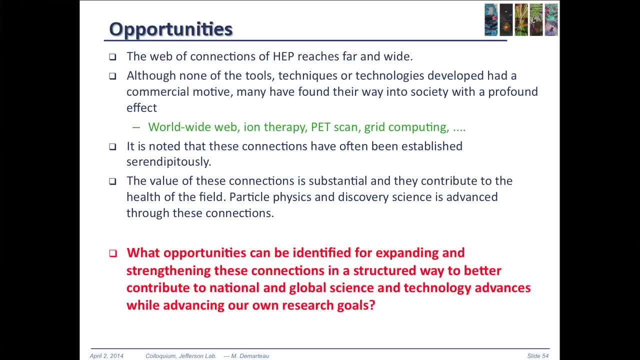 What opportunities can be identified? How can these connections be expanded? What are the advantages and disadvantages, And are these connections weiterembles to the next level? How can we understand our customers and how long they'll last, And what can we do to improve our experience, to make use of the technologies that we've? 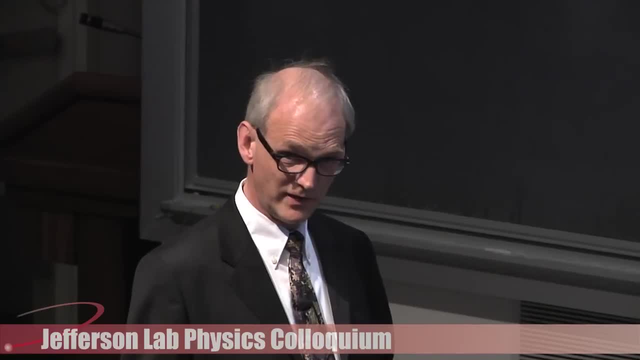 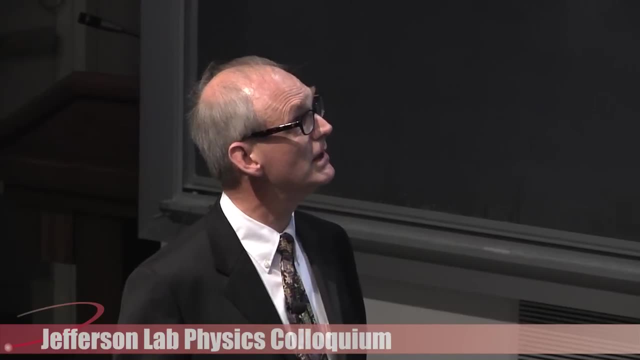 developed in the past. My goal was to present a way for the technology to expand and strengthen these connections in a structured way that helps all of us, that helps you know advanced science, helps advanced technology and helps you know benefits for society. 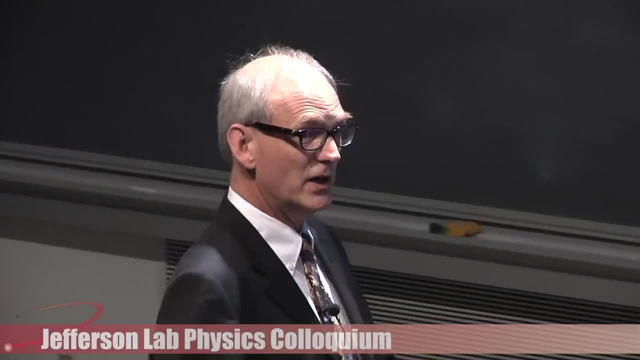 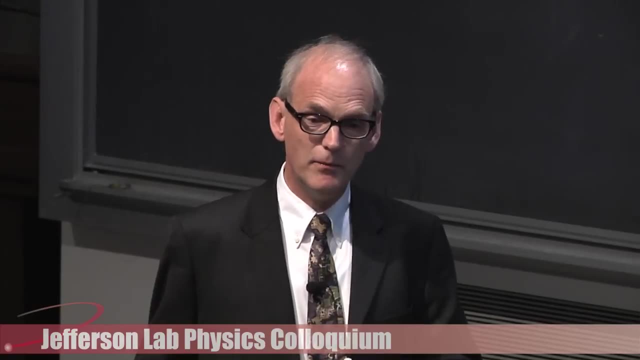 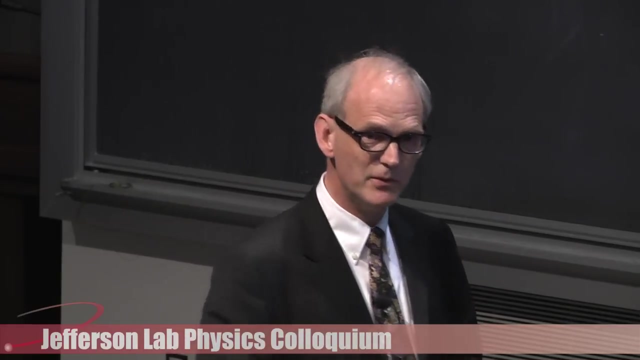 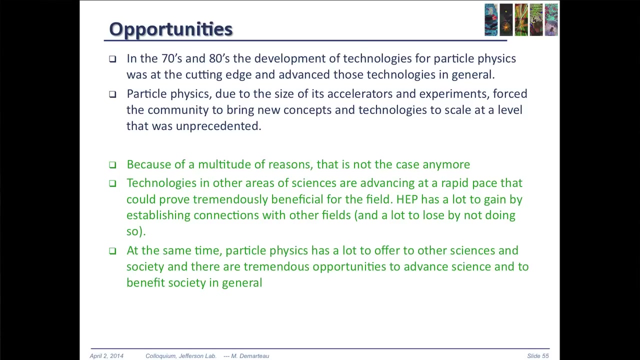 So the reason why I showed you this quiz about with Facebook is that quite a while back you know, especially for particle physics, The developments that were being done by particle physics were in sync with the developments in industry. We actually pushed industries in many aspects. 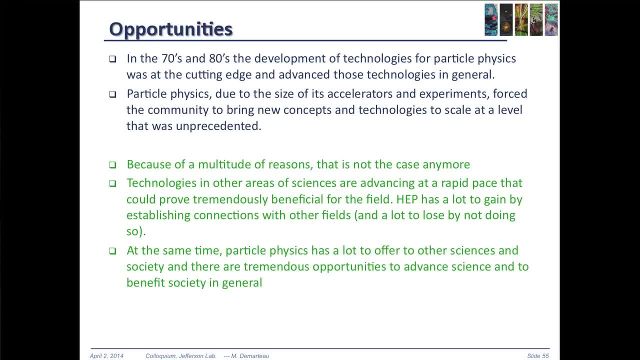 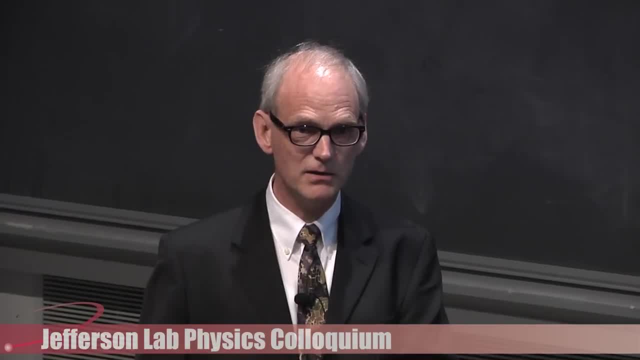 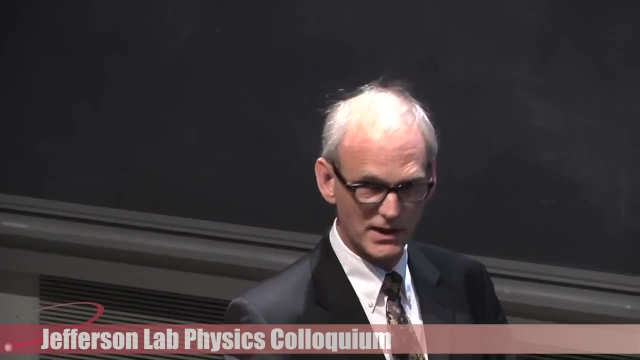 For example with the silicon technology, with the development of the integrated circuits. the requirement of our particle physics to make integrated circuits radiation hard gave industry new ideas. They came up with ways to enclose transistors in an IC And the other advantage of particle physics. 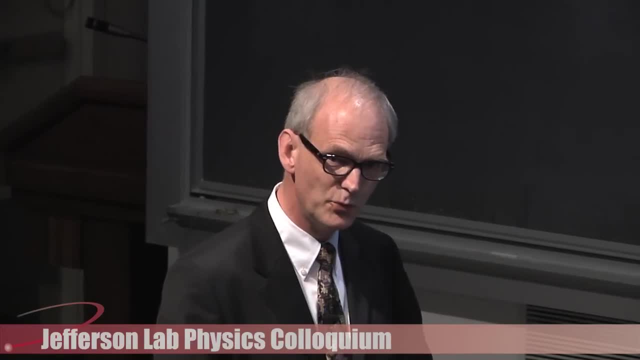 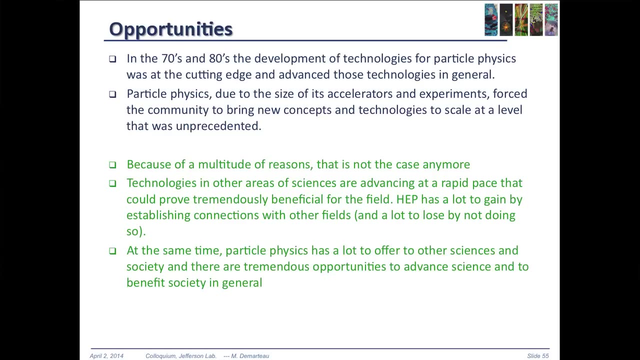 is that particle physics is required to bring these technologies to scale and make them work. But because of a multitude of reasons, that is not the case anymore. Projects within particle physics take a very long time, And there are technologies in other areas of science. 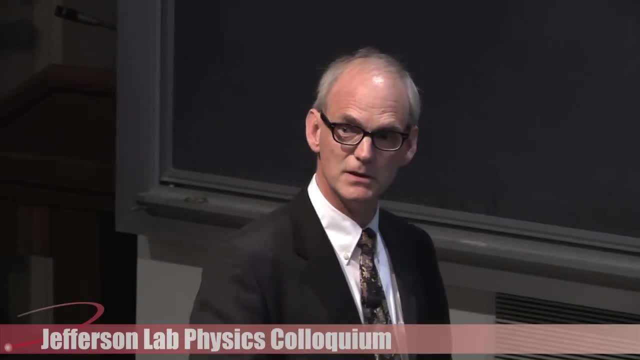 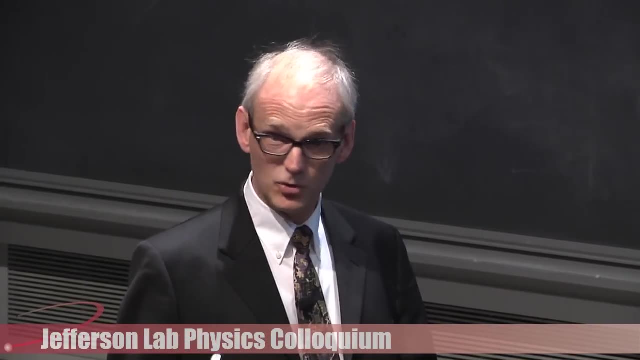 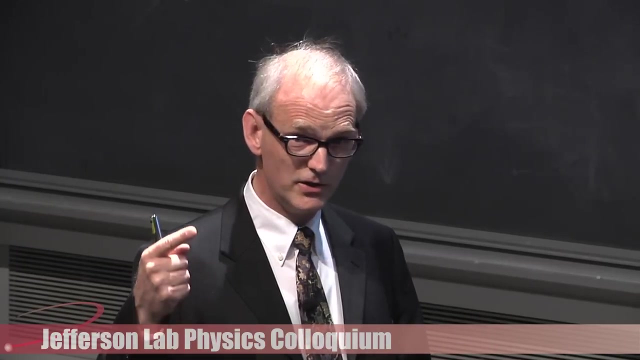 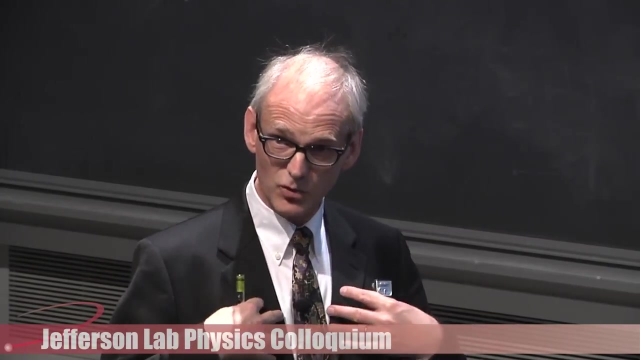 that just have overcome us. As I said, when the LHC was written down on a piece of paper, Google didn't exist, Facebook didn't exist, And now their demands on getting access to data and transporting data over this infrastructure is much larger, much higher than what we need. 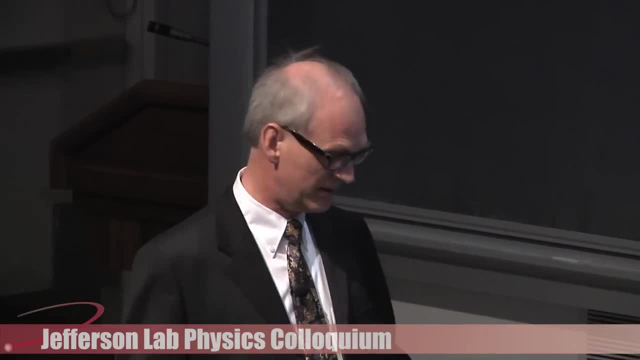 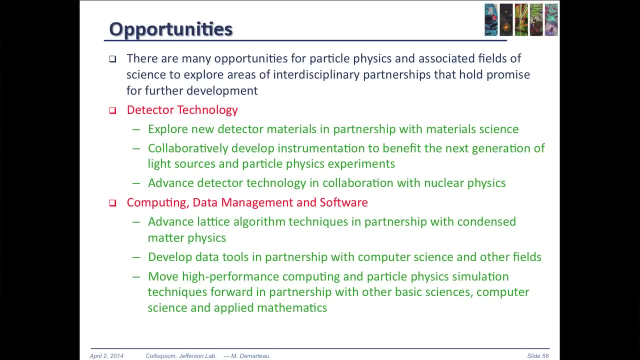 So we have to take a new look at that. So what are the opportunities? I believe that there are plenty of opportunities for groups to work together to form collaborative efforts. So in the technology, I really think that the field has to look at partnering with other fields. 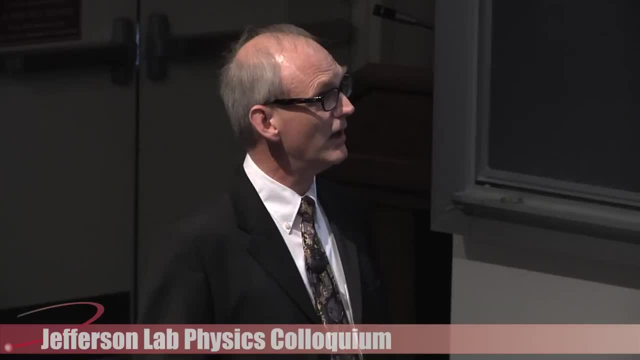 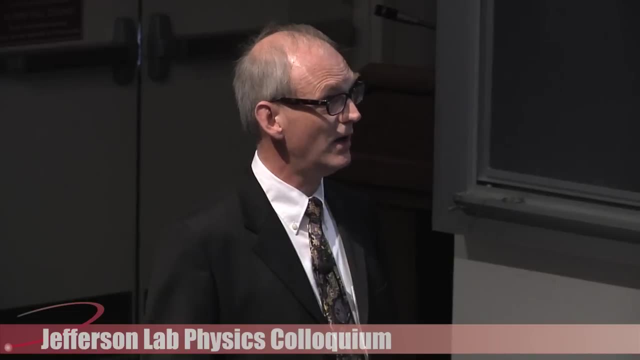 like material science. I do think that we could work with the light sources here in the country to develop better detectors for the light sources, And I think we should partner up in a more coherent and a more collaborative way with nuclear physics. The same for computing and data management. 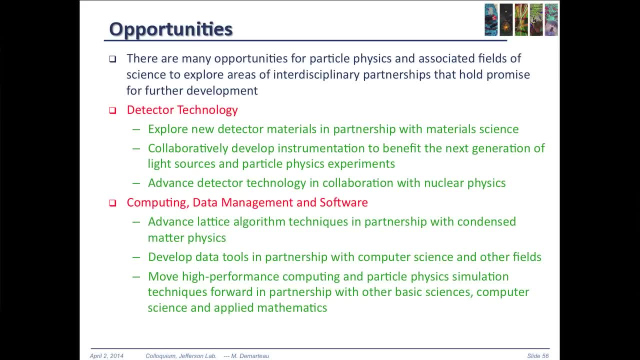 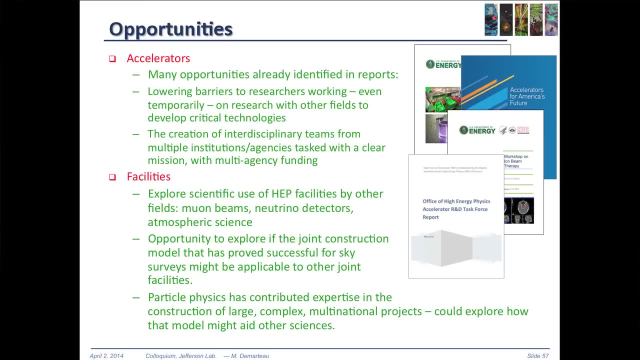 There are a lot of things that we can do, especially in the area of high-performance computing, where we could really benefit, And in accelerators. I think it has been documented quite well in these four reports that you can find on the web. 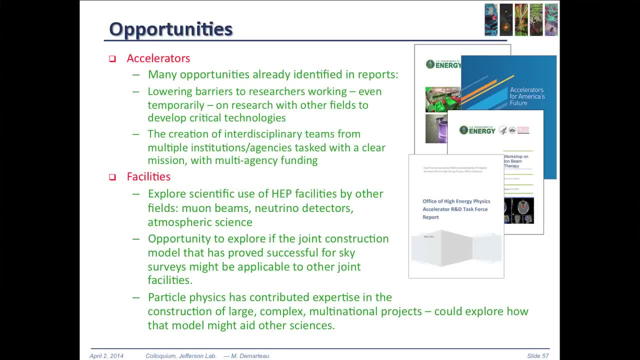 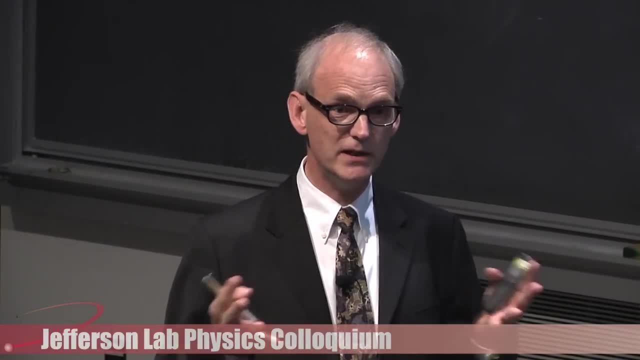 But one thing that I would like to mention is- and I'm a bit reluctant to use this word, but it's the word stovepiping- We have to break these barriers between the various science disciplines. At this moment in time it is very difficult for somebody- 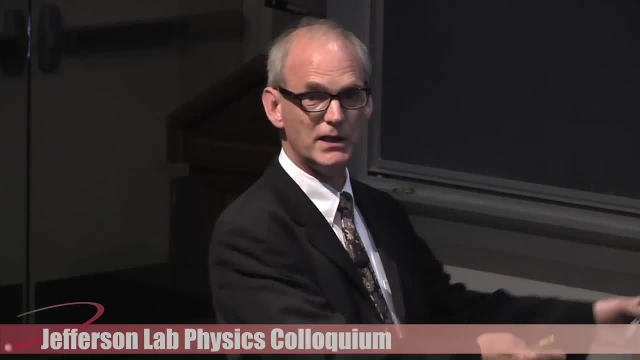 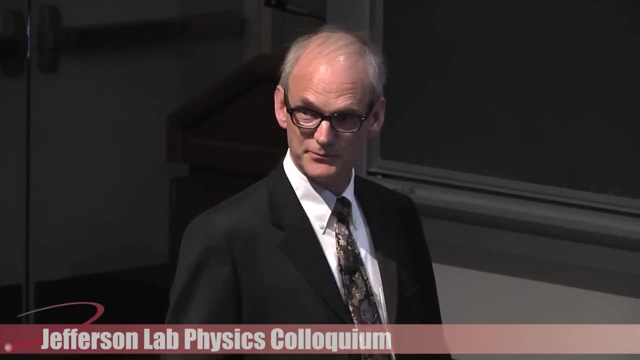 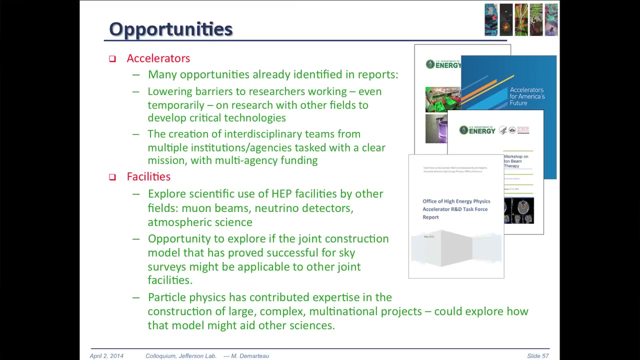 to work for a couple of months in a completely unrelated field unless you have a budget code, And often that is a limitation And that I think has to change. And similarly for facilities, I think we should explore really if joint construction of facilities, 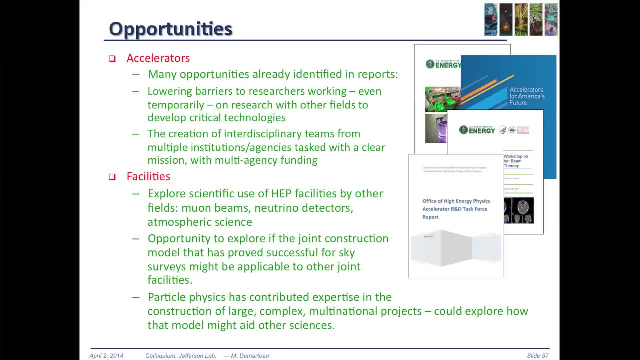 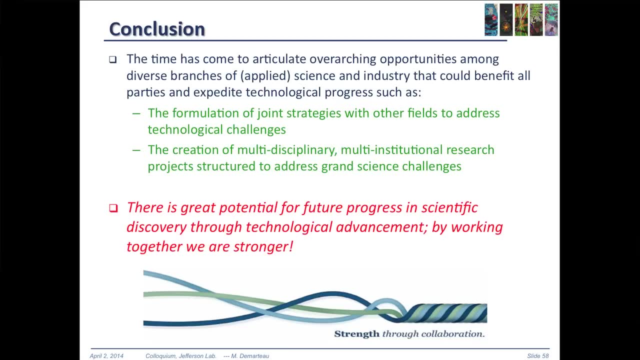 that we have demonstrated already that they are very good and can cater to a very broad community, how we can expand them. So, in conclusion, and I would like to say that the time has come really to really to articulate, you know in a better way. 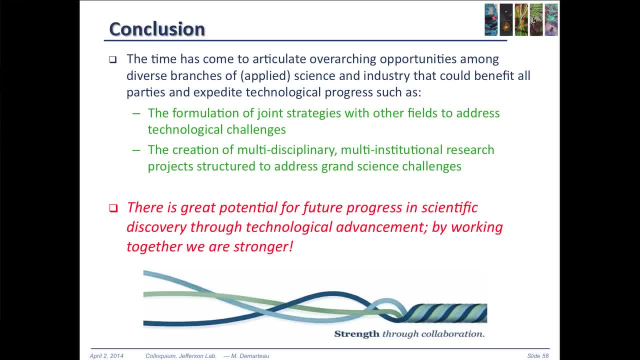 these overarching opportunities for us to work together, And I think you know two ways. that I would like to see is really the formulation of joint strategies to address technological challenges, But joint strategies beyond one scientific discipline, So really the creation of these multidisciplinary 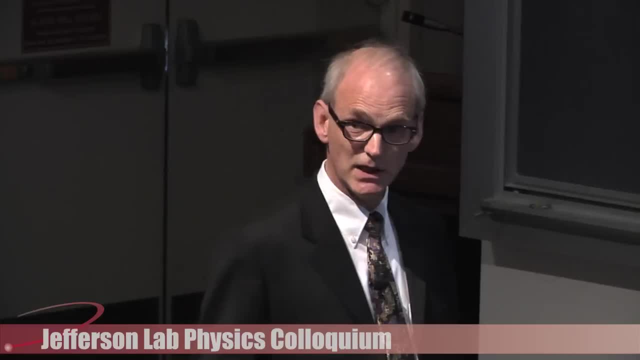 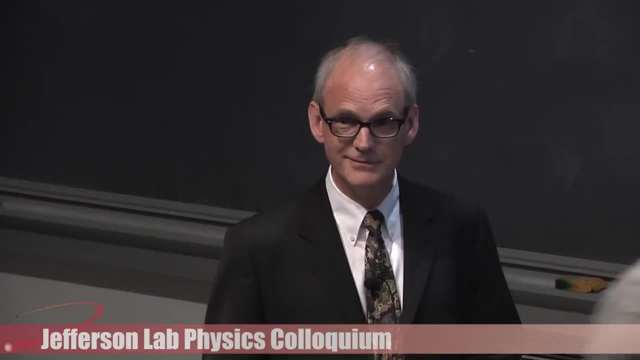 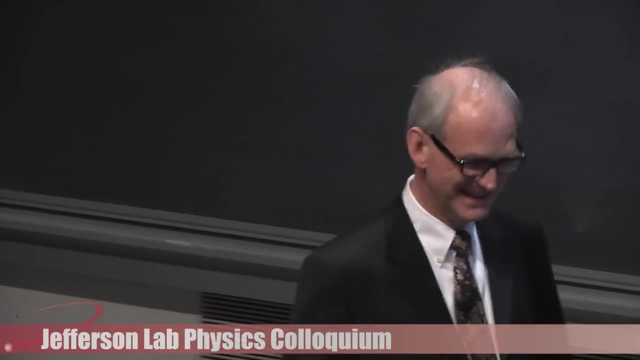 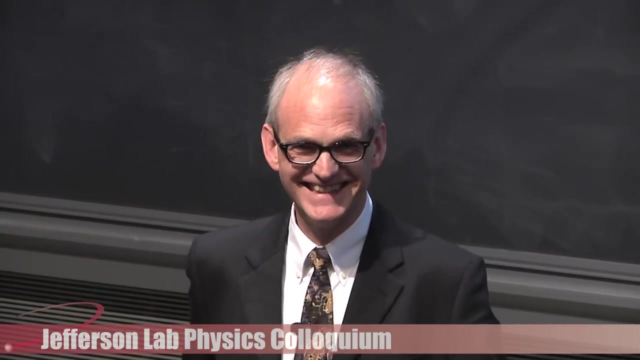 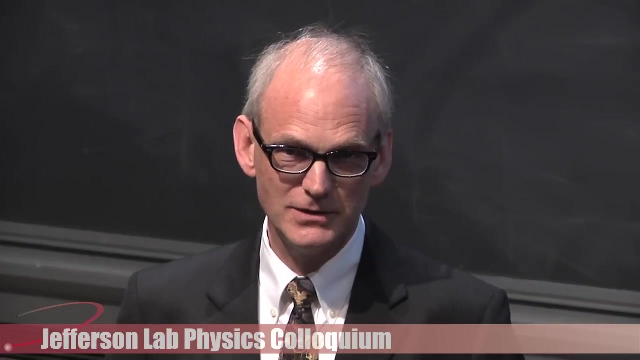 multi-institutional research programs And I think you know, together we are stronger. Thank you Questions. I can't help but ask this question, since I had my hip replaced last December. So how does the ion implantation help the titanium become more? 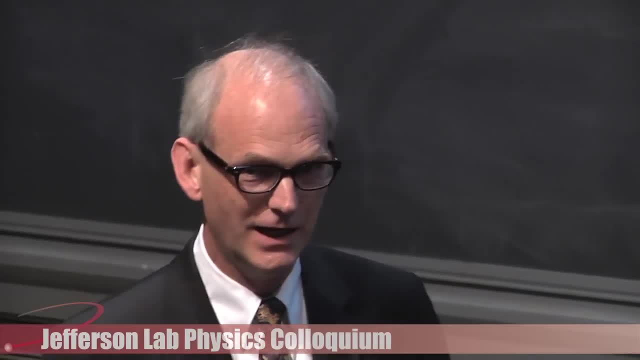 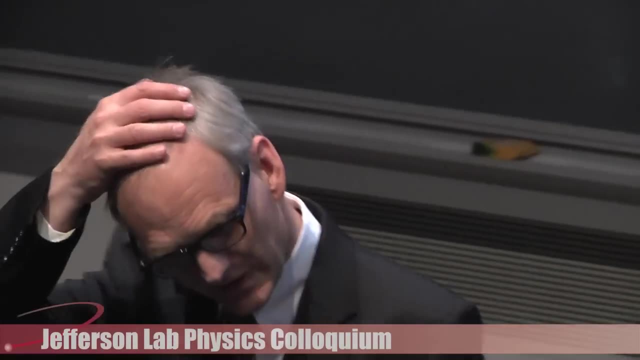 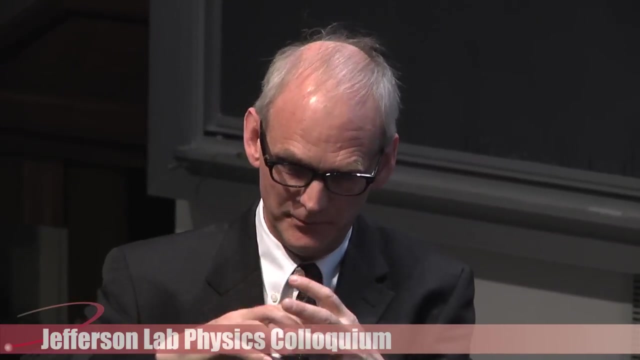 have a better affinity to bone structure? I'm afraid that I cannot answer that question, But there are two issues there as far as I understand. One is the wear, you know, of the titanium surface, And the other one is actually to 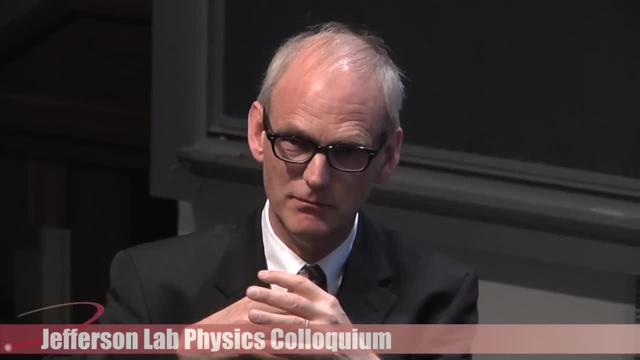 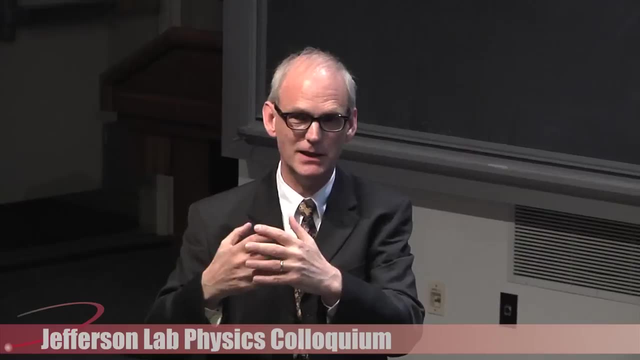 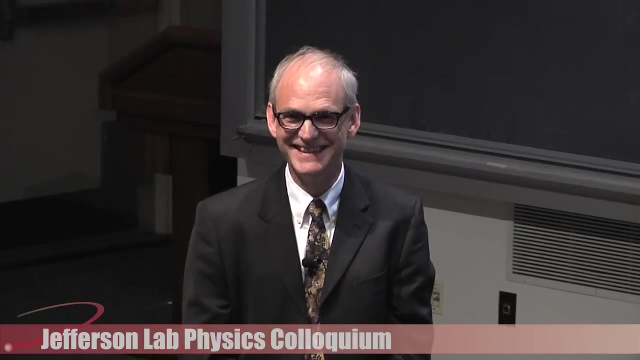 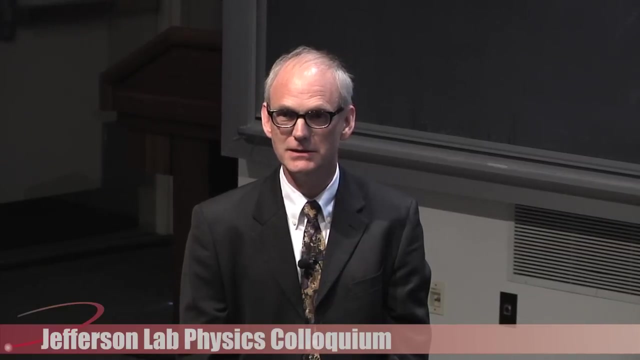 have less friction between the two surfaces. Why nitrogen, you know, in titanium gives you this result. I am sorry, I have to. I don't know the answer to that. Jim Boyce, Can you comment on the recent article from the New York Times? 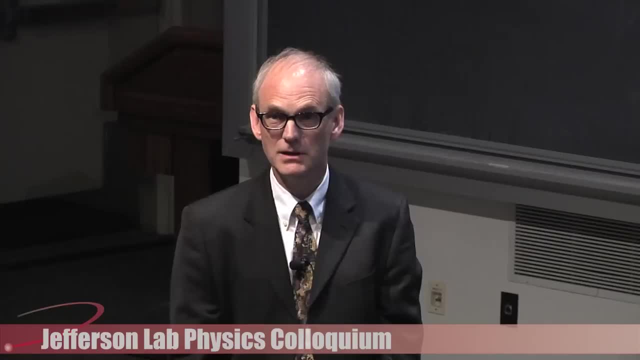 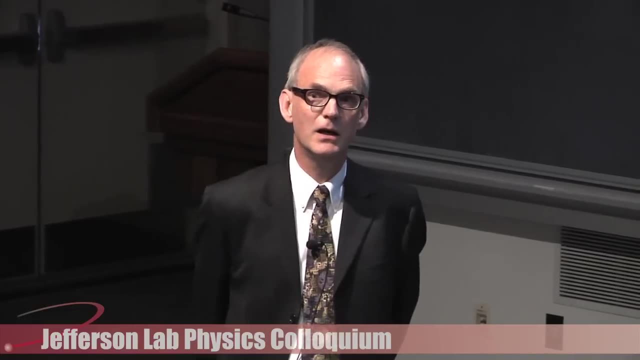 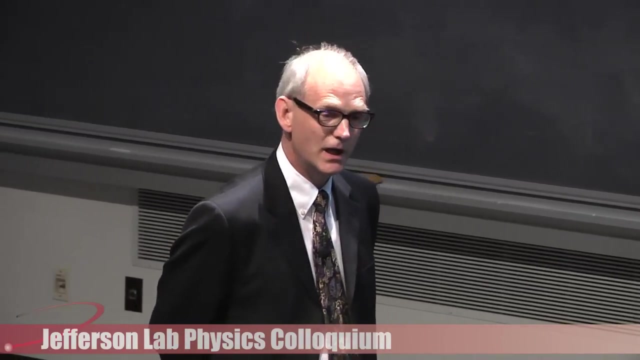 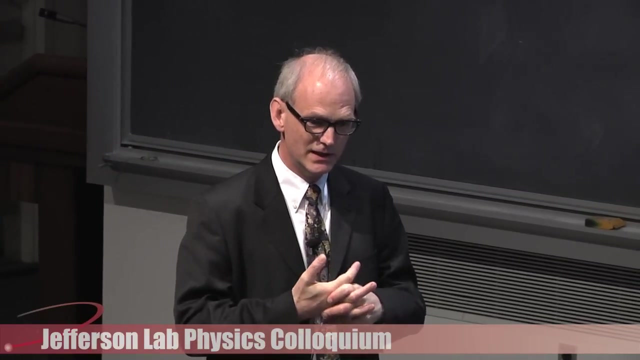 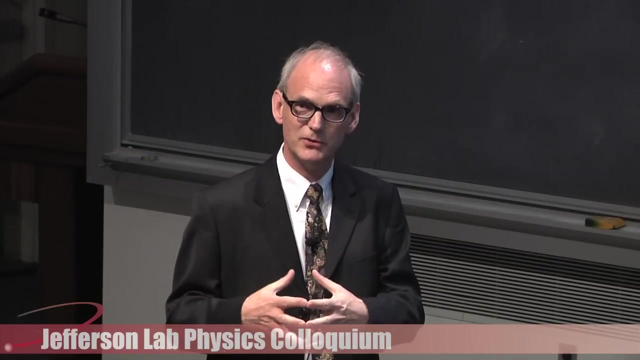 about private funding for research, the billionaires funding big research like this, and whether that is good or useful or not. That is a very interesting question. I personally believe you know there are two aspects again to this. You know, private industry fund research. 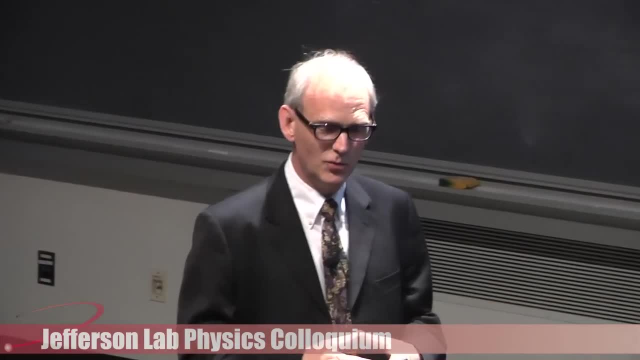 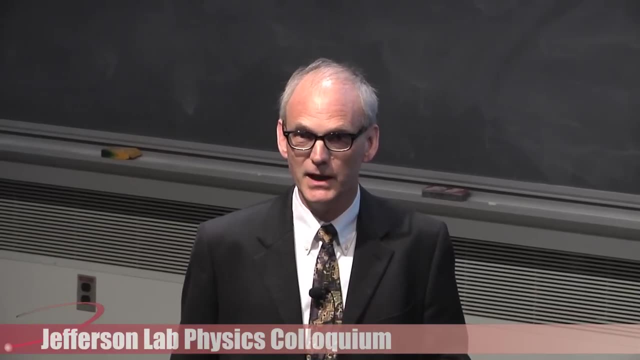 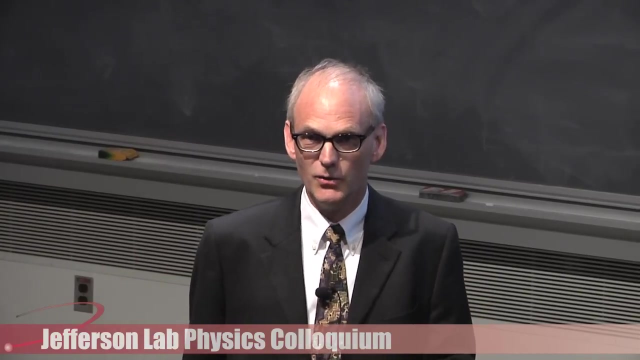 I think is a good thing. What I do not really like is, then, that you're beholden to, you know, the private donor. I really think that, and this is a question for us as a nation, you know, I really think that. 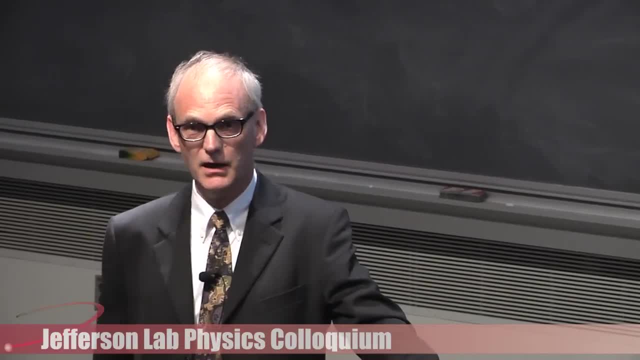 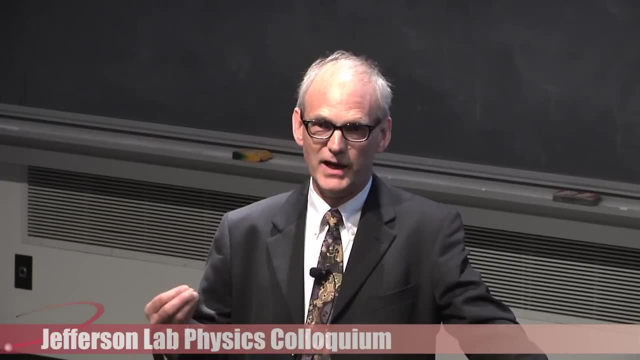 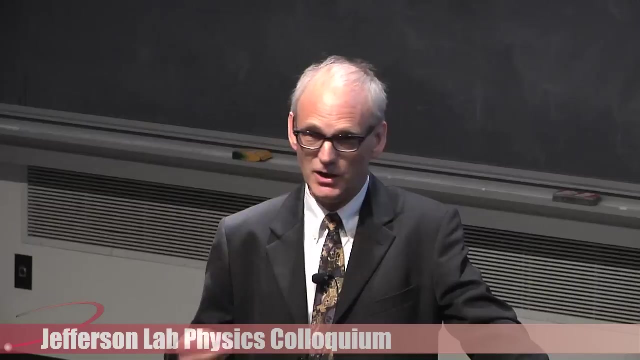 it is the responsibility of the government really to value, to decide how much value they want to put in the development of new technologies, in the development of new instrumentations, be it, you know, basic science or applied science In that sense. 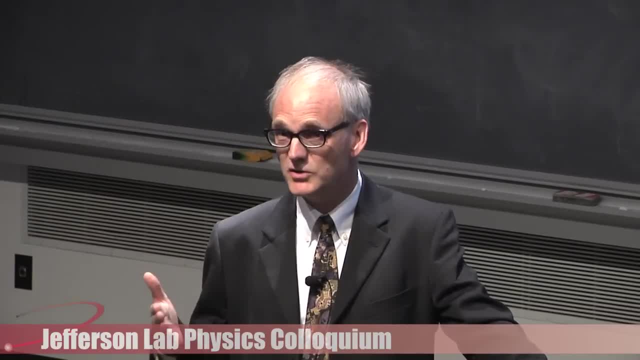 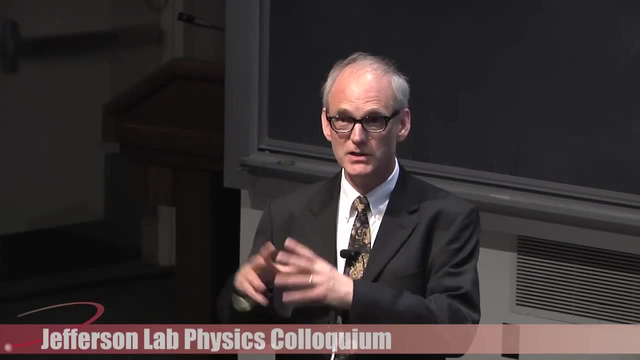 I think that the Europeans are doing a much better job at that. If you look at, you know, in Germany, for example, you have these Fraunhofer Institutes. These Fraunhofer Institutes get a chunk of their money from the government. 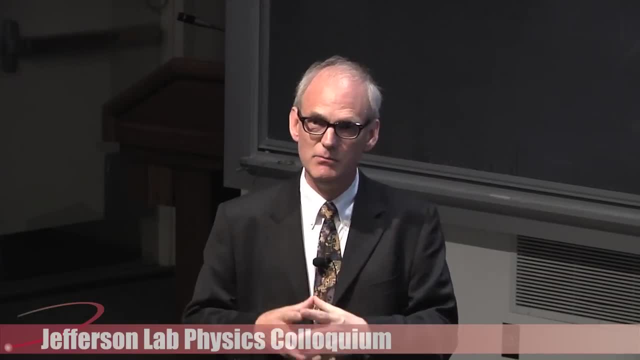 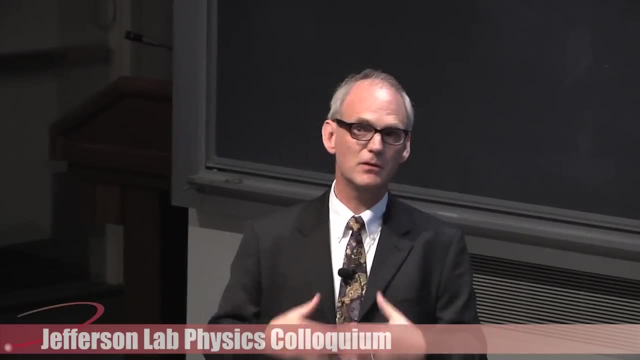 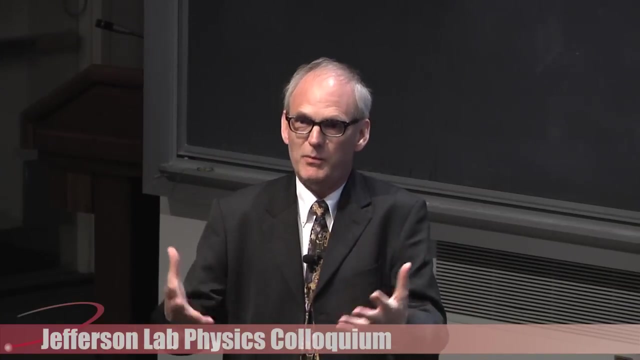 And what they then do is they team with industries and they team with universities to come up with new ideas. you know new technologies that advance. you know whatever problem they are addressing, be it, you know again, applied science or fundamental science. 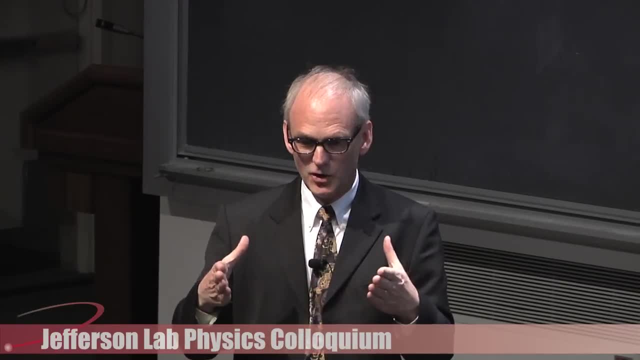 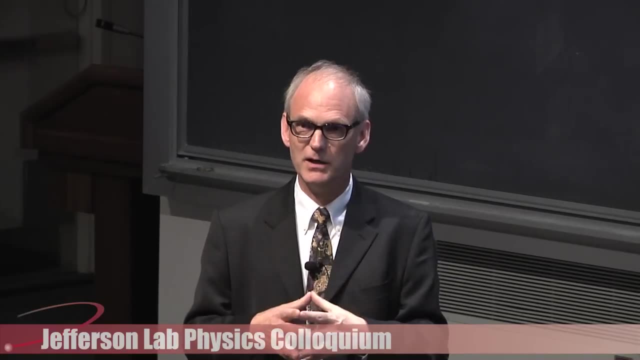 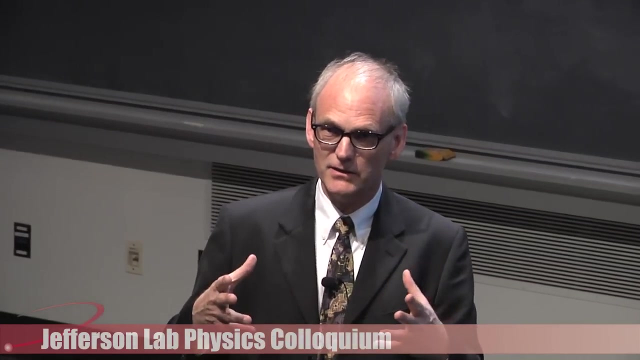 are very pragmatic And you know, I think that here in the US we are really desperately lacking some kind of initiative like that. The other thing that I want to mention- is sorry- is if you look at the European community. 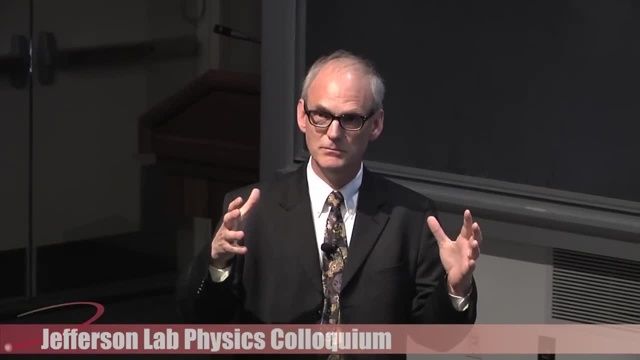 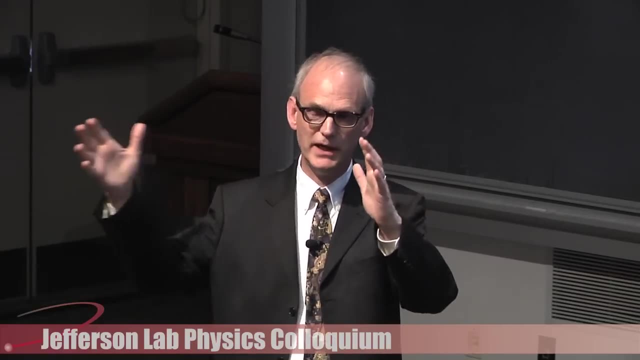 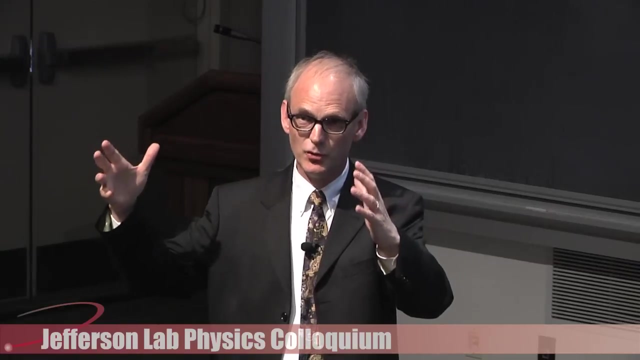 they have these four to five year. you know, frameworks, you know, and the new, the next one for the next five years, is called Horizon 2020.. And that is that is run by the European Commission, where Europe decides, you know. 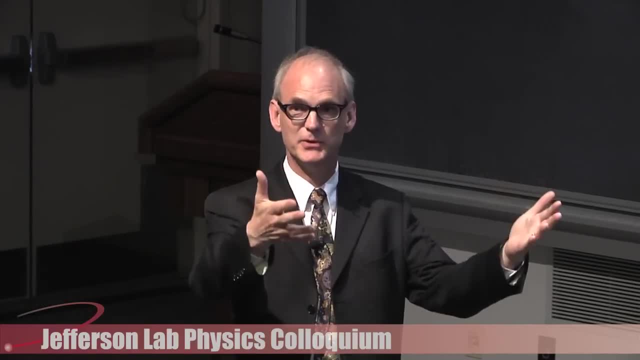 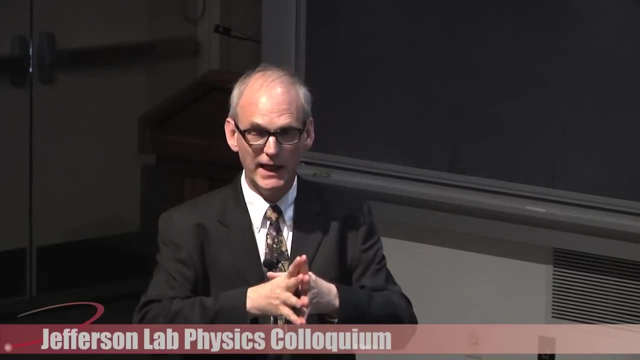 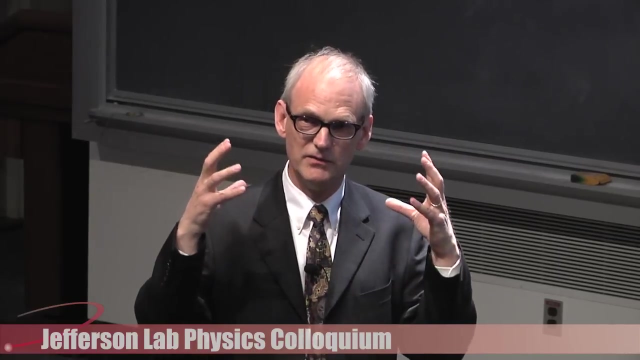 what the emphasis should be in terms of investments in, you know, basic research And, in this particular case, very applied research. And they are putting- you can look it up, you can Google it- they are putting $200 billion in as an investment. 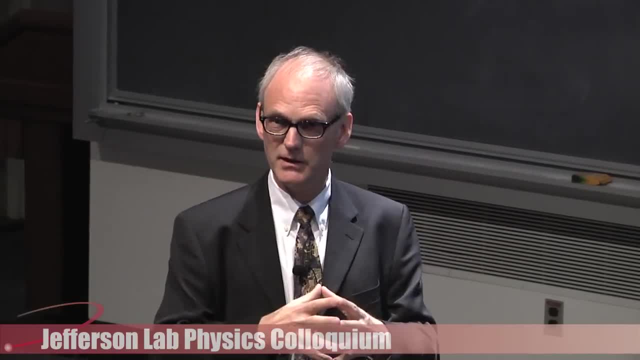 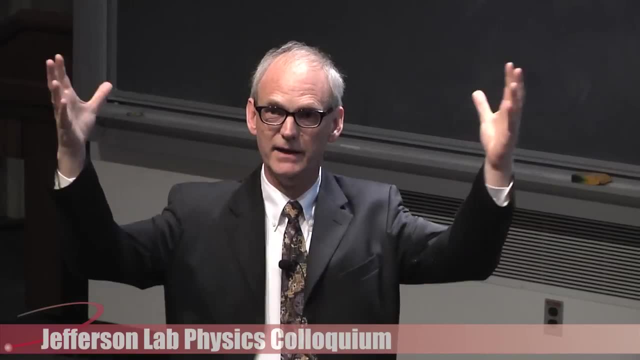 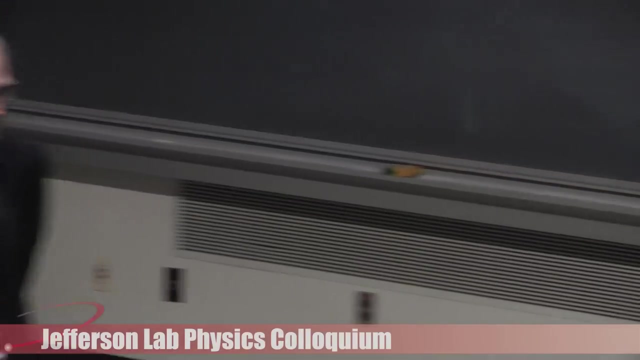 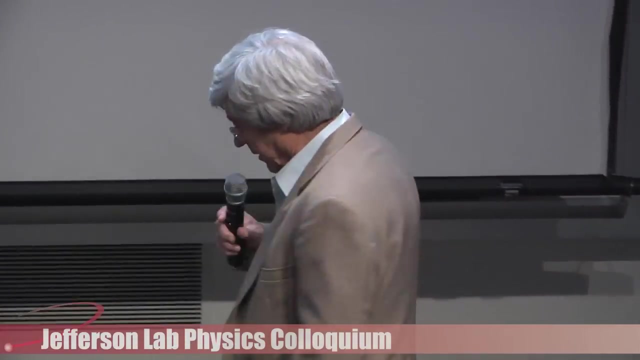 as Europe, as an investment in the development of infrastructure that will really move Europe ahead. So can I push back a little bit there? So I was on a review in Saclay in January and one of the complaints from the scientists in IFU. 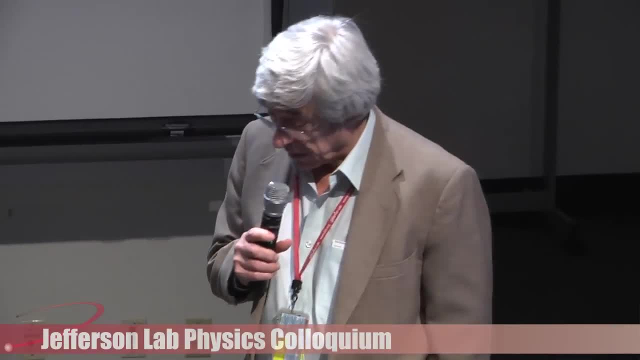 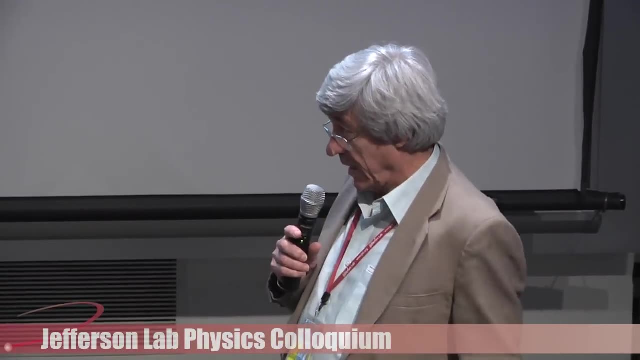 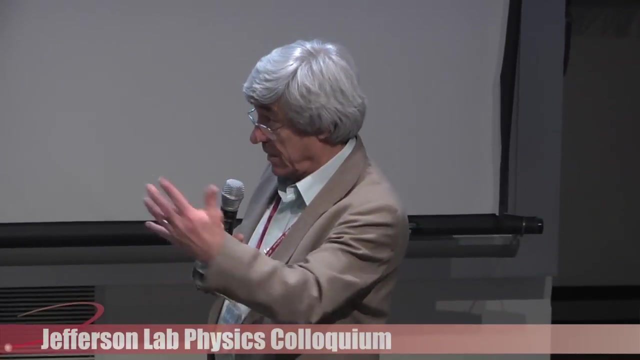 was that they, as a result of the initiatives everywhere and the inhomogeneity of the funding scenarios, that they were spending a very significant part of their time writing grants, grant proposals, And they missed the, if you like, the monolithic. 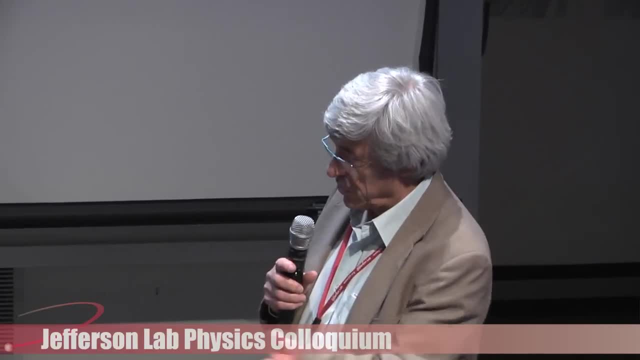 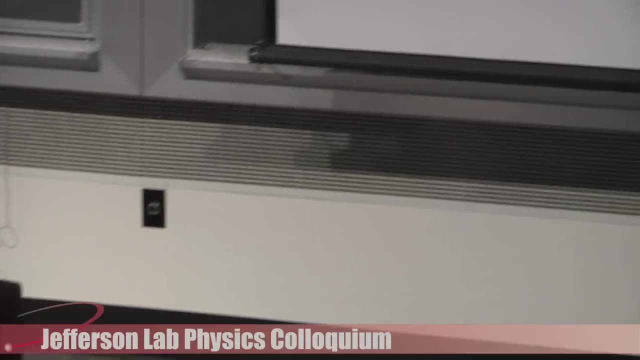 funding of a laboratory in which then the director shared it out without any administration. if you wish, Fully fully agree with you. You know, even though I mentioned the number- $200 billion- what actually trickles down to the various institutions is very small. 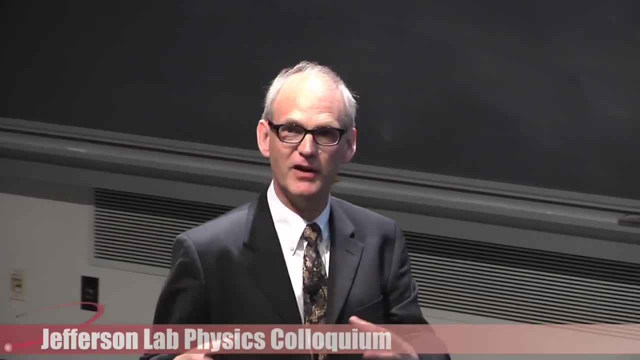 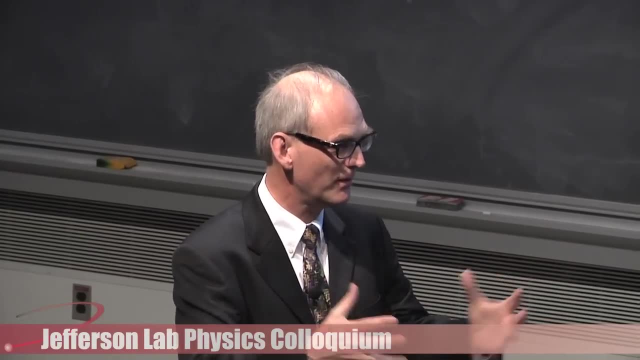 I mean, CERN is looking at you know something like $25 million, 25 million euros that they want to get out of that, and the overhead in writing grant proposals being reviewed is is bordering, you know. 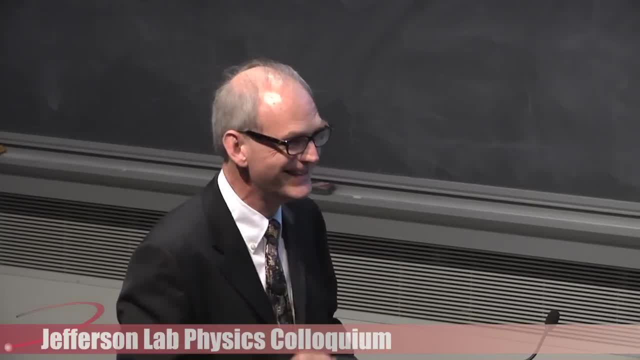 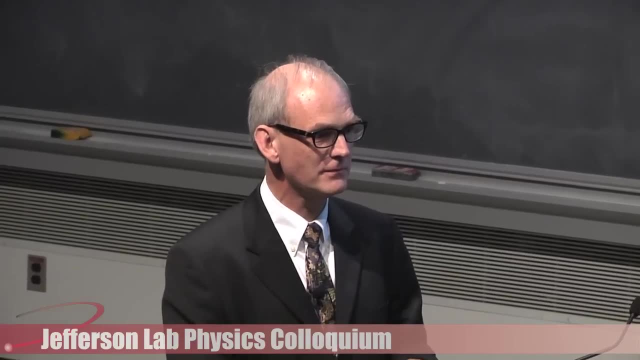 being ridiculous. I agree with you. And the other thing I would say in support, I mean with respect to Jim's point, I mean you. I would argue that that you know the the IBM Watson Center and 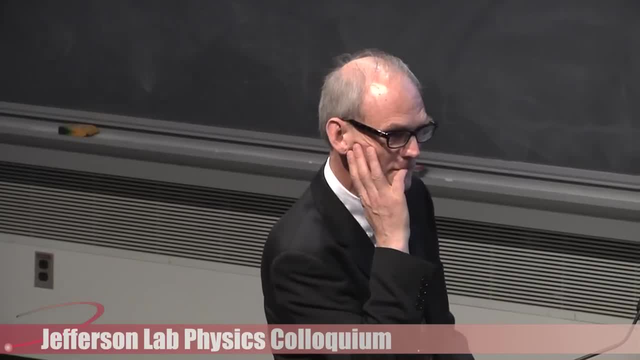 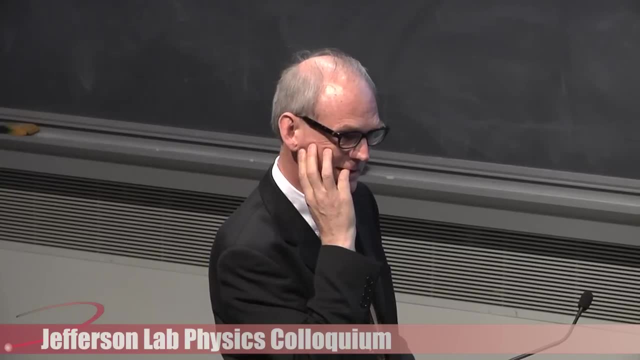 and other. you know the. these were, if you like, private investments right And and they were a major driving force of of US science for for many years. I mean, you wouldn't have the cosmic. 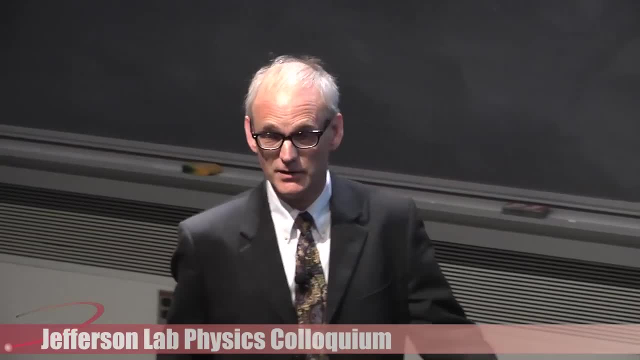 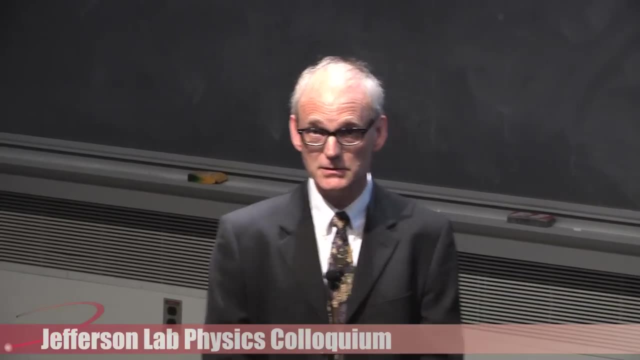 microwave background to talk about. without that, I mean, I I think it's a balance, I think you cannot, you should not just rely on, on private funding. You, you, you talked about miniaturization of electronics and radiation hardening of electronics. and you didn't mention NASA, And I would, in my mind, have felt that NASA would have been one of the leading agencies working on those two issues. Comments: To the best of my knowledge, the radiation requirements of of integrated electronics at the LHC. 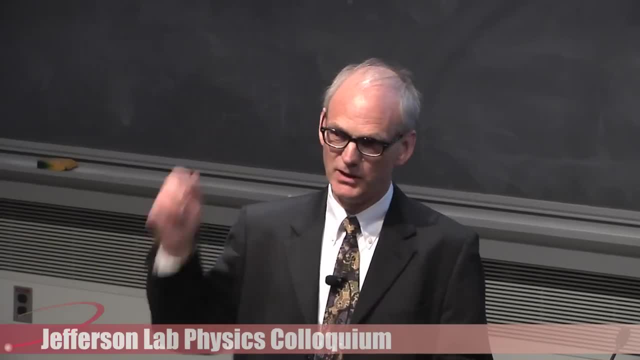 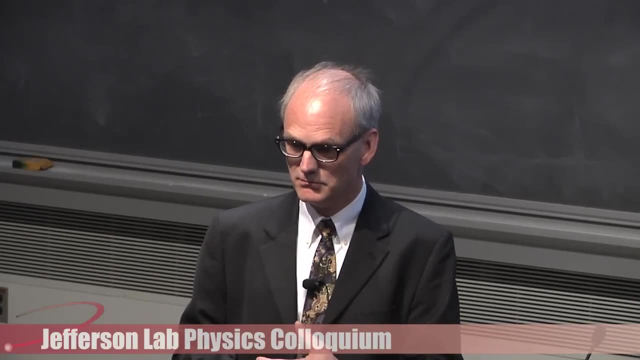 are much more stringent. So so the enclosed structures that were developed, you know, by by semiconductor industry, but with a large, you know, feedback and large input from the particle physics community, really has benefited NASA. Where did the 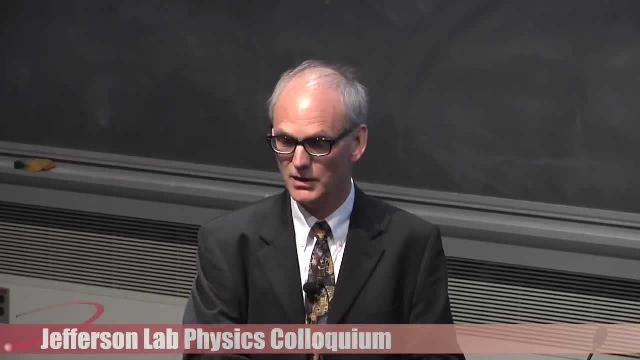 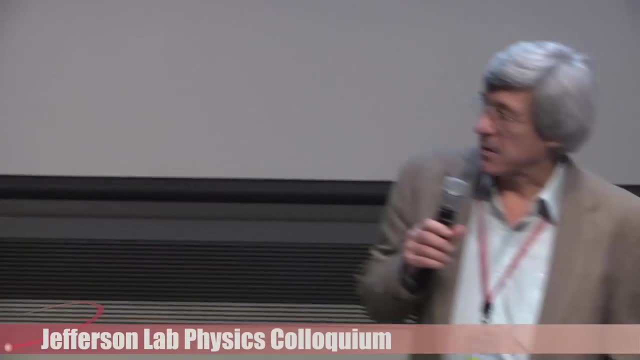 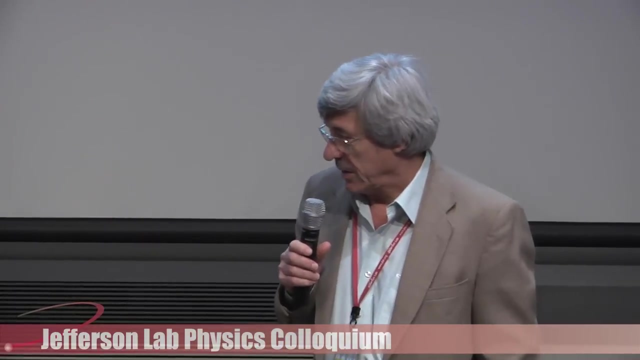 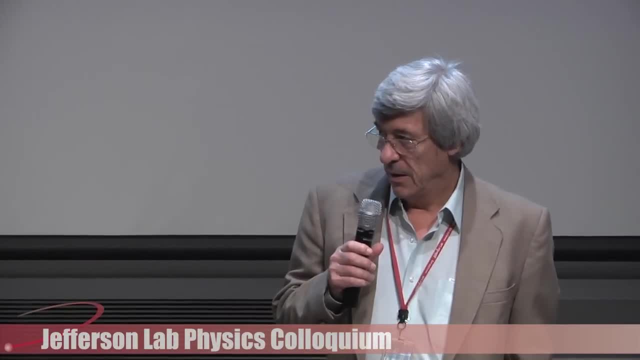 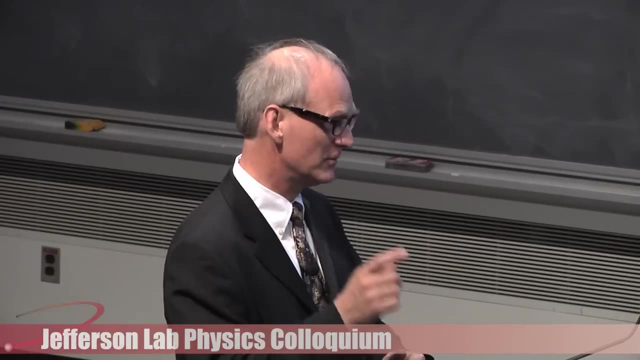 right? Yes, that that's correct. but you also know that that then, Jeff Hall, really so D-MIL was was, was was abandoned, Yeah, so we went to quarter micron technology, you know, and there 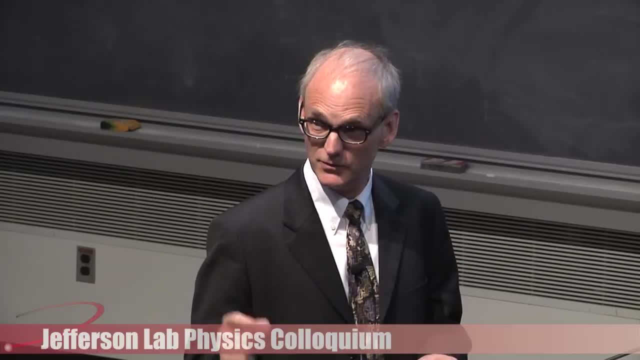 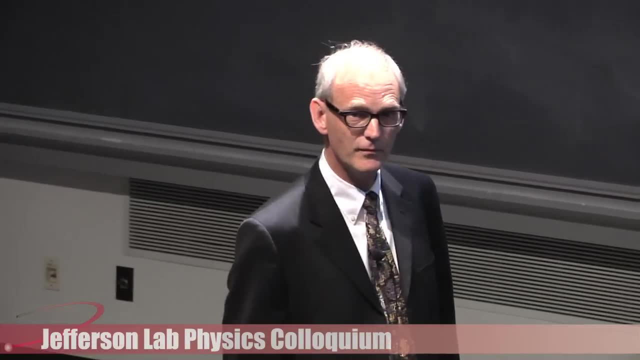 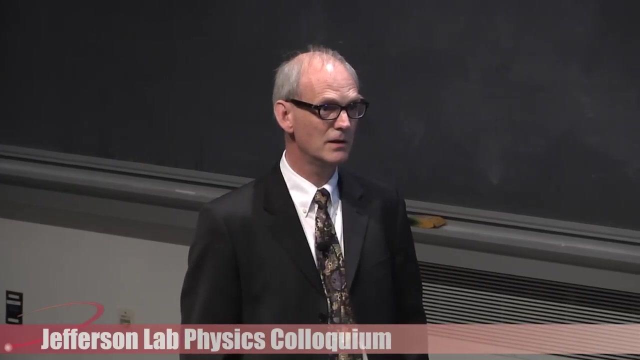 the, the, the. the designs were modified and adapted to really make sure that quarter micron technology was radiation hard and was abandoned. Yeah, So you mentioned the Alice Giga channel tracker. Just wondering what, what would be the cost for that? 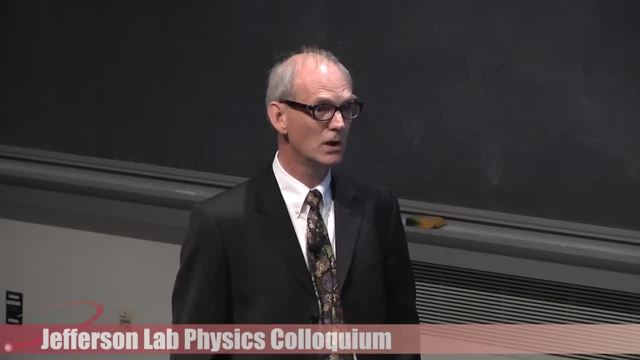 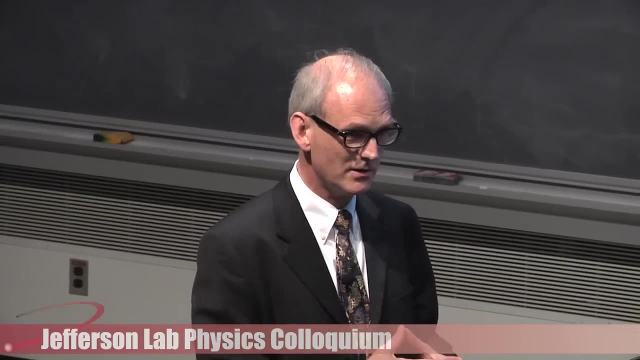 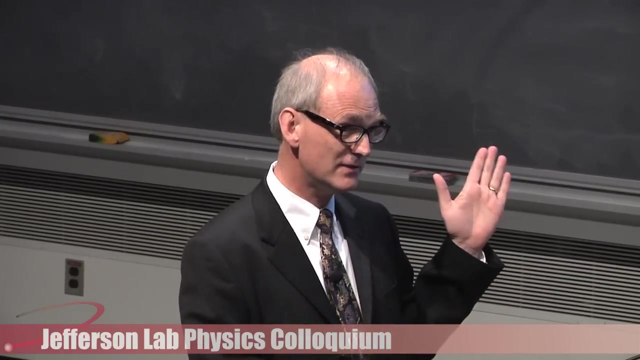 The Europe only gives you core cost, and the core cost, which is just, you know, materials for the Alice tracker is abandoned and the cost for the Alice tracker is, is, is, is, if I'm not mistaken, about 15 million.